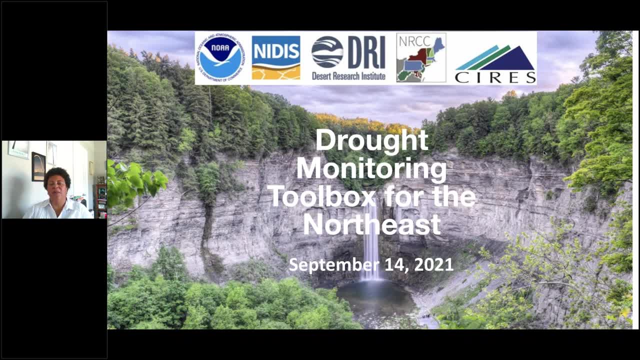 is the second of two webinars highlighting one of our many research projects and focusing on improving our drought early warning capability. So thanks for joining us. We'll get started with our presentation shortly, but I'd like to make sure that everyone is aware that in today's webinar, we will be following some slightly different rules than 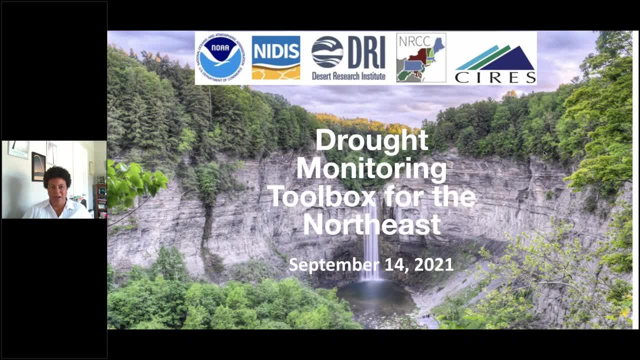 we did last week with regard to questions and the chat box. You should also know this webinar will be recorded and it will be made available within a few weeks, either through an email notification or you can always go to droughtgov, the drought information portal. 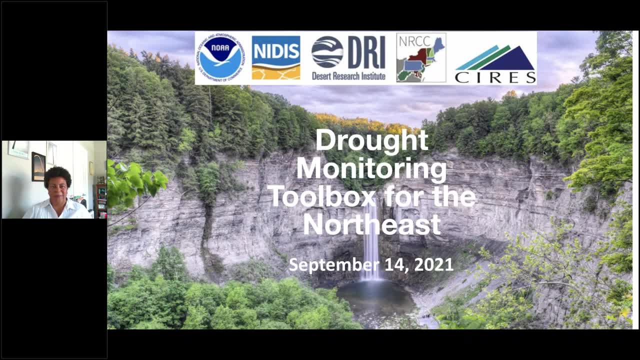 to find that recording. after we're done today, Adam is going to be monitoring the chat box with me and we want to make sure you check it frequently for any links to additional information. Also, you can put your questions or statements in the question section of the. 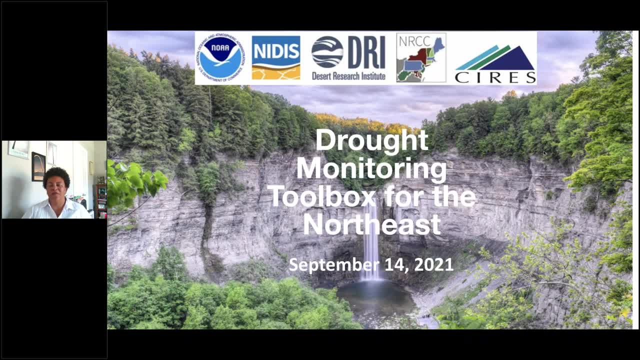 toolkit, which is on your right, for communicating back and forth for this webinar. So again, put your questions and thoughts into the questions panel and monitor the information coming from us in the chat box. So now that we've gotten our guidance for questions and chat straightened out for today, 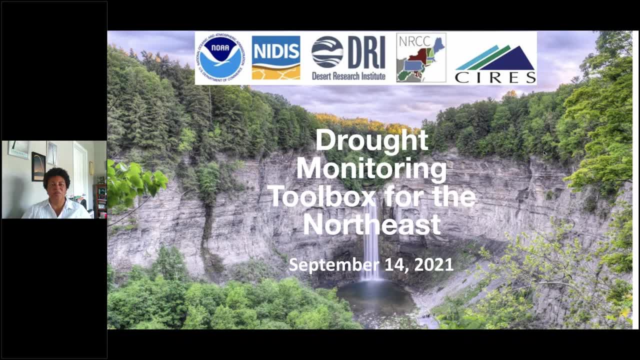 I'd like to introduce Dr Dan McEvoy, who is the regional climatologist at the Western Region Climate Center and the Desert Research Institute. He'll take a few moments to introduce his team, share an overview of the Coping with Drought project and he'll highlight 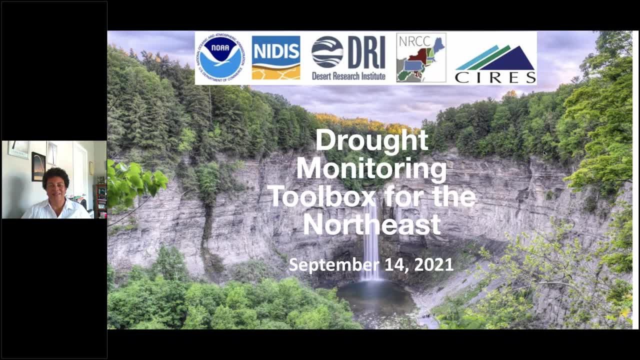 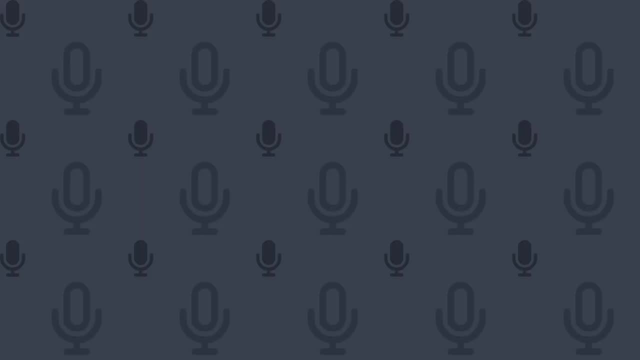 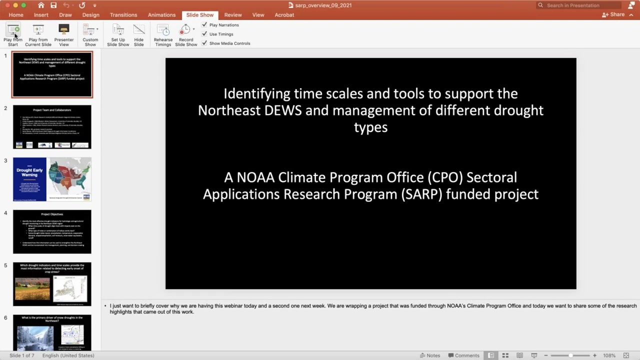 our agenda for today, Dan, all yours All right. Thanks so much, Delvia, for the introductions. I really appreciate that. Let me grab the screen back here, All righty? So before we get into the presentations on the tools today, I just want to briefly cover why we're having this webinar today, And I'll 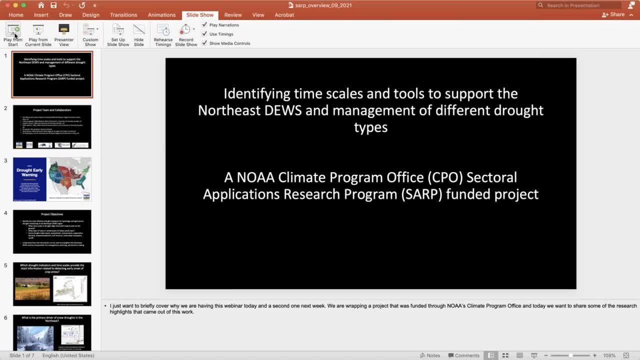 give you a little bit of a brief overview of what's going on today and why everyone's here, And so we're wrapping up a two-year project that was funded through NOAA's Climate Program Office, the CPO, And we wanted to share. first last week, we shared some of 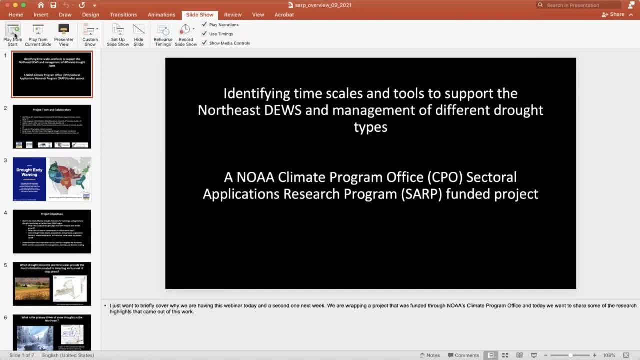 the research highlights. And then today we're going to focus more on how to access some of these drought indices, maps and data through some of the tools that the team has developed. Okay, So first I do want to introduce the team here, So I'm the PI, and then we had a group. 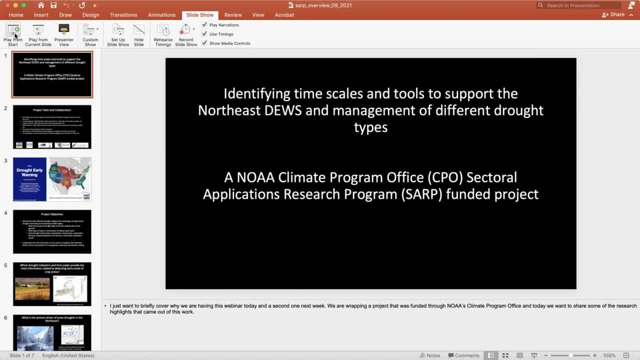 from CIRES and NOAA's Physical Science Lab in Boulder, Colorado. We had Imtiaz Ringwala, Heather Yochum and Mike Hobbins, as well as my graduate student Shuang Zai, who presented last week on the relationships between drought indices and crop health. And then we've also 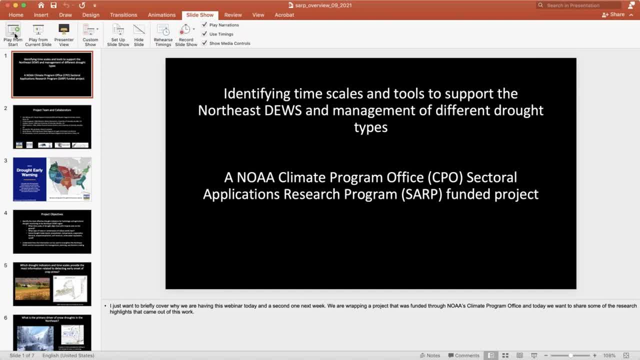 been working with Silvia and Art from the Northeast Regional Program. So we're going to talk a little bit more about the climate center and the Northeast DEWS. So this was a big collaborative effort. So Silvia briefly mentioned about NIDIS. I did want to mention a few more things about 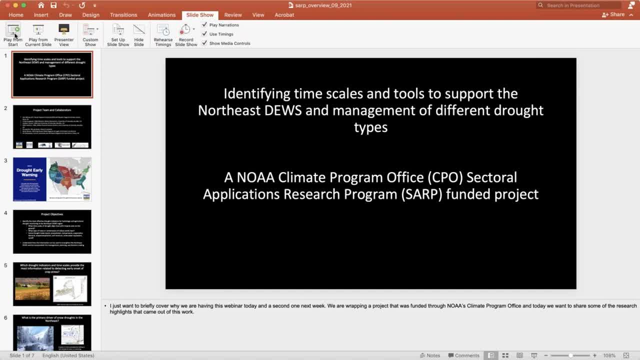 these DEWS, the Drought Early Warning Systems, And so this is a map of all of NIDIS's different DEWS regions. Hey, Dan, Yes, We are just seeing the slide deck with the slides on the side. We're not seeing it playing. 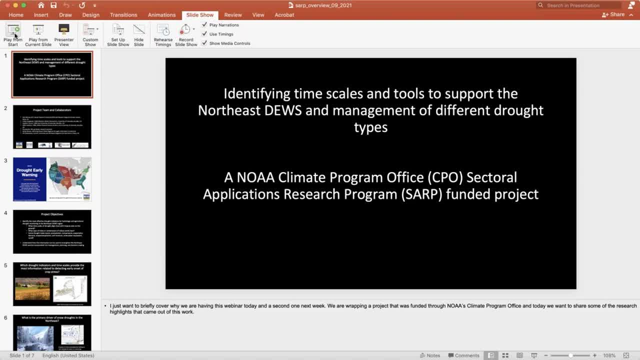 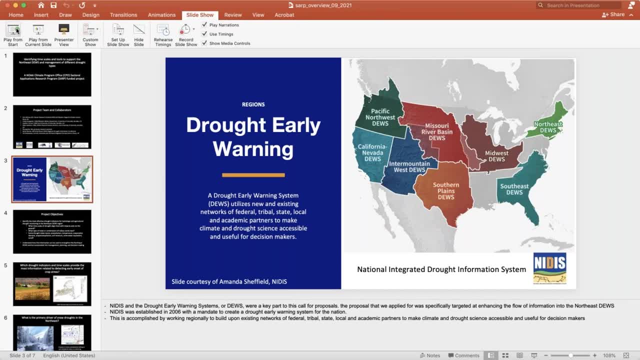 Okay, So this is a map of all of NIDIS's different DEWS regions. Okay, Thank you. Okay, Let's see here. How about now? No, we're seeing that slide now, but we're still seeing it on the side. Try play from. 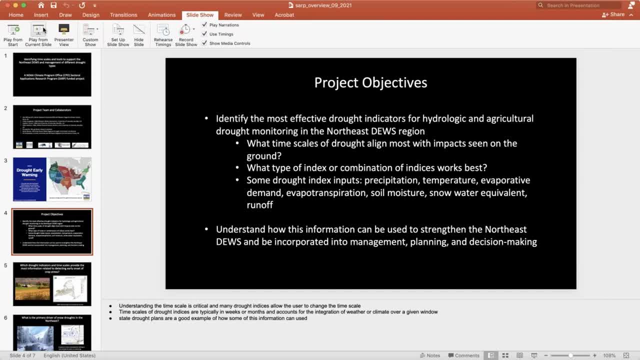 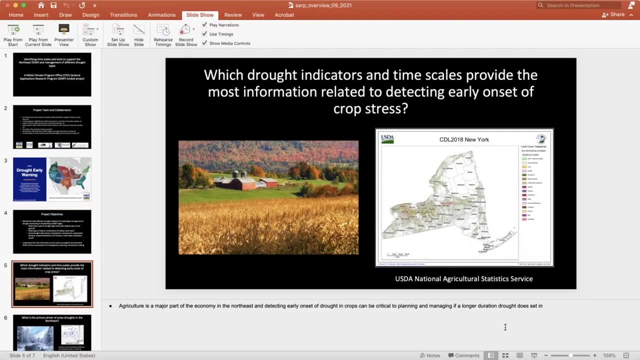 current slide, maybe Okay. Okay, Is that any better? Nope, Let me try a couple more things here. Sorry everyone. How about now? No, Maybe try closing it out again and opening it and see if that works. Yeah. 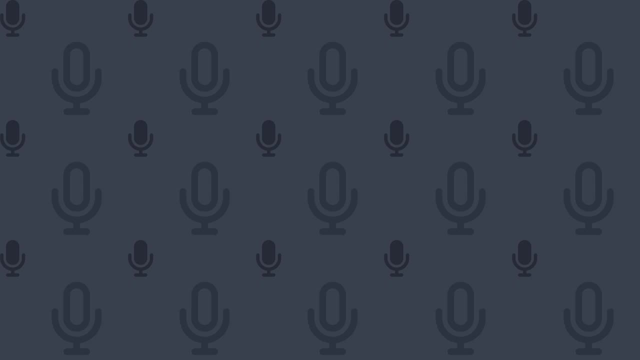 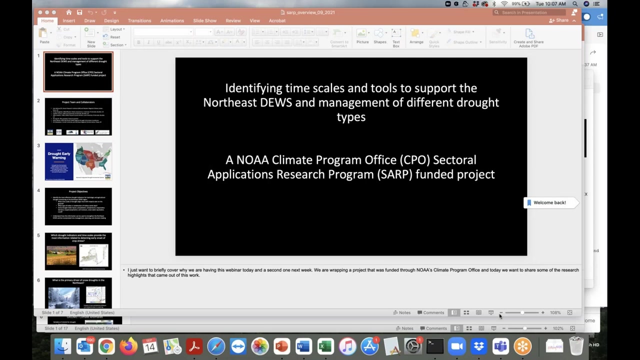 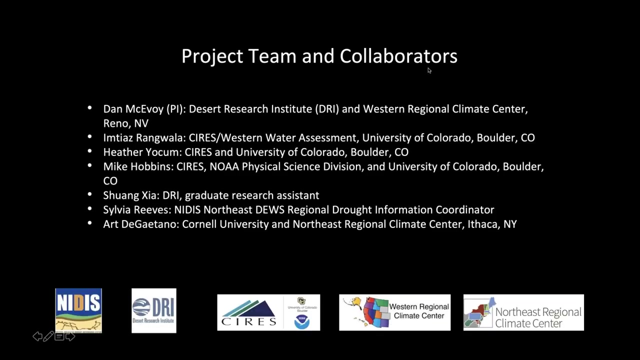 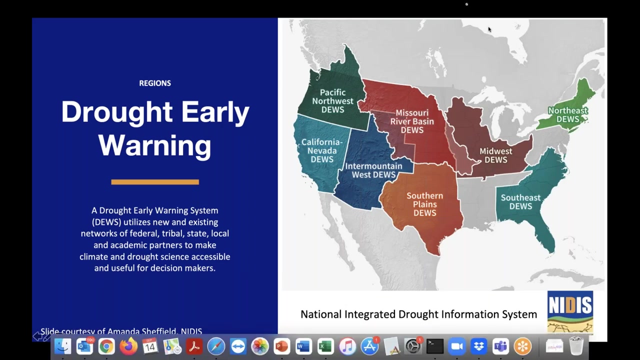 Okay, Let me see here, There we go. Okay, Let me just make sure you're seeing it. progress through Yep, Perfect. Okay, Apologies everyone, After all these months, or now years, of this, we're still having technical difficulties. 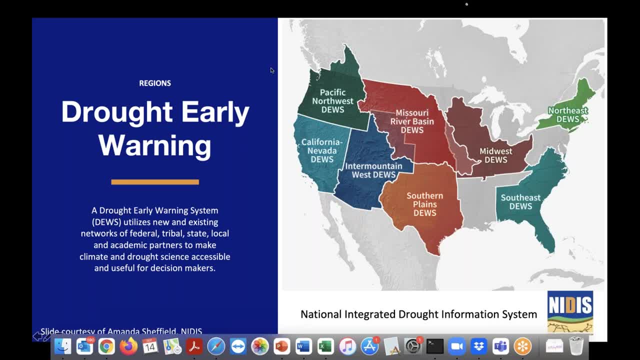 So let me get back into the drought early warning systems: NIDIS's drought early warning systems. So this map on the right has all the different regions and the Northeast region is one of the more recently established drought early warning systems. And this came about after. 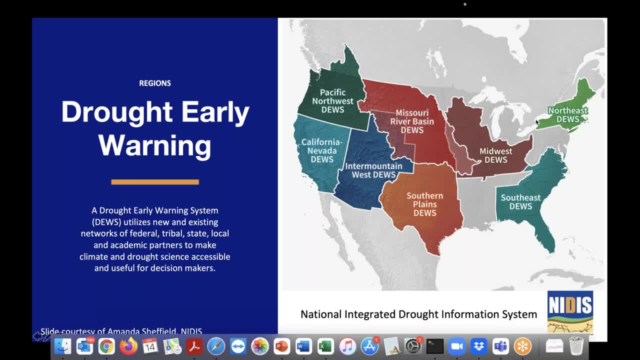 or during and after the 2016 drought, when there seemed to be a bit of urgency for better monitoring and understanding of drought. So this is a map of the drought early warning systems in the Northeast, And so that's where the Northeast DEWS came into play. 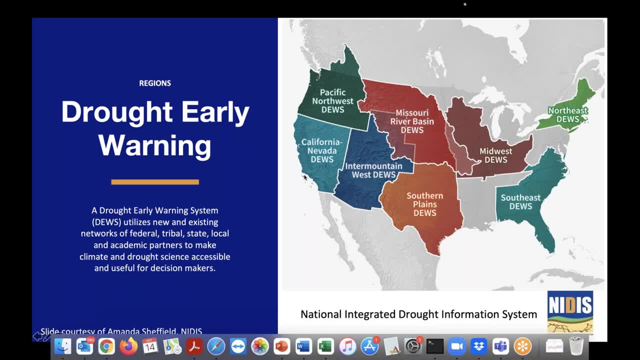 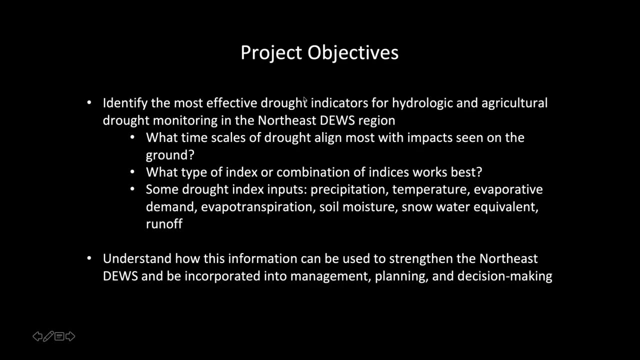 And the work that we've been doing is really to just help understand which drought indices and indicators and data sets really work best to help monitor these drought conditions in the Northeast. So we did have a few main objectives On the research end. it was to identify the most effective drought indicators for hydrologic 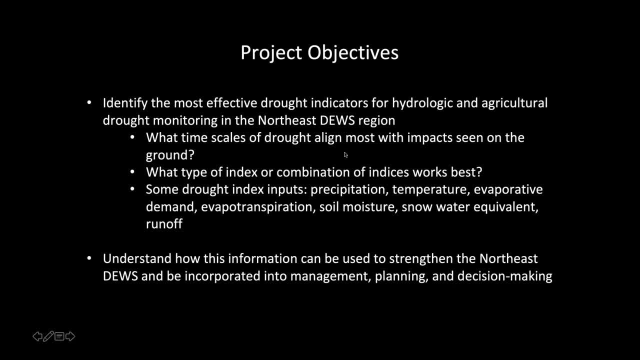 and agricultural drought monitoring in the Northeast, And this got into the different timescales of drought and how they relate to impacts, which indices or indicators, and that varied from atmospheric variables to land surface variables. And then the last bullet is talking about incorporating this into the Northeast DEWS. 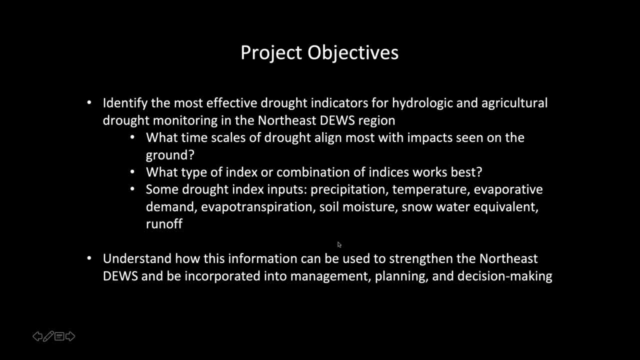 and the management and planning, And so a lot of that comes from being able to identify the most effective drought indicators for hydrologic and agricultural drought monitoring in the Northeast. And then the last bullet is talking about how to access the data and the visualizations. 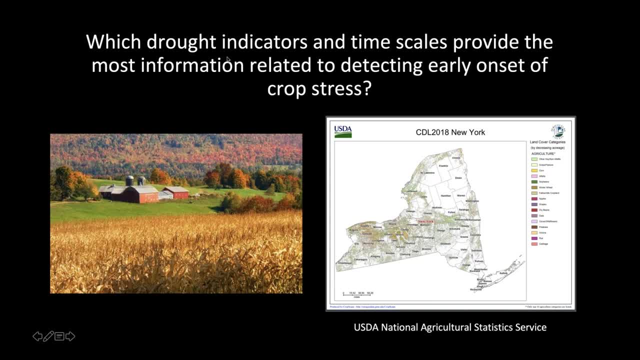 through different tools And, again, that's going to be the focus today. So last week we covered a couple of different research topics, one of them being the relationship between drought indices and crop stress. That was presented by Shuang Zai, who did a great job. 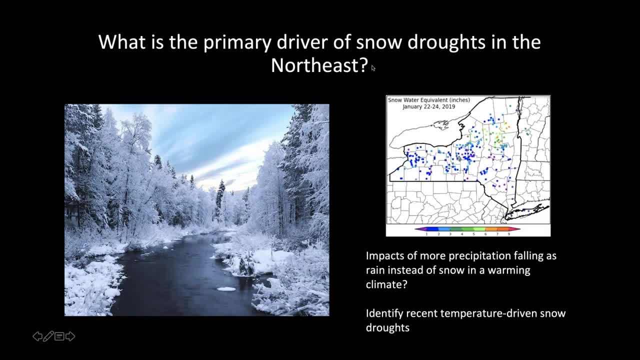 And he talked about a lot of different indices and showed a bunch of maps and time series, And so we're going to show you how to access some of that today, And then we're going to talk a little bit about some of the other topics that we covered. 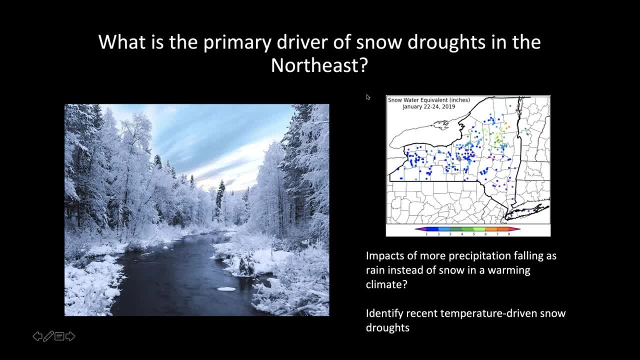 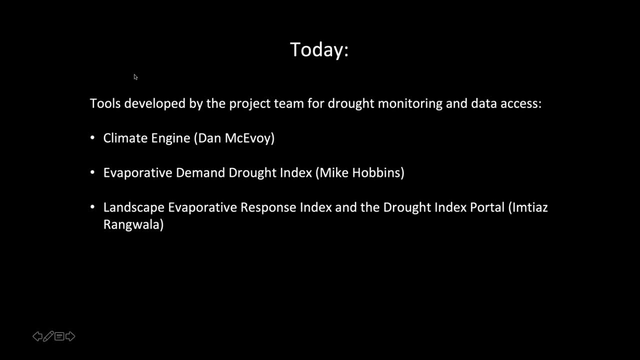 and learning about how temperature drives a lot of the snow droughts in the Northeast, And we also talked about flash droughts as well last week. But the focus is going to be shifted today from what we learned in the research to learning about some of the tools that have been developed by the team and how to access these tools. 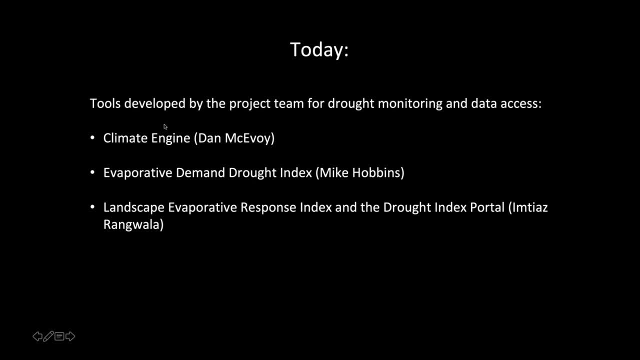 and the data that comes along with them. So I'm going to start off with a presentation on climate engine, And then we'll turn it over to Mike Hobbins for the Evaporative Demand Drought Index. And finally, Imtiaz Renwala will present on the Landscape Evaporative Response Index. 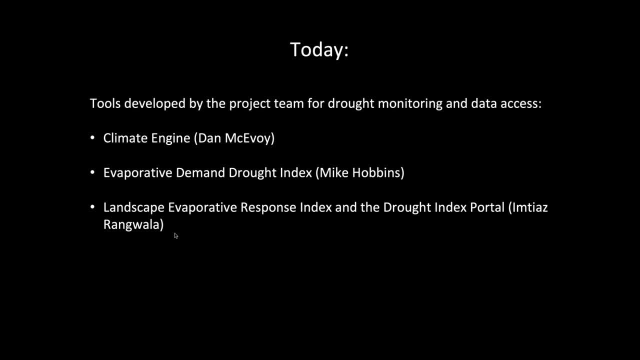 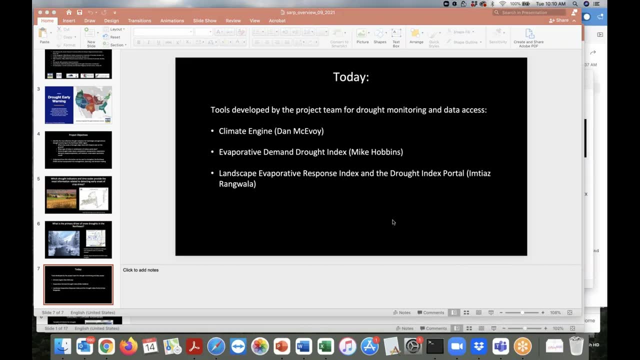 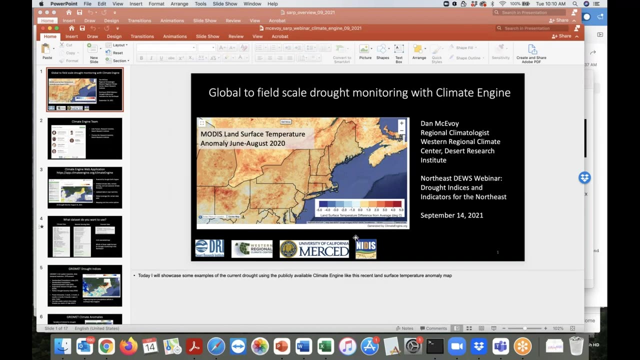 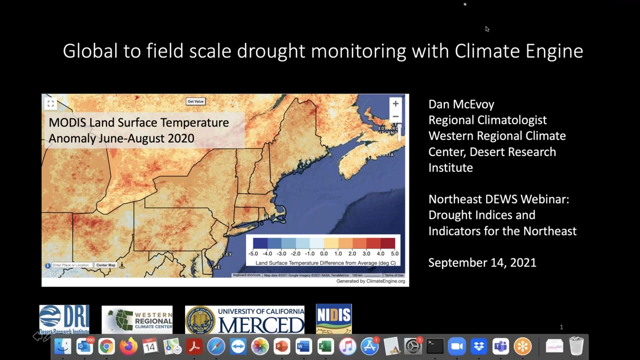 as well as the Drought Index Portal. So I am going to shift presentations now And hopefully this will work. Okay, Are you seeing the full screen mode? Adam Looks good. Okay, Great, All right, Yeah, So I'm going to start off with the climate engine presentation. 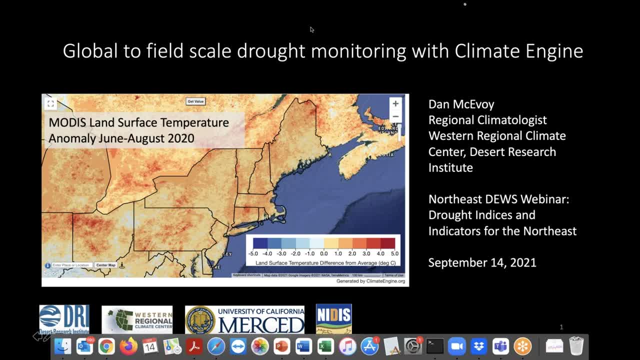 And this is doing a collaborative development between DRI and University of Merced, California, along with a lot of support from NIDIS, And this first map is showing one of the data sets that we can access from climate engine, Which is MODIS's land surface temperature. 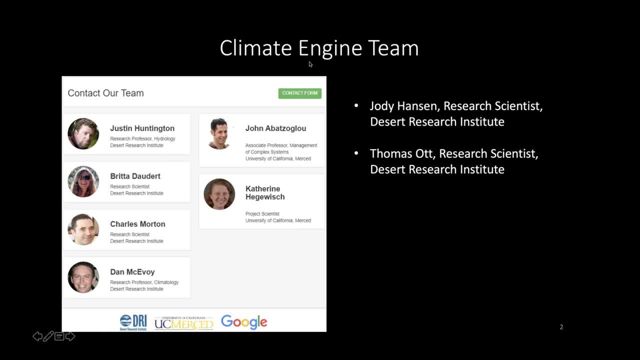 And I'll discuss more about that. So before I go any further, I do again want to acknowledge the climate engine team. This is my role in climate engine has been very minor compared to most of the folks shown here. Justin Huntington is the PI of this project. 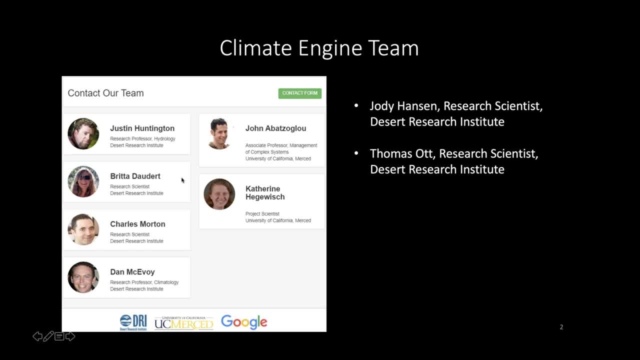 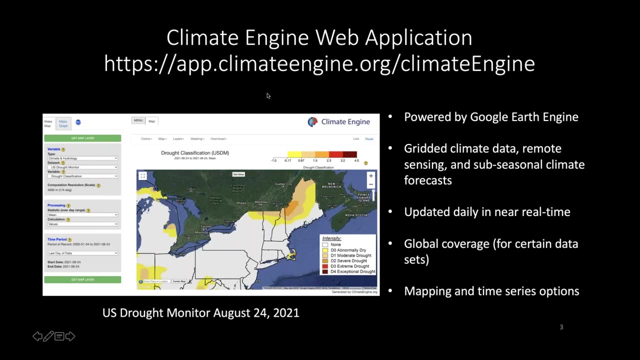 He's a hydrologist from DRI- But the developers, the software developers- there's a whole team, Five of them here that have really done the heavy lifting on developing this tool. So let's get right into it and talk about the climate engine web application. 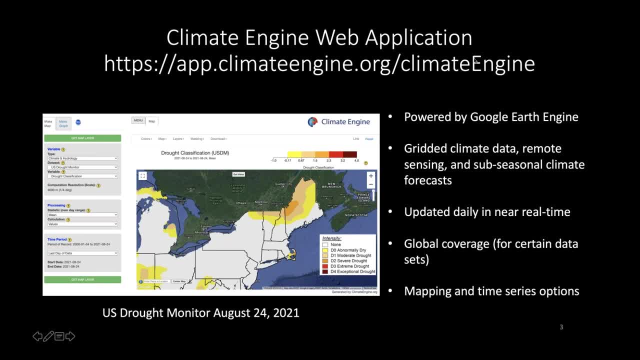 The main website is here, And I think Sylvia, if she didn't, will be putting this link into the chat as well. And so what climate engine is? it's a point and click web application And it's powered by Google Earth Engine. 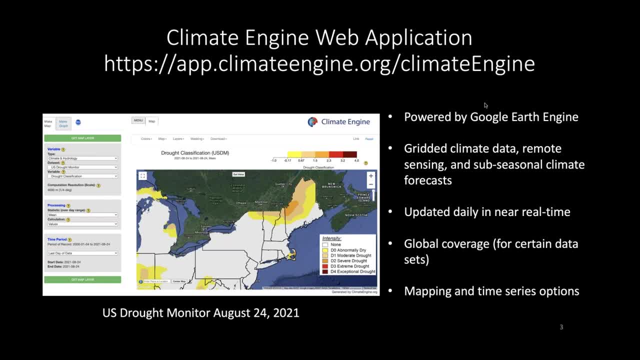 And so this uses Google's cloud, And I think most people are familiar with some type of cloud application, Whether that's Google Drive, Dropbox, Amazon Web Service. These are all cloud-based data storage where you don't have to store any of your data locally. 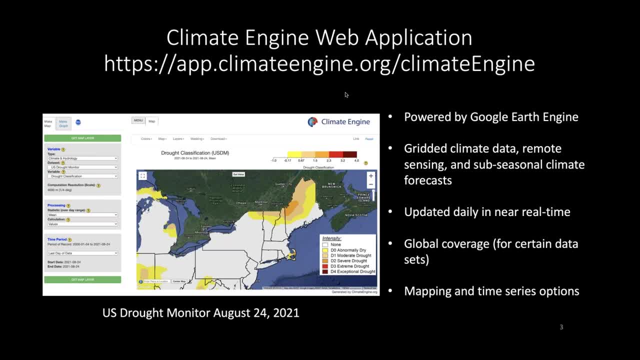 And it all lives on these data farms in various different places. So you can access that information without the data being stored locally. And this screenshot here is the main web interface, The mapping interface, And so climate engine hosts various gridded climate data remote sensing. 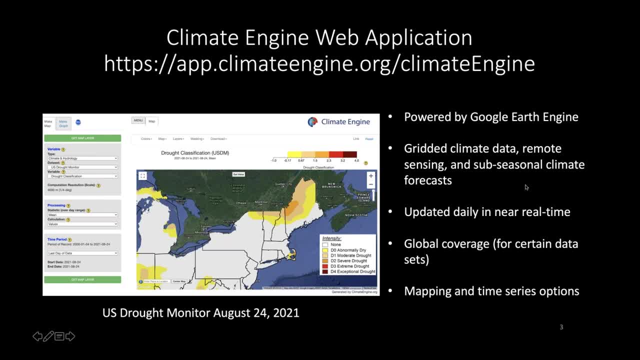 And recently we've added some sub-seasonal climate forecasts as well. Most of the data sets are updated daily or in real time, Whatever the time stamp of the data is- whether that's daily, monthly, Something like the US Drought Monitor, that's weekly. 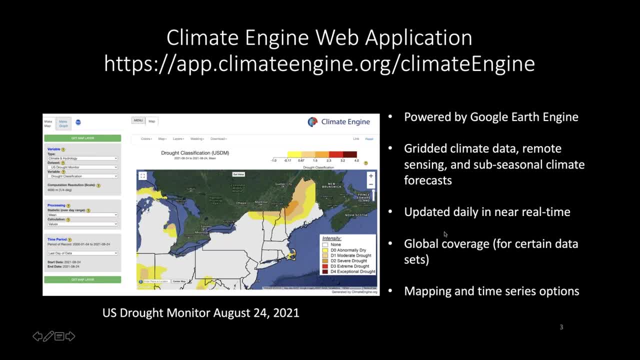 And a lot of these data sets are global, And so we also have the two main features are mapping Or time series options, And I am showing the US Drought Monitor map here from August 24th, And so this was a data set that was recently added into climate engine that you can access. 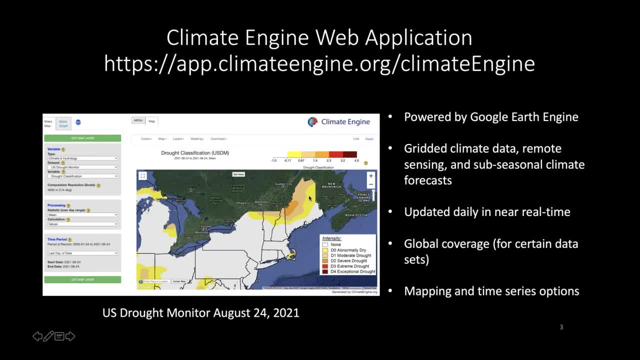 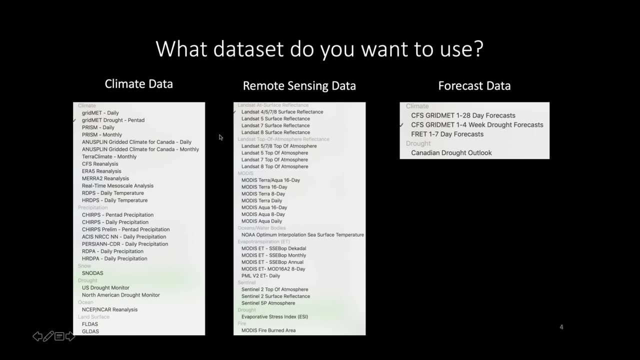 And so this is a Google Earth type of interface where you can pan and zoom in and out. There's a transparency bar where you can see what's the underlying map as well. So what data sets should you use in climate engine? So when you get in there, you'll have 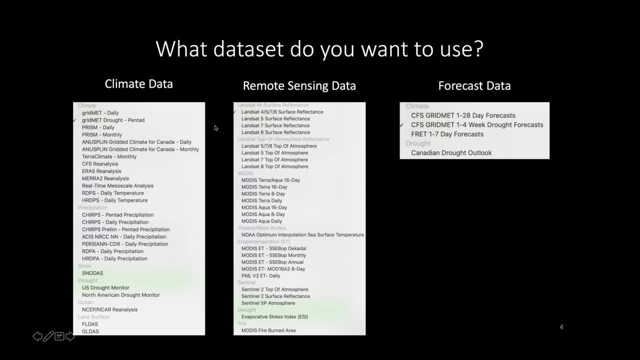 On the left. there you'll see all these drop downs, And so we have climate data. There's a big list here with different climate variables. Then we have some precipitation focused data sets: Snow based drought, monitor land surface models. Then the other main option is remote sensing, which is primarily the Landsat and MODIS archives. 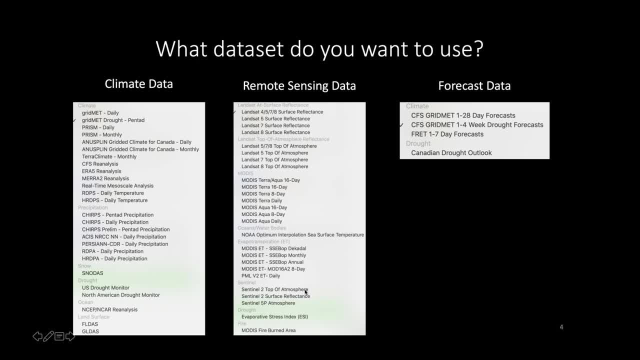 As well as some others, including Sentinel and some other products in there, And I also mentioned we recently had added the Sub seasonal forecast data from climate forecast system, as well as NOAA's forecast reference, ET and the Canadian Drought Outlook. So that is a long list of data products. 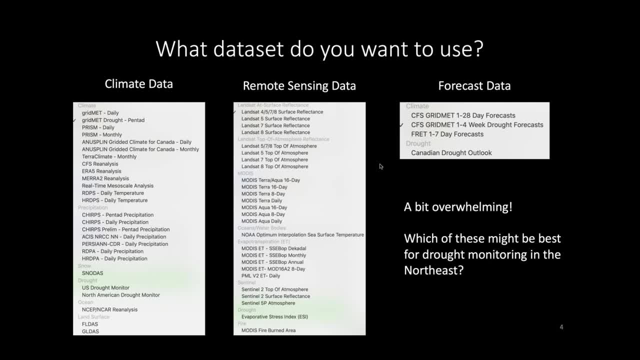 And it would be hard to come to climate engine and really know what to use unless you specifically already kind of know what you're looking for. And so what I'm going to do is walk through which some of these products that might be most useful for drought monitoring in the Northeast. 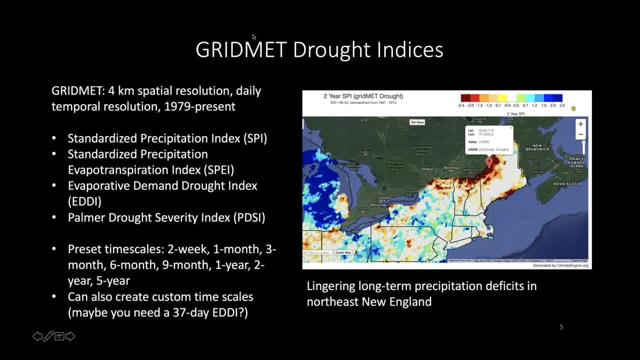 So I want to start off with the GridMet Drought Indices, And GridMet is a daily gridded product that was developed by John Abatzoglou at the University of Merced, And so this product extends back to 1979. 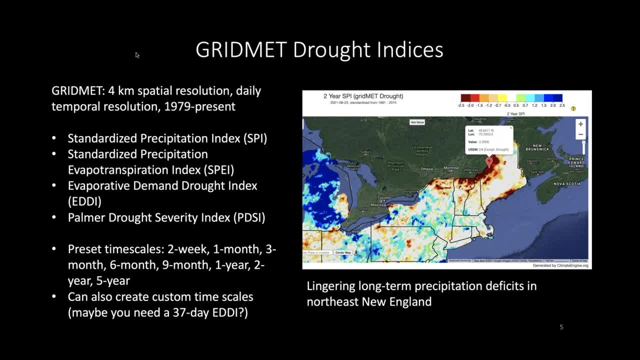 And it includes temperature, precipitation, wind speed, downward shortwave, radiation, humidity and several other variables at daily time scales, which is a great asset For drought monitoring And on climate engine. we have some of these in drought index form, including the standardized precipitation index, which is just precipitation. 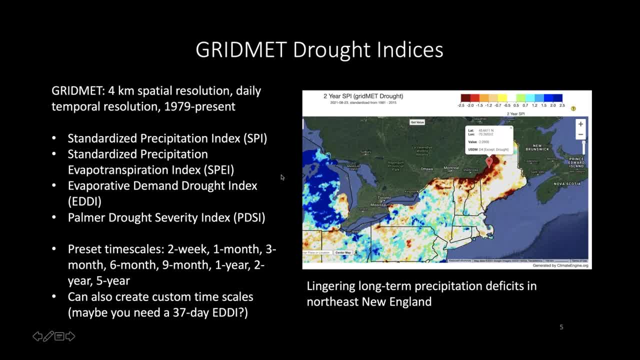 The standardized precipitation evapotranspiration index, which looks at the balance between precipitation and evaporative demand, And then just the evaporative demand drought index, which we'll hear more about from Mike later- the EDDI as well as the PDSI. 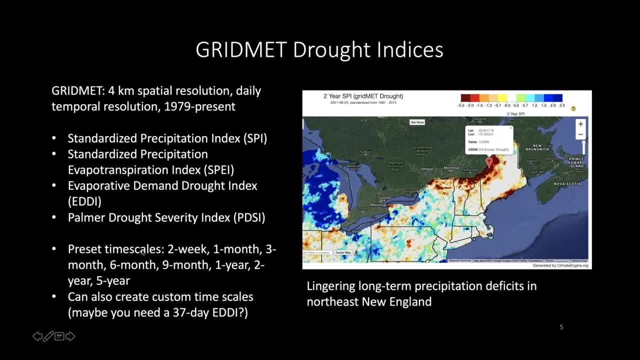 And so, with climate engine, we have some preset time scales Available, from very short sort of time scales that you might use for flash drought monitoring, like two week and one month. one time scales out to very long time scales- two and five year- that reflect the multi-year drought conditions. 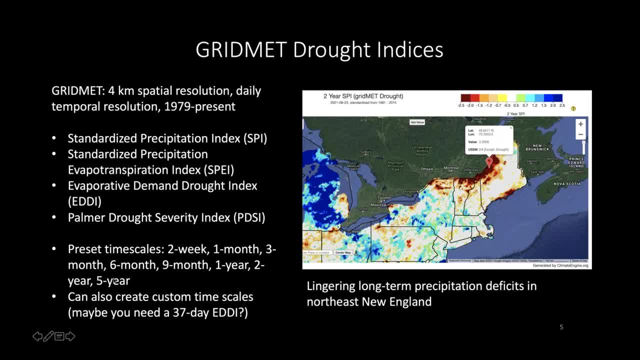 And aside from the preset you can create custom time scales if you want. Some people are interested in some, some you know odd number of days that they are interested for a certain drought and they can compare that to all the other time periods in the record. 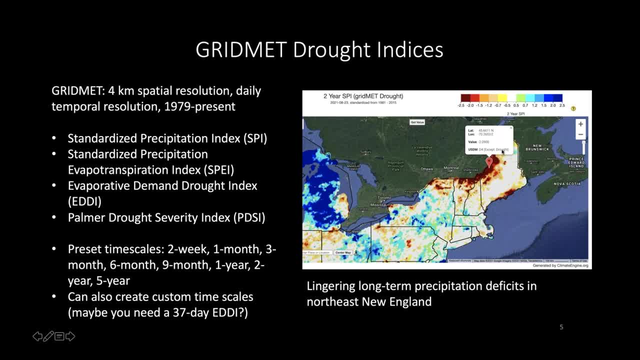 And so I'm showing here the two year SPI from GridMet, And this is from August 23rd, And so we can see some of these lingering red, these darker reds, in parts of northern New England, which shows lingering two year drought conditions there. 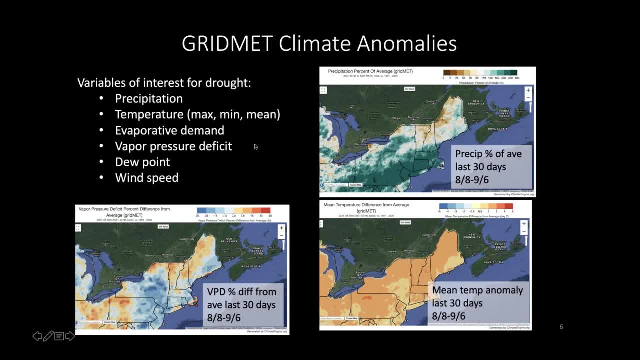 So, in addition to the drought indices, you might just be interested in the climate anomalies themselves, the raw values expressed as anomalies. Some of the ones for drought would probably be precipitation, Temperature, evaporative demand. We have vapor pressure, deficit, dew point and wind speed in there as well, which we use, those for the evaporative demand calculation using the Pem and Monteith. 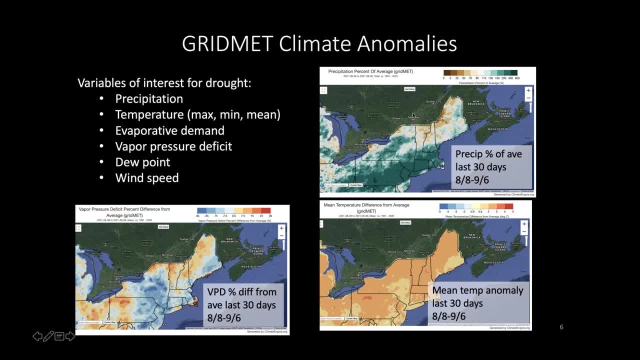 And so on the top right we have the precipitation percent of average and we have options for for last seven days, 15 days, 30 days, et cetera, or you can customize your, your period, And I was putting these together last week. 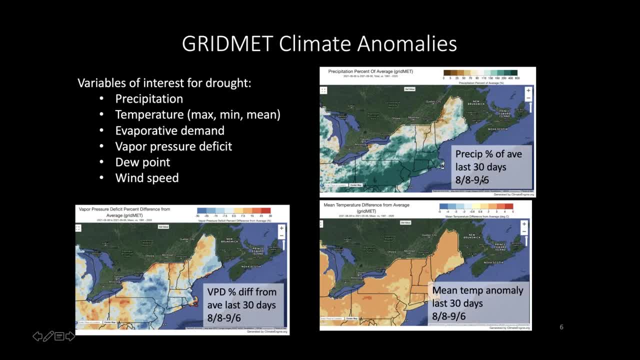 And there's usually about a two or three day lags. If you went on there today, you'd probably get GridMet data from about two or three days ago, And so we see the precip percent of average And then on the bottom right the mean temperature anomaly for the same time period. 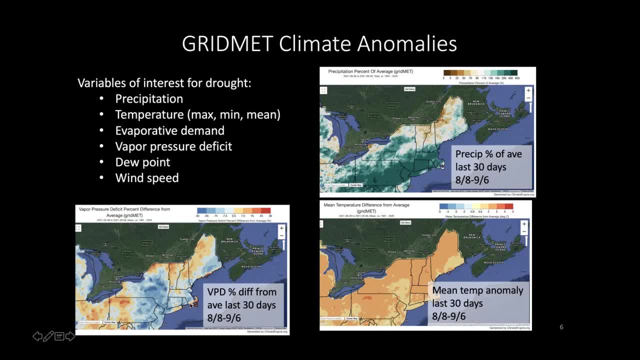 And then on the bottom left is the vapor pressure deficit, And you do have the option to express this as just a straight anomaly: a percent of average or a percent difference from average, because some of the variables might not. The percent of average doesn't work so well for something like vapor pressure deficit because the values are so small. 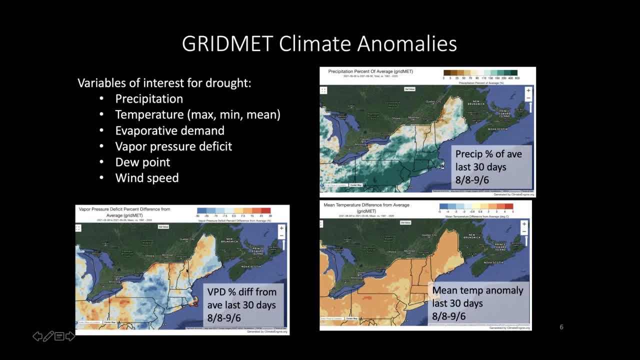 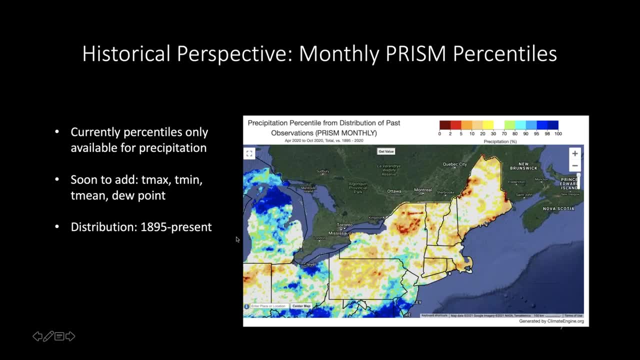 So you can look at the percent difference from average to really see that some of these higher vapor pressure deficit areas align with the drier precipitation areas. So, yeah, the GridMet tools are great, But one limitation of them is they have a shorter period of record relative to some of the other data sets out there. 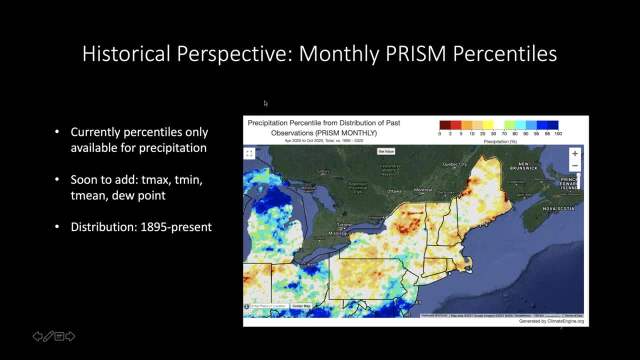 So, as I mentioned, that went back to 1970. 1979. But we also have the monthly PRISM data that goes all the way back to 1895. So you get a much longer period of record when you're looking at things like percentiles or the SPI. 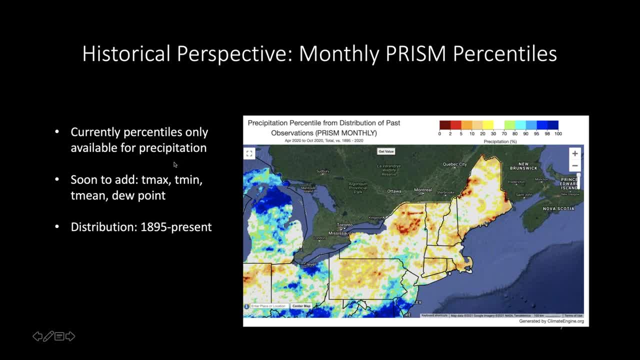 So we currently have the percentiles in there for precipitation And hopefully we'll have maximum mean temperature and dew point soon And so you can actually select the period you want to have for the distribution of the percentile. But for this example I chose to use 1895 to present for the April through October precipitation. 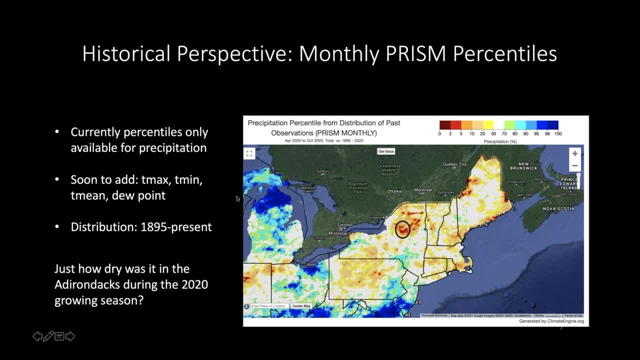 So this map is showing 2020.. And we see that. you know, overall there are some drier areas, but there's a lot of areas in the long term that were sort of near average or even wetter in parts of Pennsylvania and New York. 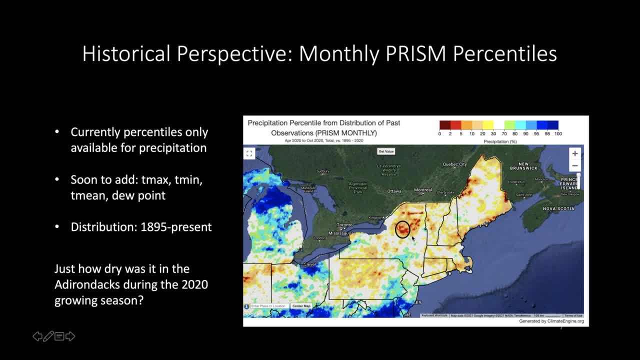 But one area that does stand out is the Adirondack Mountains in New York, And you see some of these drier grid cells showing up as less than the fifth percentile. And so then you might ask: well, you know just how dry was it. 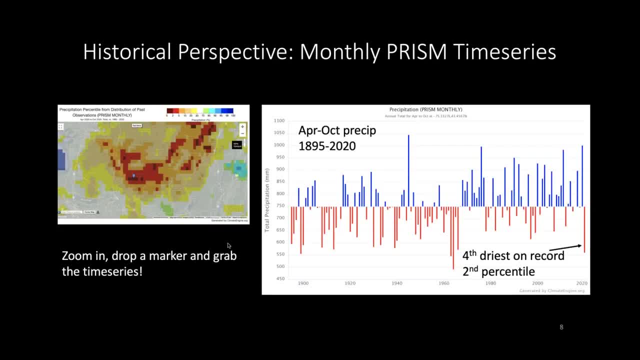 We see it's in those lower percentiles, But how does that compare? So what you can do then is you can actually just zoom into that area I highlighted before, which is shown here on the left, And you can go to, then switch over to the time series option and drop a marker in there wherever you want. 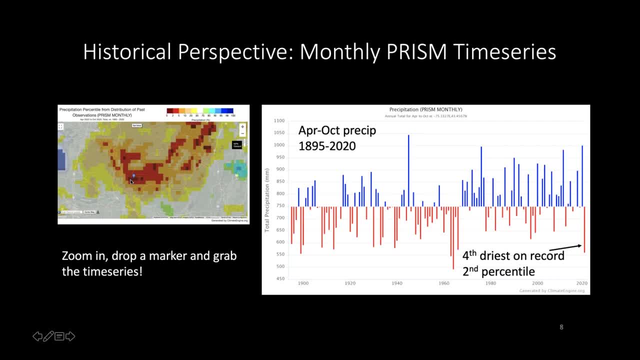 And so I dropped it in that little bullseye of zero, And then you can just plot the time series of all the April through October, going back to 1895. And so we do see, indeed, that it was in that lower percentile. It was the fourth, driest on record here in 2020, which comes out to the second percentile. 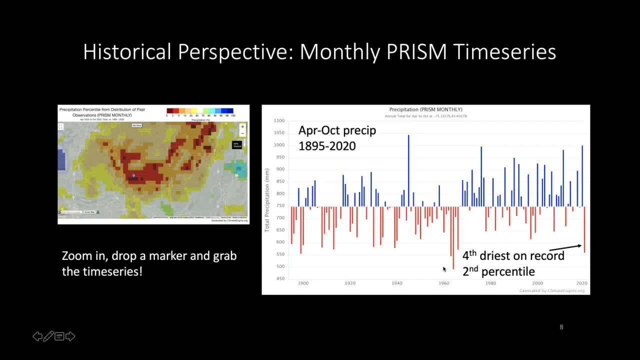 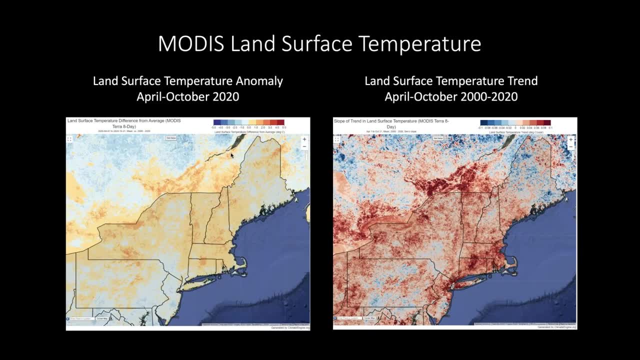 And it was almost as dry as some of those driest years that were in the 60s, where we saw a string of very dry years in this part of the North. So next I want to talk about a few of the remote sensing products. 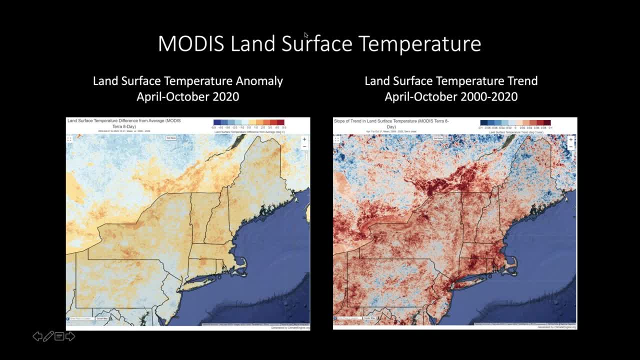 One is the MODIS land surface temperature, And I think Imtiaz will mention this as it's used in the LERI as well, And so these are the land surface temperatures, which is different from what we would see with, say, the gridmet temperatures, which are the two meter temperatures, the air temperatures. 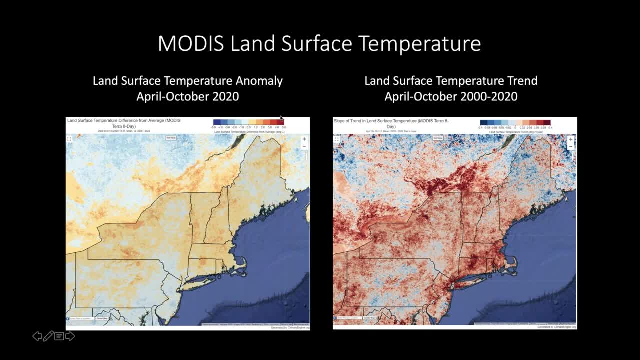 And so this is the actual temperature. This is the temperature of the land surface that you can look at, And the anomalies can tell you a lot about drought. where you have higher land surface temperatures, You have a hotter land surface, typically lower evapotranspiration and drought conditions in those areas. 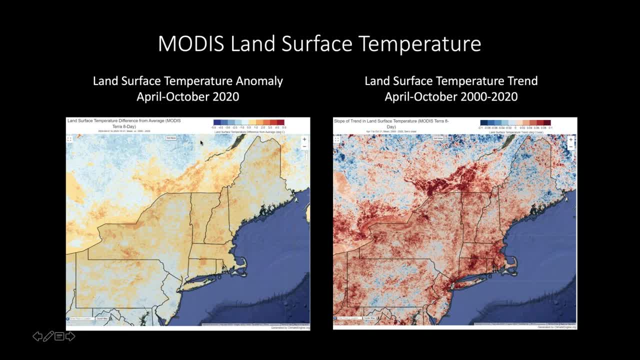 And so this was the growing season land surface temperature anomaly for 2020.. We do see a lot of areas with above normal land surface temperatures. Another feature that was recently added to Climate Engine was the ability to plot the spatial trends, And so I looked at this map on the left and you can say: well, how has that changed over time? 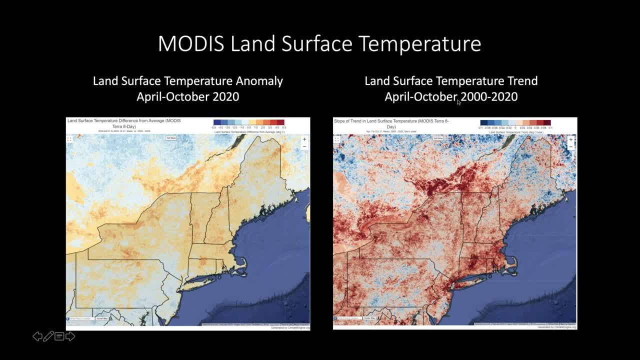 And so you can select a period, so April through October, and plot the trend spatial. So for each grid cell it's taking that 20 year time series and computing the trend in degrees Celsius per year here And we see a pretty strong warming trend in the land surface temperature over that 20 year period. 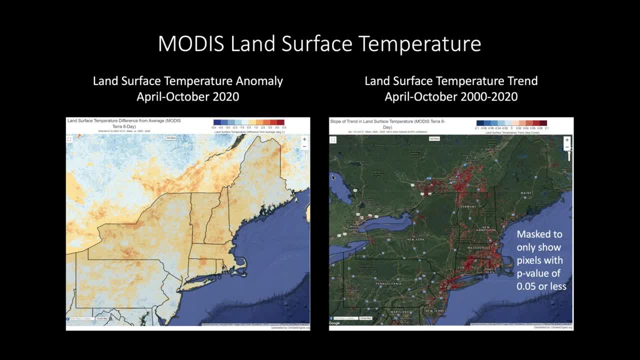 And so another option you can do then is so when you look at a trend, you got to be a little cautious, especially if it's a shorter period of record, And so you do also have the option then to mask that based on key value or the significance of the trend. 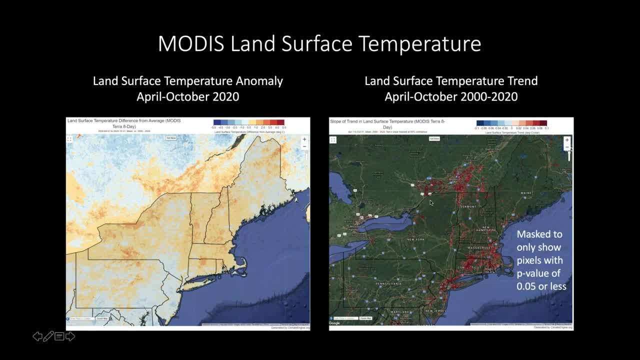 And so what I've done now on this slide on the lower right is only showing the values With a p-value of 0.05 or less or 95% confidence, And we see those areas in parts of New England mostly that had a stronger trend are indeed significant trends. 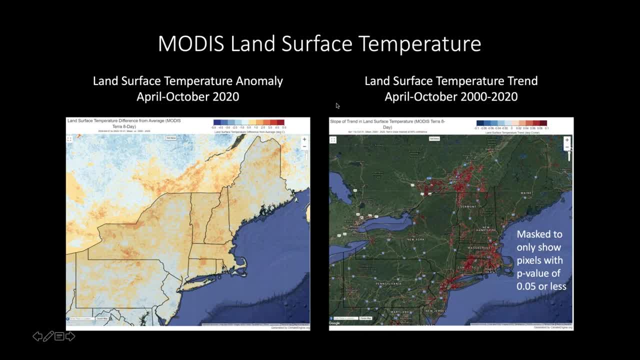 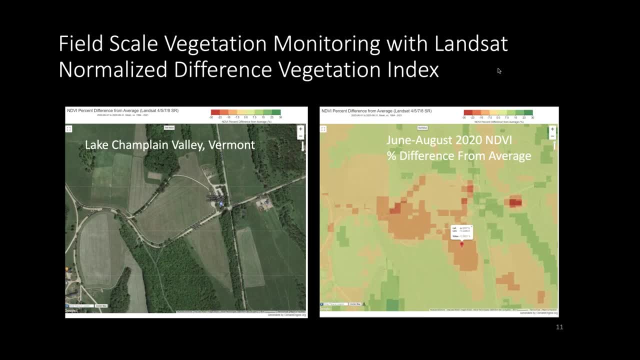 And so that's a nice feature if you wanted to do a quick spatial trend analysis in Climate Engine. And last product I wanted to mention was field scale vegetation monitoring with Landsat Using the normalized difference vegetation index, And so with MODIS that went all the way back to 2000 and Landsat we have all the way back to 1984. 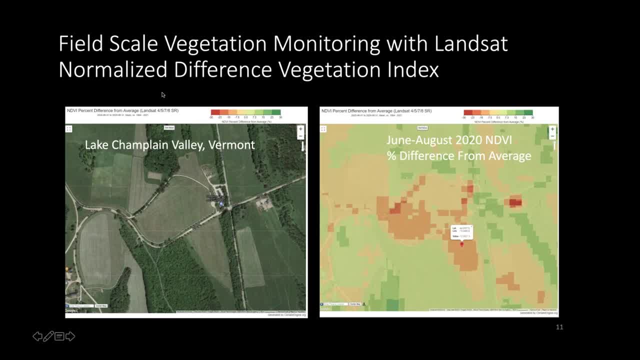 So you get a bit of a longer period of record. So what I'm showing here on the left, and so, as I mentioned, you can use the transparency bar in Climate Engine to actually look at the map. And so I zoomed into an area in Vermont, in the Lake Champlain Valley, south of Burlington, that is a AG area. 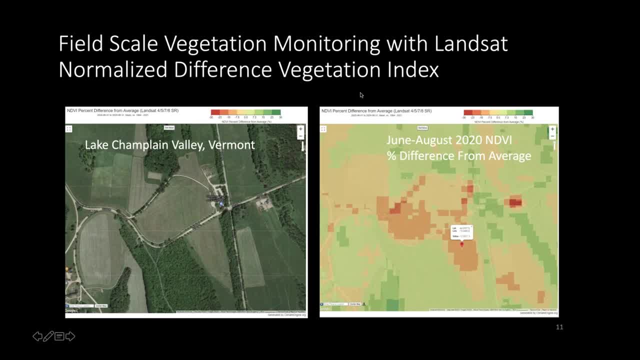 You can see the AG fields here, And then on the right is the map of the percent difference from average NDVI. And so the NDVI gives you a measure of vegetation health or greenness. So higher NDVI would be greener and lower would be browner or less healthy vegetation. 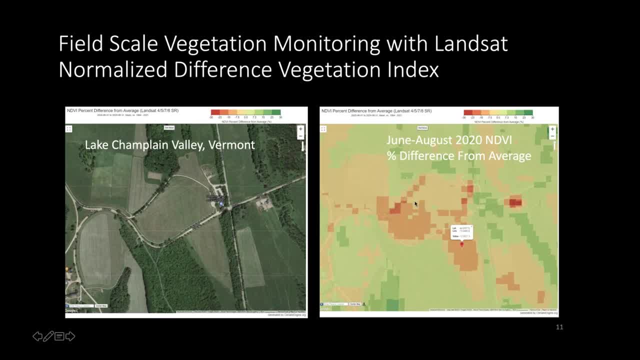 And so we do see in 2020 for the summer NDVI that in these fields it is showing below normal NDVI And I highlighted a grid cell there that says it's about 12 and a half percent. It's below normal. And so what does that really mean? 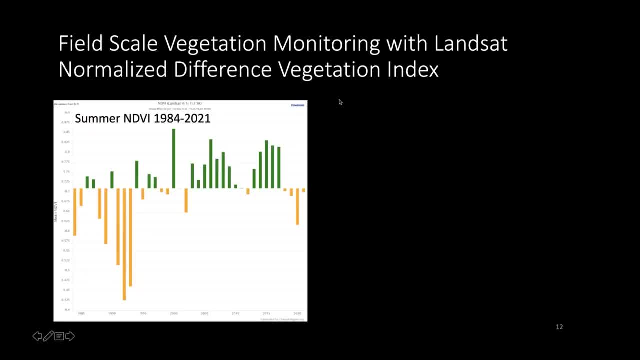 What does it look like through time? You can then again go dig in, And so I clicked on that grid cell and then went to the time series And you can plot the summer NDVI through time, And so this is 1984 to present. June, July, August mean NDVI values. 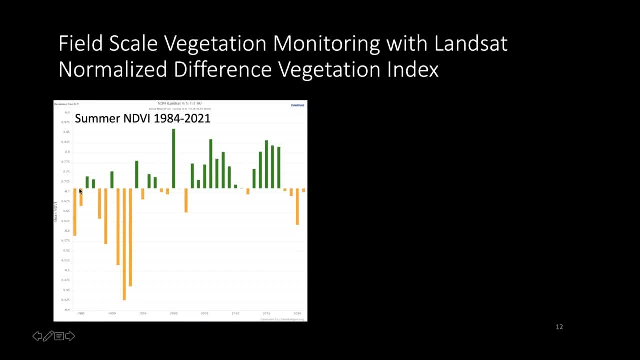 This line, separating the green and the yellow bars, is the mean, And so a few things stand out. We do see 2020 was lower than that average, And so if you do know about your own region, you might know about this specific field. 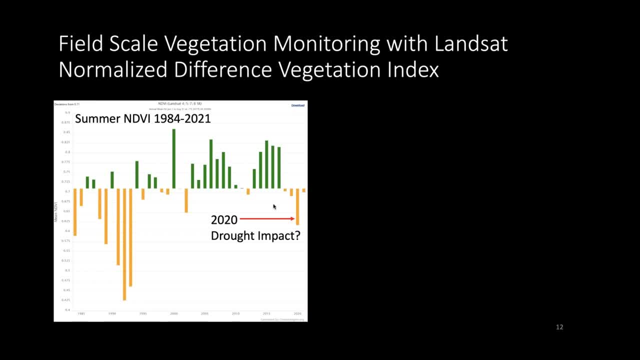 You can then say a lot more, But just looking at this, we don't know necessarily if that was a drought impact. It could have been a drought impact because we see, other years in the past were higher NDVI, although 2016 was pretty high. 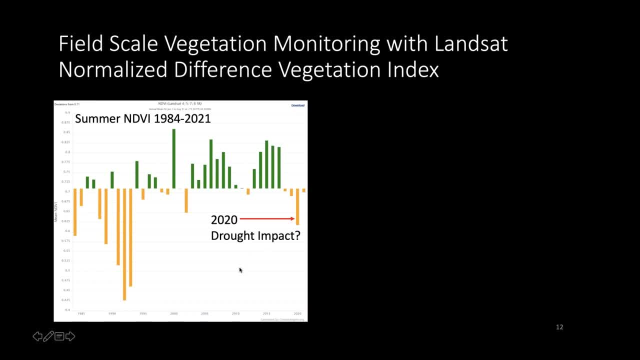 And so It doesn't stand out in that sense. Then you look back further in time and you see these. you know, for an ag field, you know the summer NDVI is going to be high. It's going to be 0.7 to 0.9.. 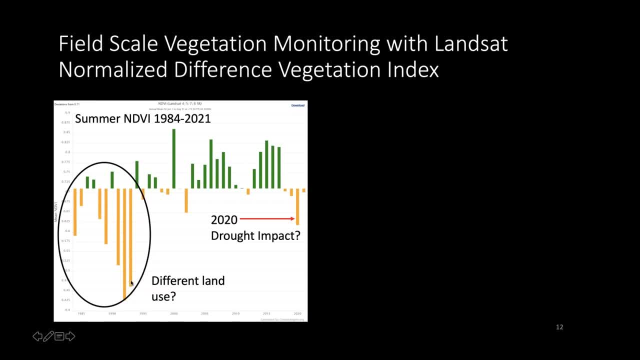 And you see all these values in the early part of the record: 0.4, 0.5.. And so it makes you wonder: was this not a farm back in that time period And was there a different land use? So you can start separating these different types of drought versus human impacts, versus land use. 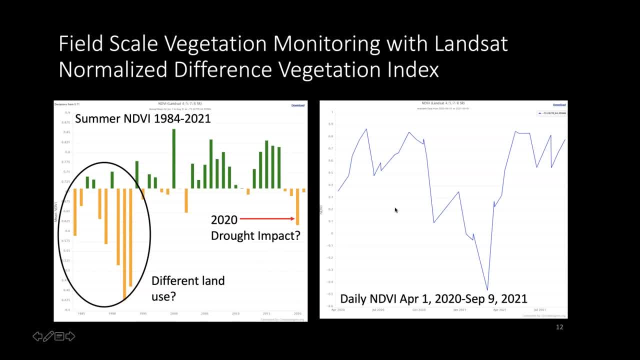 And then, if we zoom in even further, this is now showing the daily NDVI, or from Landsat. it's once every eight to 16 days, from April 2021 through present, And so we see the seasonal cycle, where it's high in the summer. 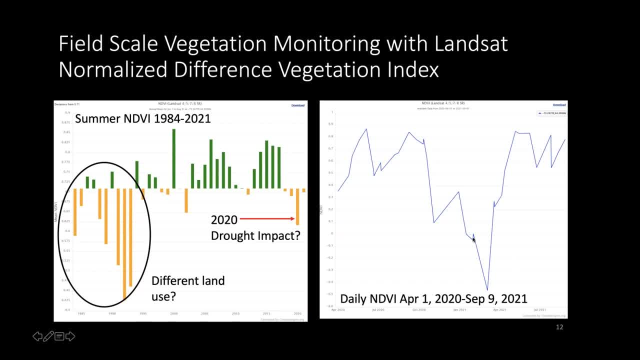 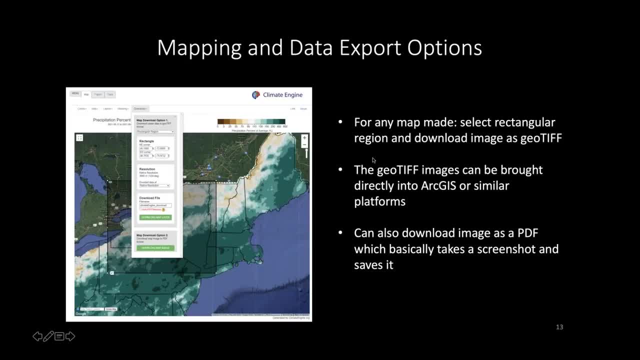 And then, when it's snow covered, it goes to these negative values, which really don't mean anything from NDVI perspective. But we can't. What we can see are these dips in the summer. Oops, sorry about that. These dips in the summer are actually cuttings or harvesting of a crop. 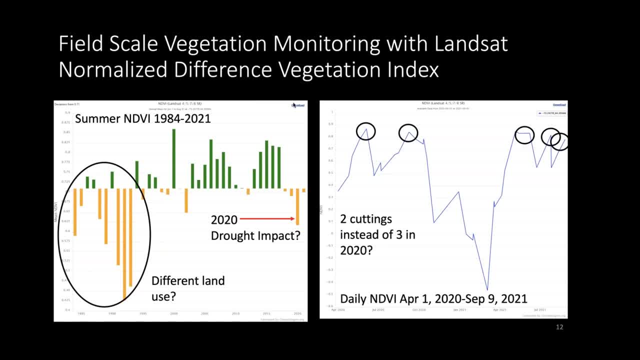 And so I don't know what was planted there, but you can see that in 2020, there was what appeared to be one cutting, And then something happened in the middle of the summer where they didn't seem to get a full cutting. 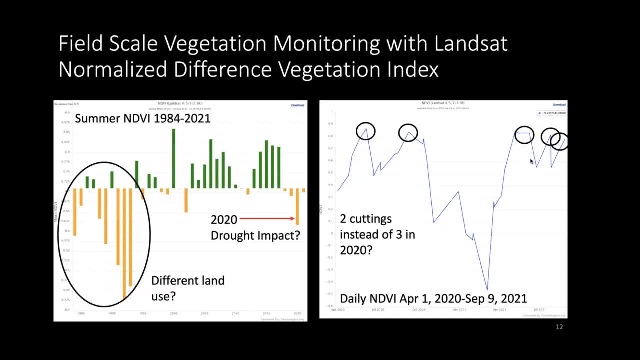 And then it grew back to full greenness later in the summer, Whereas this year, in 2021, there were two full cuttings already And it looks like they could get a third crop or a third harvest, And so was that a drought impact. 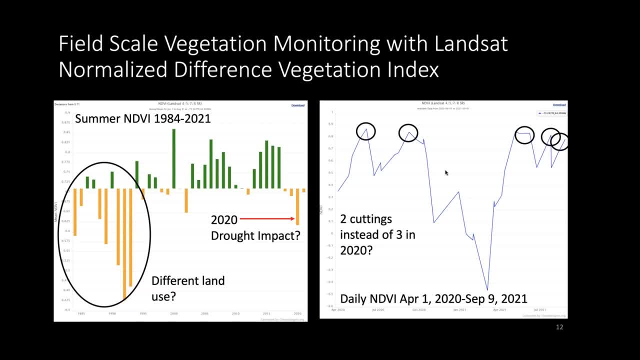 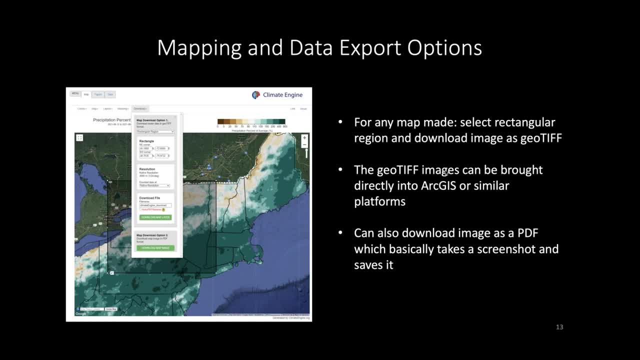 We don't know, But again, if you know more about your specific area, you can make more conclusions about these data. OK, so now, what can you do with the data? How can you access on your own? And so, for any of the maps I've been showing or any maps you make, you can draw a rectangular box and export them as a geodata. 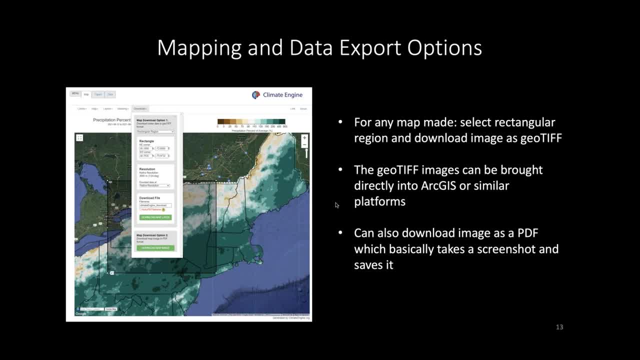 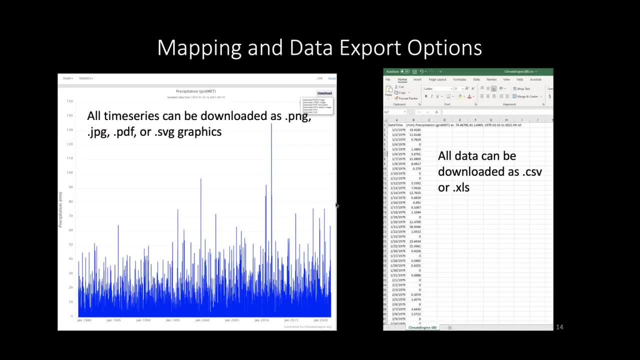 You can also download them as a PDF, which basically takes a screenshot of the image, And I showed a bunch of time series, So with any of those time series you have the download button here on the top right where you can download that picture as a PNG, a JPEG, a PDF or an SVG. 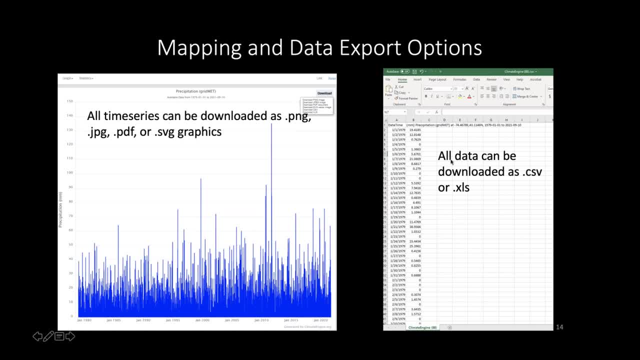 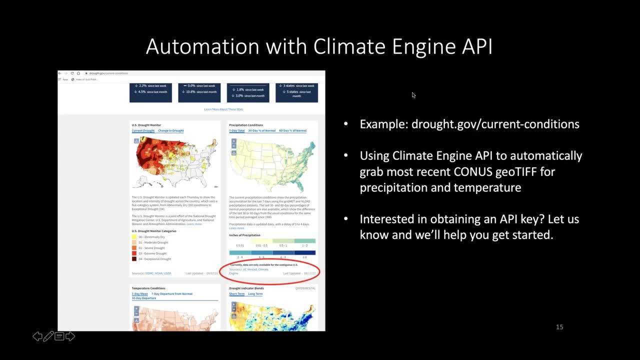 And then you can also grab the data too, And you can download that as a CSV or a PDF, And then you can use that as a PDF or an Excel file, And so, lastly, I did want to mention that there's an API in development with Climate Engine. 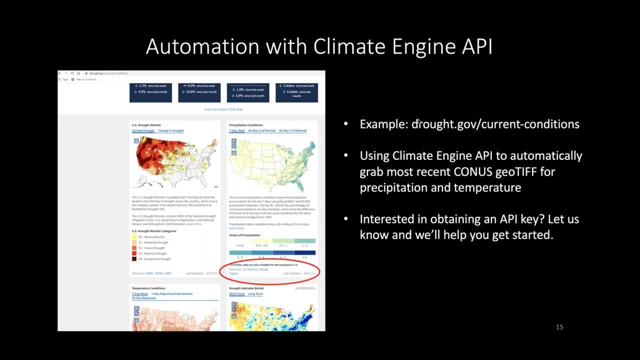 This would allow you to automate and put use write code to access some of this. you know on a daily update type of status, And so the example I wanted to highlight is what Droughtgov is actually doing with Climate Engine. If you go to their current conditions page you'll see they have some of these seven-day totals- 30-day percent of normal, 60-day percent of normal for precipitation and temperature- in some of the drought indices. 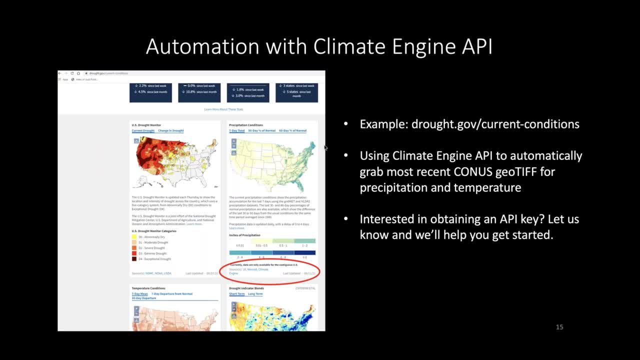 And so they're actually using the Climate Engine API to hit Climate Engine each day and get those precomputed values and use them in their own web development, And so at this point the API is still in development. So if you are interested in obtaining an API key, please let me know and we could help you get that and perhaps do some testing of this API for us, like Droughtgov is doing. 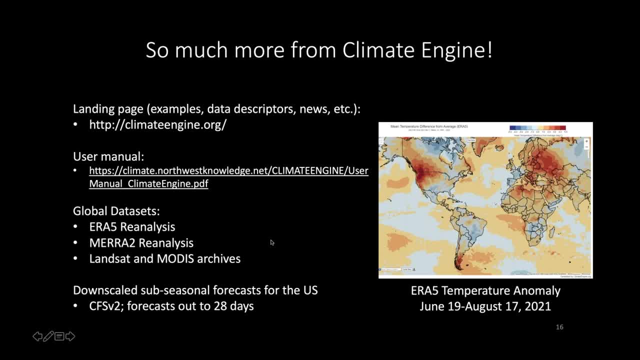 And so I'll just wrap up by saying there's a lot more available. It's kind of overwhelming sometimes. what's in Climate Engine? Here's our landing page. There is a user manual, a very detailed user manual with examples. There are global data sets. 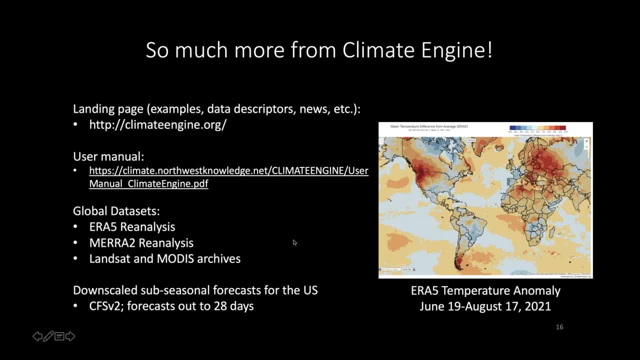 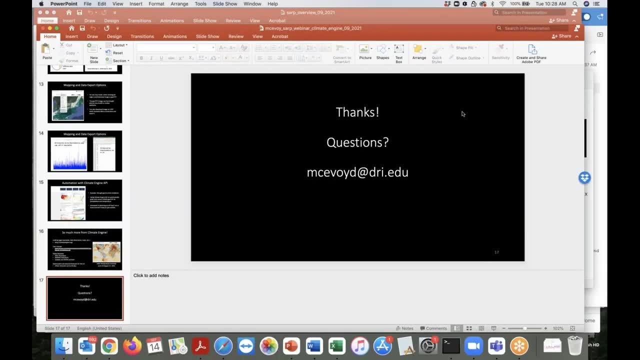 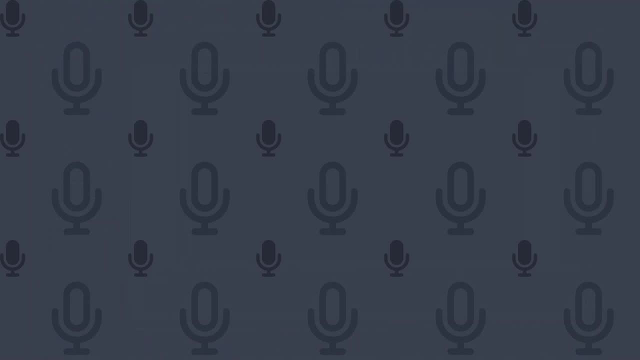 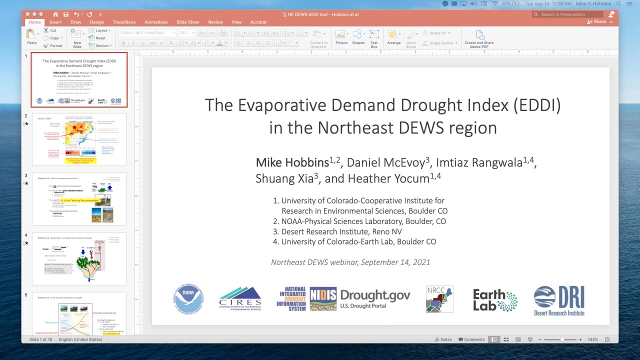 There's the seasonal forecast, which I wasn't able to get into today, But I will end there and we will hold questions to the end And I will pass it now over to Mike, And Mike, you should get that now, Okay. 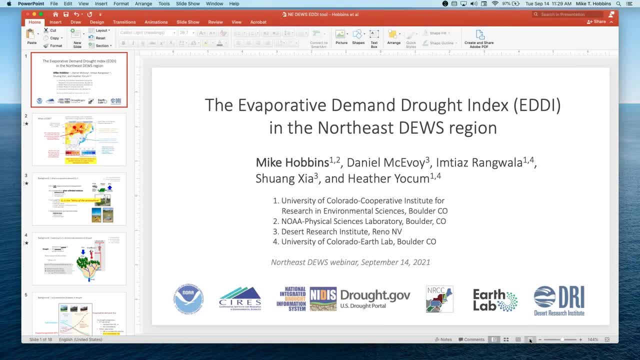 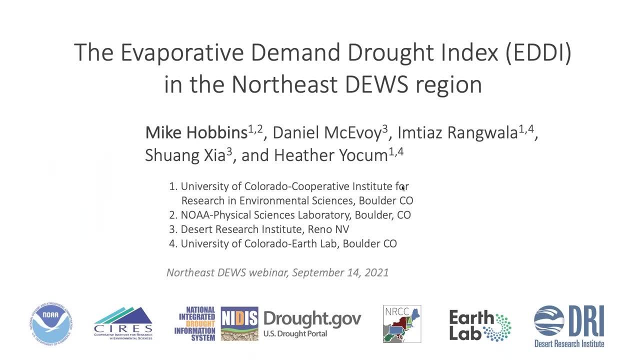 Okay, you see my screen And let's turn to presentation mode. Okay, Yep, Looks good. Okay, Excellent, Great. So thanks for that, Dan, And for a few plugs in there for Eddie. But here we go, Diving into a bit more detail about what Eddie is, Evaporative Demand, Drought Index and what it can do for the Northeast region. 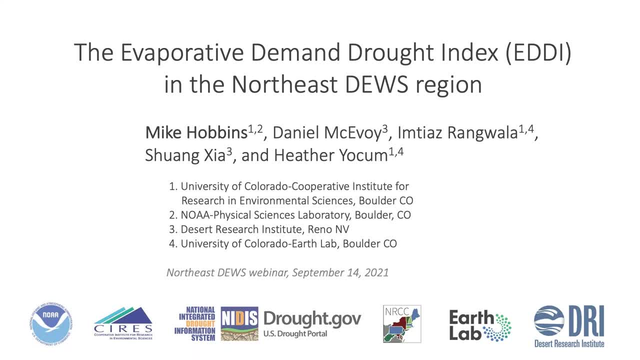 Dan's already introduced the team And here we are again: The salad of logos. What I'm going to do here is quickly go through some background on Eddie and evaporative demand That underpins it. So basically what Eddie is, how it's estimated, how it works and what it can be used for. 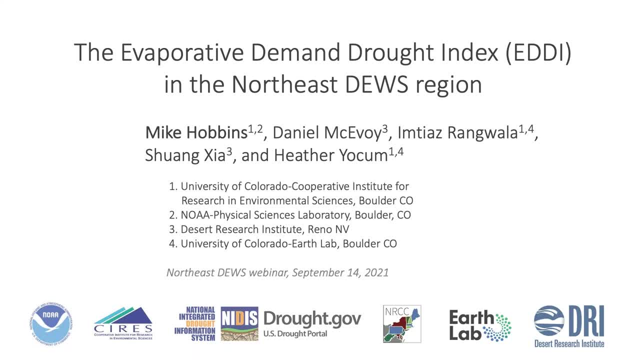 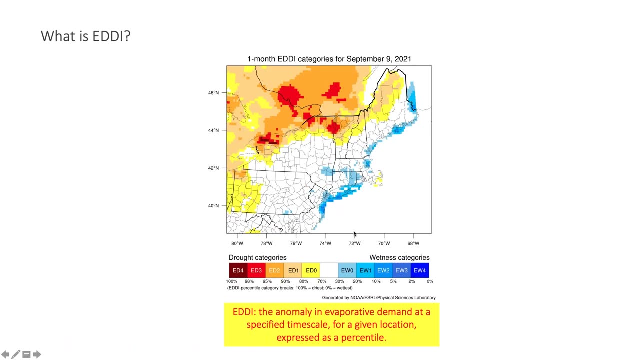 And how you can find out more, and how you can find and download the data and the maps for the Northeast dues. So let's get going. So this then. I'm trying to advance the slides. There we go. This is the most familiar iteration of Eddie. 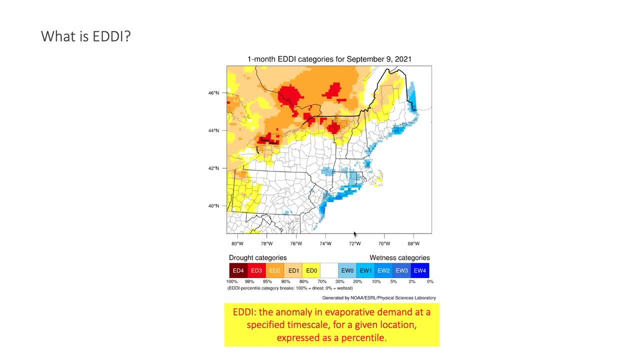 What Eddie looks like. It's like most familiarly And it's a map of the Northeast dues, clearly with counties and states, And you'll see that there's some various labels and timescales indicated. So what Eddie is in a nutshell, it's the anomaly in evaporative demand, which I'll talk about in a second. 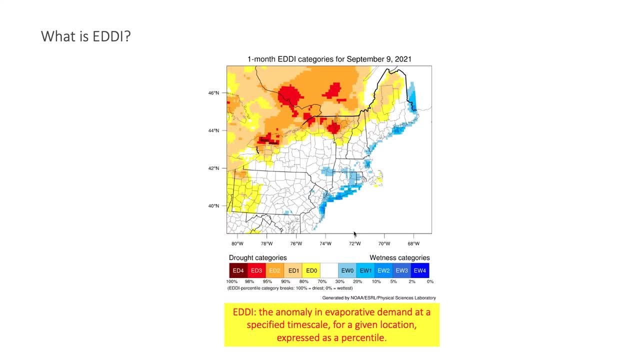 At a specific timescale, mapped across given locations, And it's all expressed in percentiles. So this here, then, is the one month Eddie, Which means actually 30 days. So this is one month Eddie, then. I downloaded it yesterday And it covers the period from August 11th to September 9th. 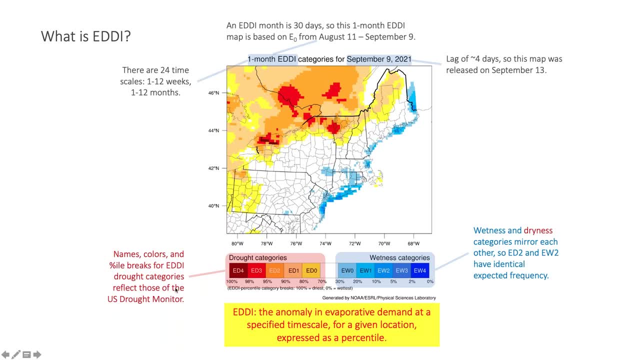 30 days. It was released. Like I said, it was released yesterday, But it was September 9th, So there's a lag of four days. That's because the driving data aren't available for four days. We have a bunch of different timescales. 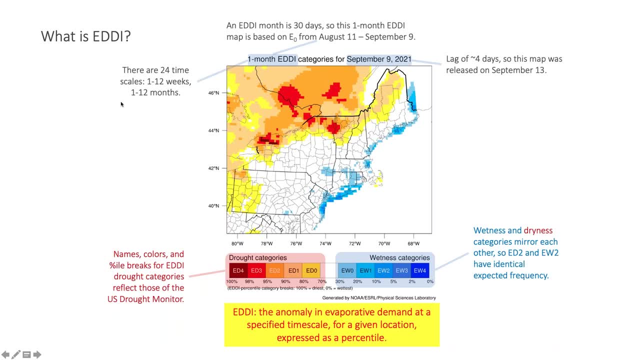 There are 24.. One to 12 weeks And one to 12 months, So from really super dynamic weather scale out to above seasonal scale, Annual scales, And it's mapped in terms of warm colors. down here Which are the drought categories: 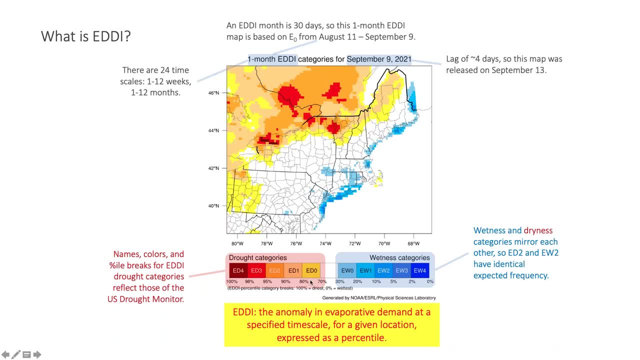 Which match very well to the US Drought monitor: drought categories, The same colors and same percentile rates, And on the opposite side, we have wetness categories, Which are at the flip side. Okay, So what does this map show us? for example, 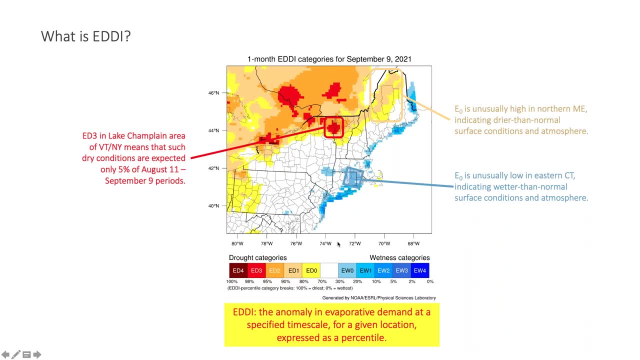 So here we see, you know, in northern Maine, for example, we see evaporative demand is unusually high. That indicates growth, That indicates drier than normal surface conditions and the atmosphere. There's a connection between the surface conditions and the atmosphere. 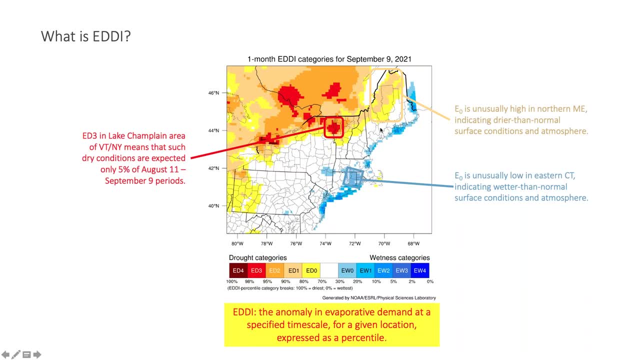 And that's what we're seeing in northern Maine And actually more intense drought in the Lake Champlain area of Vermont and New York. And you'll see here, this is ED3. Which, if you go down to the key, is between the 98th and 95th percentile. 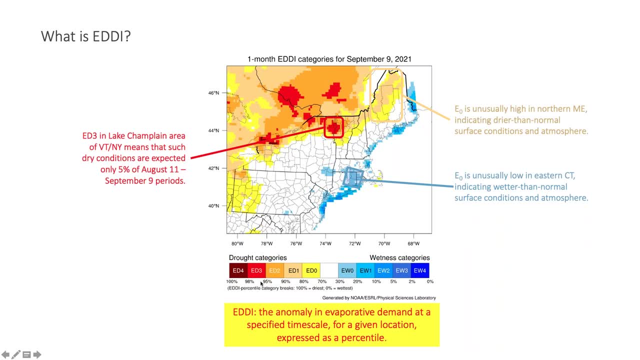 So you would expect to see these conditions, only 5% of those periods, Of those August 11th to September 9th periods. And EDI is based on a time series of evaporative demand. It goes back to 1980.. 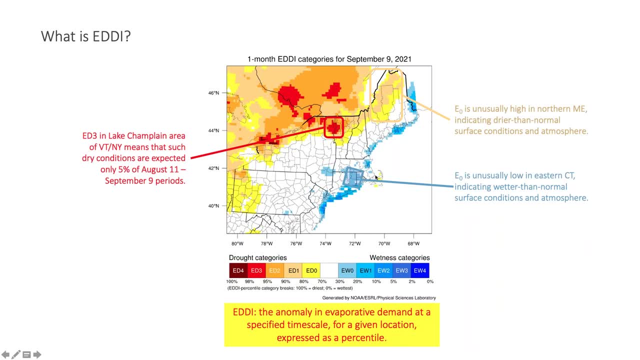 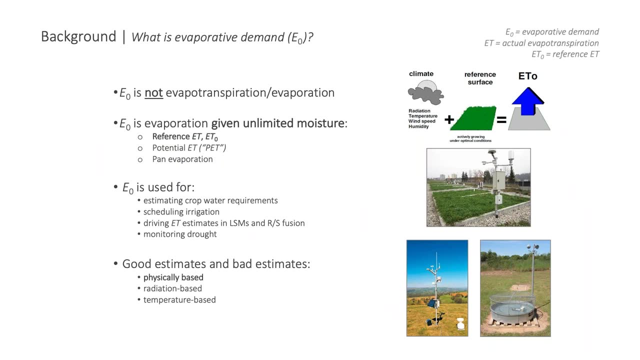 So it's over 40 years long. right now, And on the opposite side, here you see, in eastern Connecticut, it's wetter than normal. Okay, So backing out a little bit further, what is evaporative demand? So you may be familiar with the expression PET, or potential evaporation, or reference ET. 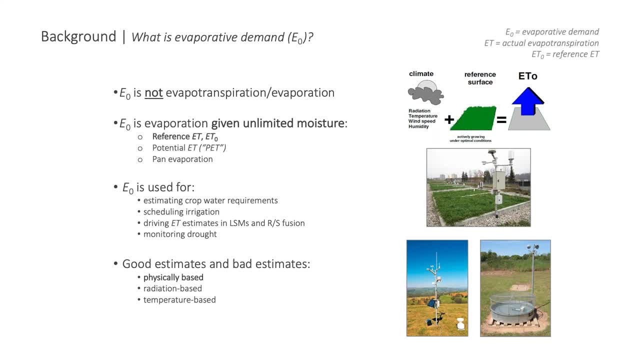 So what we talk about here is reference ET. Evaporative demand is an umbrella term that's given to reference ET, potential ET and PAN evaporation. It's not evapotranspiration, It's not the actual flux, It's the demand in the atmosphere for moisture at the surface. 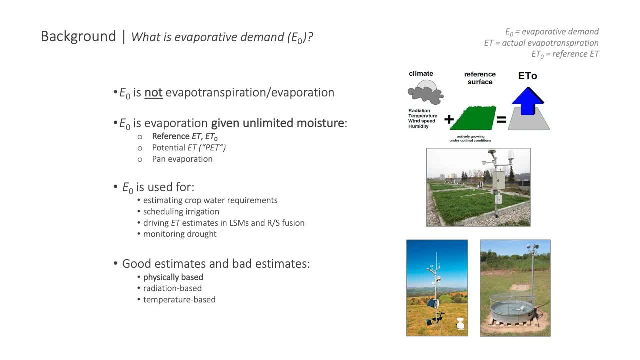 So it's used for crop water requirements, irrigation scheduling, It's used in land surface models, But we're using it here for monitoring droughts And we're using a physically based estimate of evaporative demand. We're using the Penman-Monteith reference ET equation. 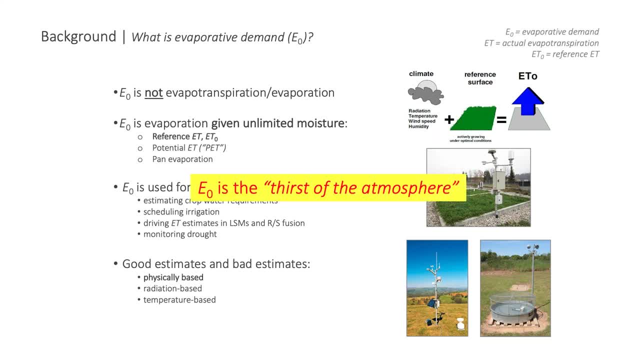 So simply, you can think of evaporative demand as the thirst of the atmosphere, And it makes sense that the atmosphere and the land surface are linked. When the land surface is linked, When the land surface is drier, the atmosphere is more thirsty. 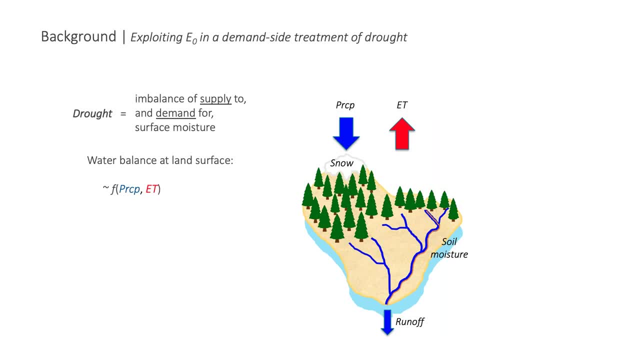 That's sort of in a nutshell. So how do we use it to measure drought? Well, historically, drought is an imbalance between supply and demand for the surface moisture. But historically we've estimated the evapotranspiration, the return flux of moisture from the land to the atmosphere. 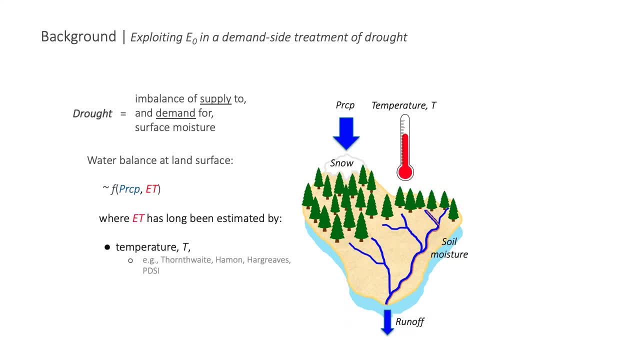 as a function of temperature, which is not a good estimate. What we're doing here is replacing that with a demand that's physically based. It's a function of these variables- Temperature, specific humidity, wind speed and solar radiation- And it's more physically driven by soil moisture status at the ground. 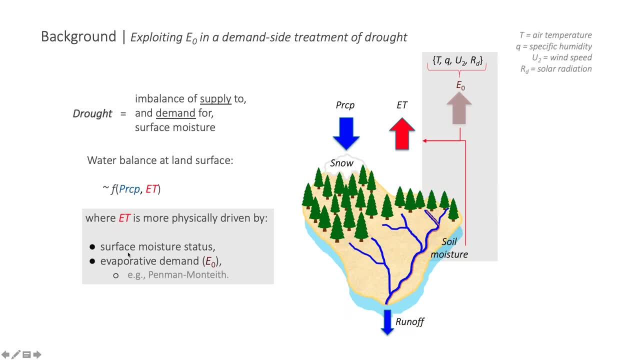 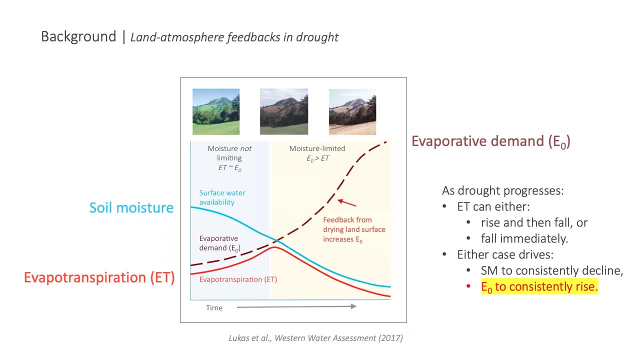 where evapotranspiration is physically driven by surface moisture status and evaporative demand. OK, So boiling this down to the land surface fluxes and states that we're interested in, we see that as time progresses, if you think about this graph in terms of time running from left to right, 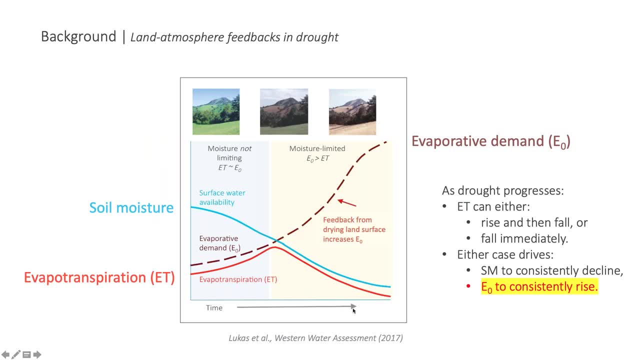 as time progresses, through a drought, through a drying anomaly, precip can decline and meteorological anomalies force drying, whether it's through excess temperature, sunshine, wind or low humidity, Evapotranspiration, which is the actual flux, can rise in response to that elevated evaporative demand. 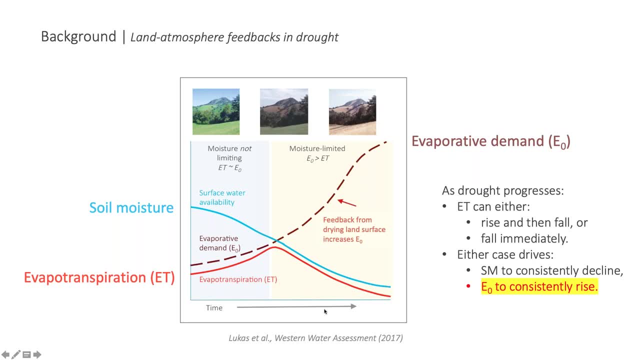 and then crash as soil moisture dries out. There's simply no more moisture available, But evaporative demand always increases in drought, Which makes it The response of evaporative demand is often detectable earlier than that of soil moisture, which can make evaporative demand a leading indicator of drought and of flash drought, as we'll see. 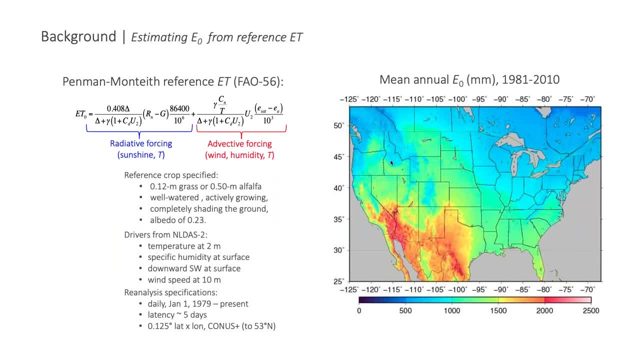 OK, So how do we then estimate eddy? First of all, we start with generating a time series of evaporative demand And we use, like I said, the PEMM-1T reference ET. It encodes radiative forcing and effective forcing. 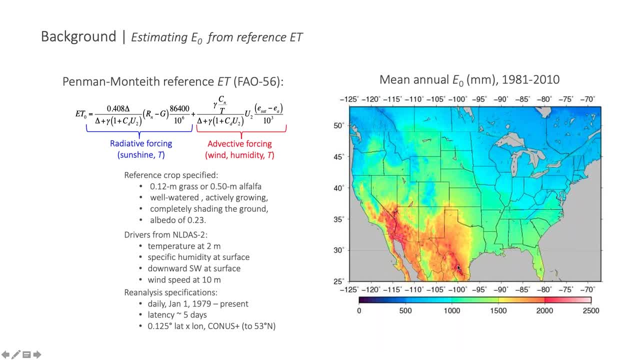 The details aren't that important here, But here you see a map of evaporative demand, mean annual evaporative demand across the continent of the United States And clearly it makes sense. Evaporative demand is higher if the atmosphere is thirstier. 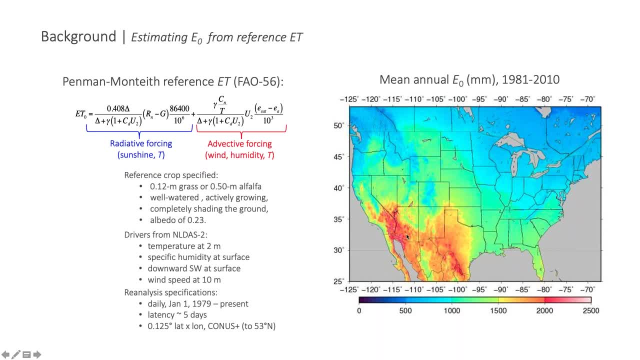 where it's hotter, windier, sunnier or drier, And up in the northeast it's not those things. So it's lower than in other areas of the country. So we take that evaporative demand. This is to calculate eddy. 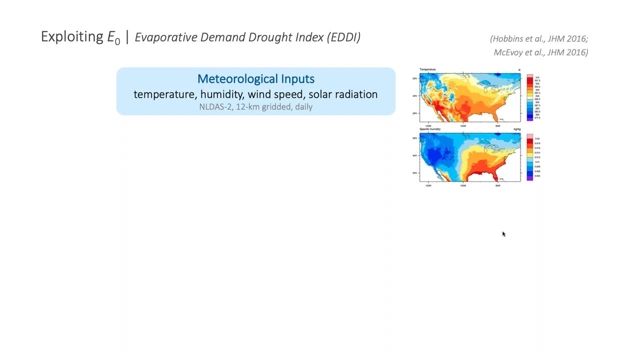 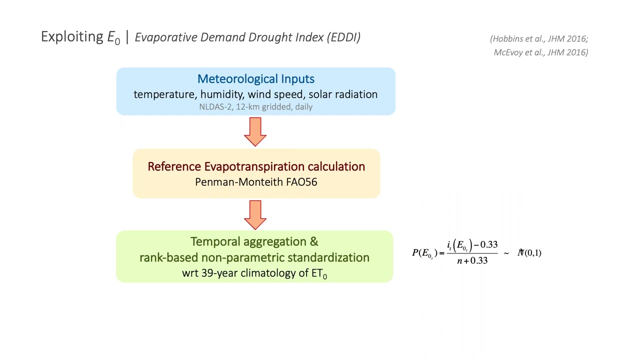 We take that evaporative demand reanalysis that's driven from NLDAS to temperature, humidity, wind speed and solar radiation. We calculate reference ET from it And there's that map again And then for our period of interest we aggregate evaporative demand at each pixel in the data set. 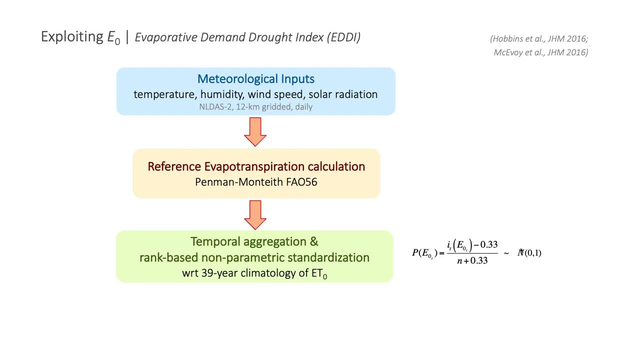 And if it's a month, then we aggregate one month's worth of evaporative demand And we compare it to that same month over the entire 42,. well, this is an out-of-date slide, 42-year record And we convert that into a standard normal distribution. 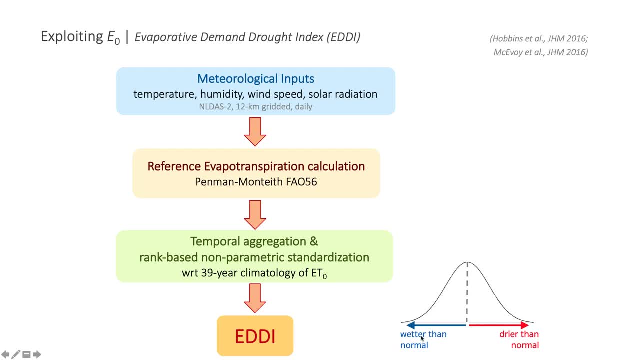 So, where anything is, anything on the left side of the bell curve is wetter than normal, The bell curve is absolutely normal, And anything on the right side of the bell curve is drier than normal, And that's what we evaluate as eddy. 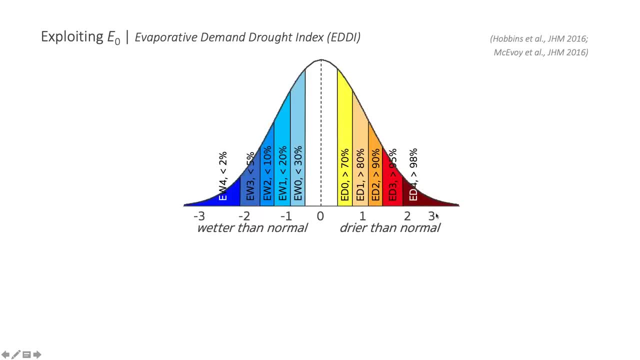 So, eddy, then here's that bell curve again. The extremes on the dry side are ED4. That's over 98 percentile. So it would only occur 2% of the time, And the extreme wet would only occur 2% of the time as well. 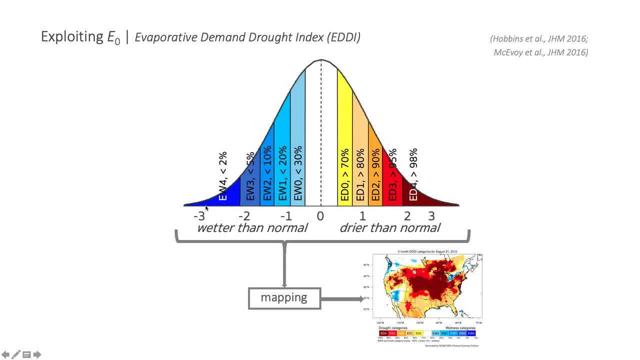 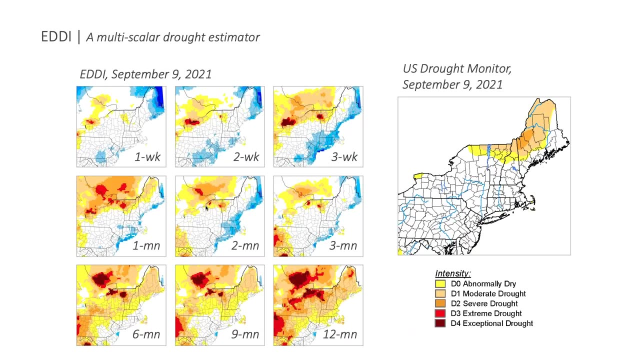 And that's EW4.. And that's calculated for each pixel, So we can map it across cones. As you see here, this is a 2012 graph. So how can we use eddy? Well, for a start, the first thing to note is that eddy is multiscalar. 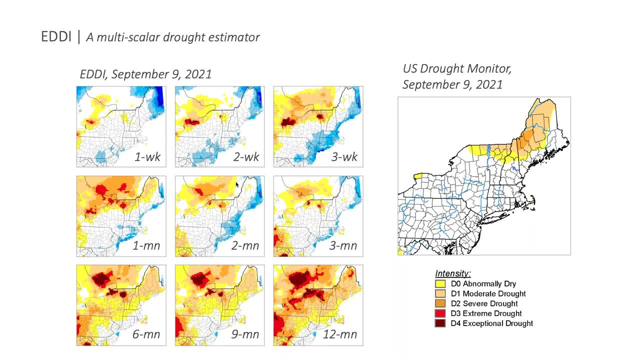 Like I said, we have these 24 timescales Here. I've just picked out nine timescales for the same date, So this is September 9th. I made this graphic yesterday And you can see that eddy operates differently at different timescales. 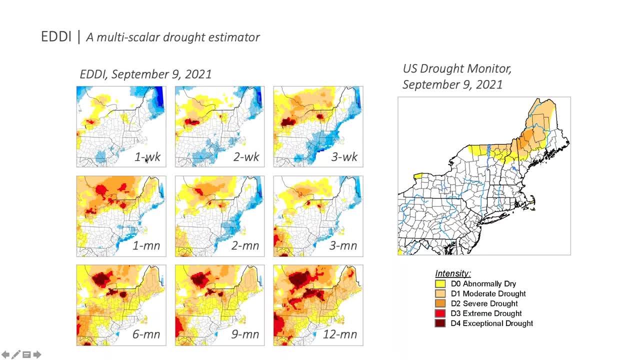 This is the last week of eddy in the Northeast. This is the last two weeks and the last three weeks, And here you're really probably seeing Hurricane Ida. It sweeps up the coast of the Northeast and it's just dumped a bunch of rain. 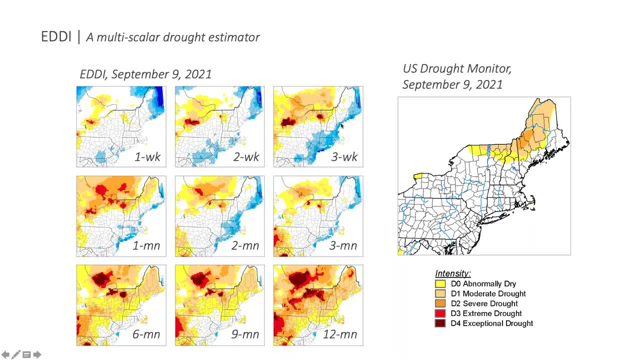 And it's made the atmosphere moister than normal over that three-week period. But if you move down to the 12-month period, you're really seeing the effect of that 2020 drought, or the remains of the 2020 drought Where it's ED4 up in northern New York and Vermont. 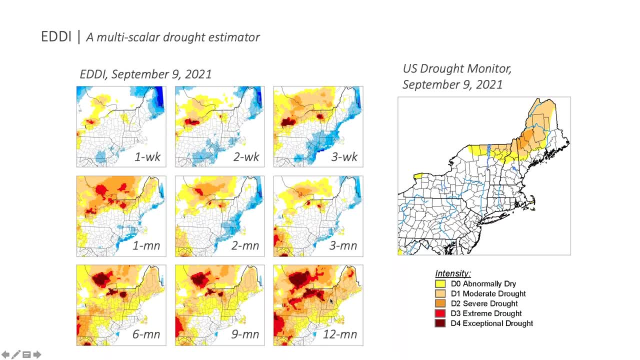 And it's drier than normal almost everywhere through the region. So eddy is multiscalar and it captures different drying dynamics that operate at different timescales, So the optimal timescale is specific to your region, your season and your sector. 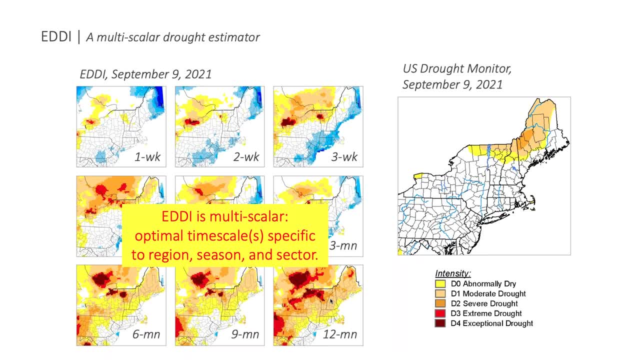 So, for example, as Zia showed us last week, for example, the one-month eddy is strongly correlated with crop yield for corn and silage in New York, New Jersey and Pennsylvania, But these are state averages with a correlation of 0.6 or more. 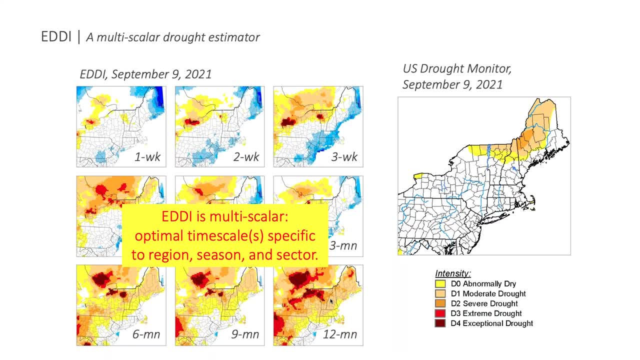 So some regions will be much more strongly correlated. Like the optimal timescale can vary through seasons and regions, The strongest correlation to crop yields of corn and silage in New York is for the two-week to one-month eddy, And it's in May, for example. 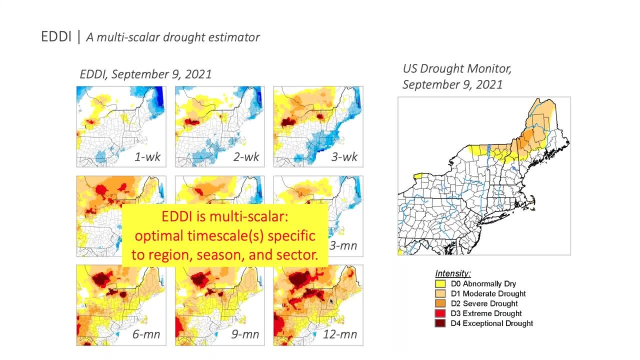 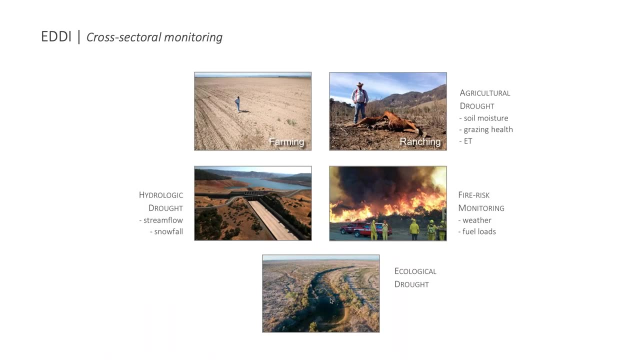 So these are just examples to show that regionally and seasonally, and sectors affect regions, seasons and sectors affect what the optimal timescale for you would be. So for crop yield they were generally around one to three months. So what can you use to calculate? 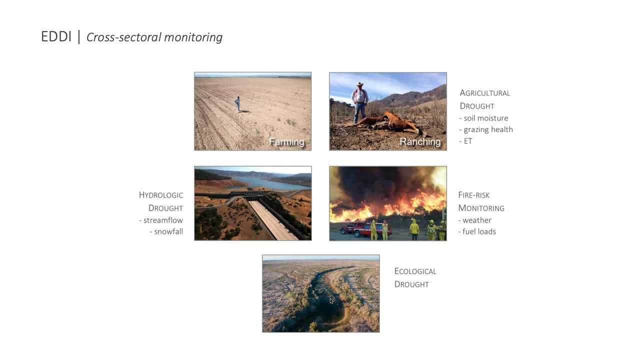 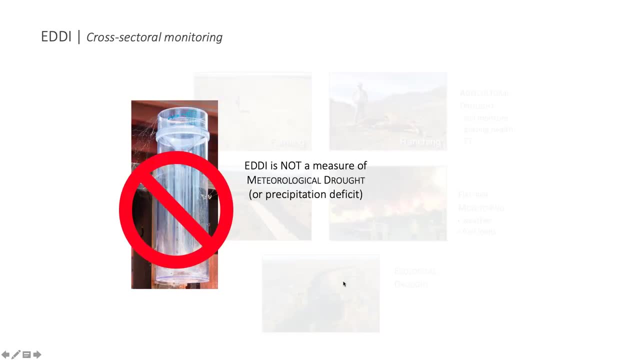 What can you use eddy for? Well, you can use it in farming, ranching, which obviously we're not doing in the Northeast- but also for hydrologic drought, for fire risk monitoring and for ecological drought. But what eddy is not is not a measure of meteorological drought. 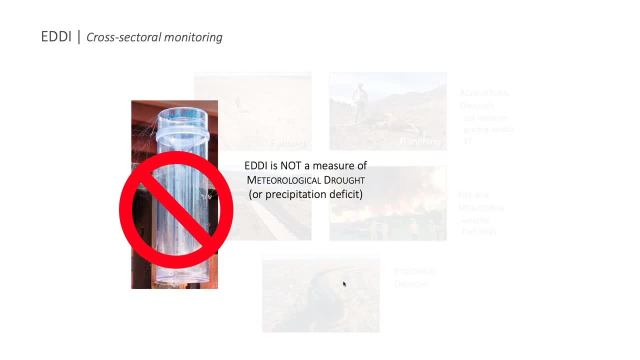 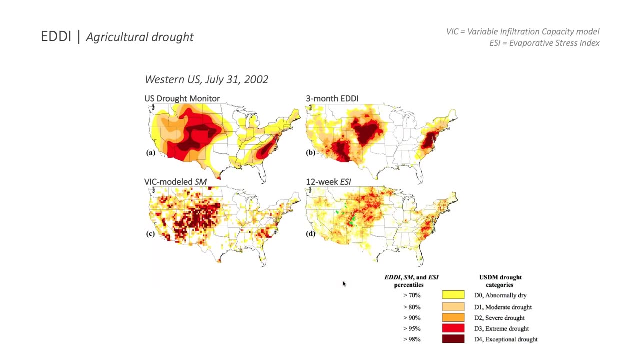 There's no precipitation input into eddy, For that you'd want to look at the standard precipitation index, standardized precipitation index. So just some maps to show how eddy looks at the agricultural drought. Here we see the eddy, which is this top right one. 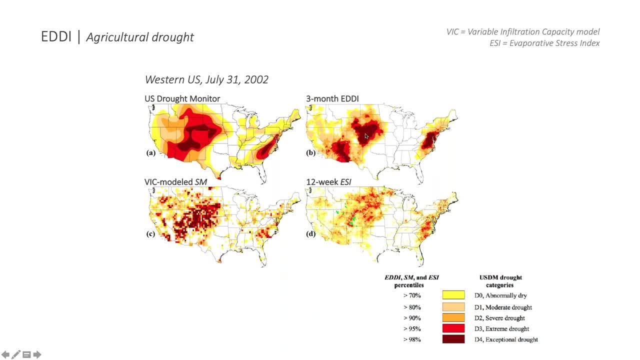 This is a three-month eddy- Really picks out the sort of two lobes of drought in the West that the USDM captures here as well, And it captures this eastern drought. This is in 2002.. You know it's offset to the north compared to the US Drought Monitor. 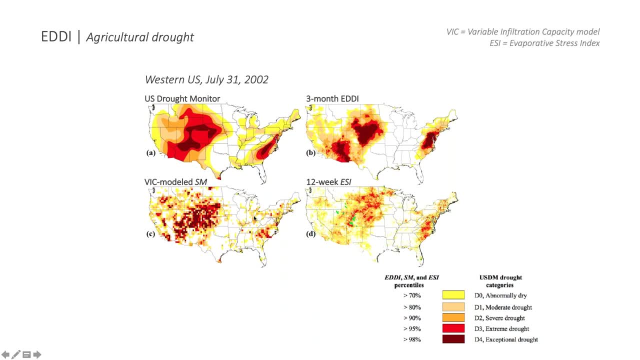 But all these maps are agricultural. These three maps are agricultural evaporative-related drought indices and they all look very similar. They don't look identical and we wouldn't want them to look identical because they all bring different information to the table. 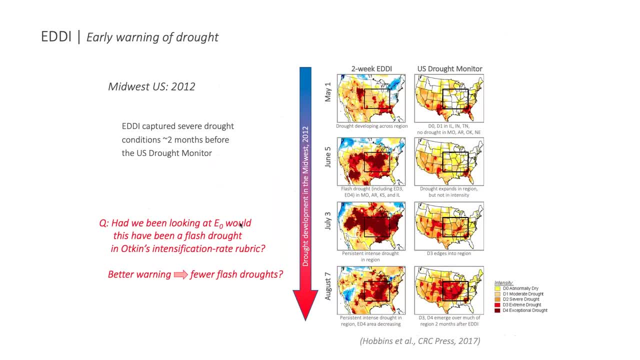 So it shows similar patterns. So it shows similar patterns to the US Drought Monitor and other agricultural-related metrics. So for early warning drought, this is one of the big selling points of eddy: It shows early warning of drought And this is not in the northeast, of course. 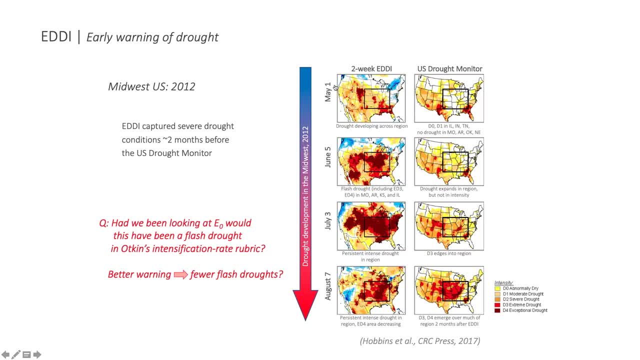 This is the Midwest drought And you can see the progression of this is two-week eddy from May through August during the drought, And you can see this rapid explosion of very dry conditions through July and then in August. So the first thing that we observed in the two-week eddy was the US Drought Monitor lagged behind significantly. 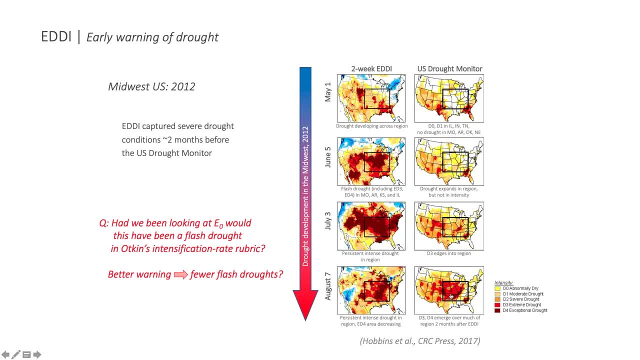 But the US Drought Monitor didn't have eddy as an input at this point because eddy hadn't been developed in 2012.. This is just retrospective, So it leaves the US Drought Monitor in identifying flash droughts in general. 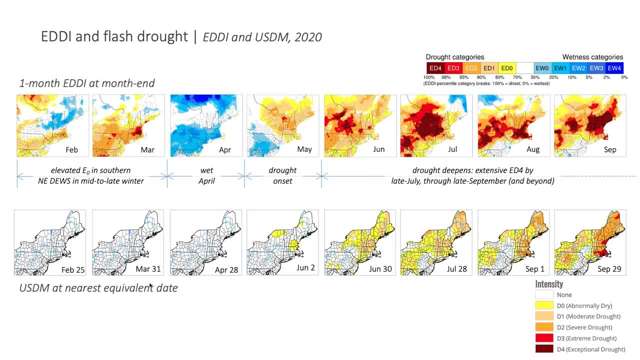 So what about the flash drought that occurred last year? We talked about this in a bit more detail last week, But here, if you look, this is sort of a film strip of eddy and the US Drought Monitor starting in February. 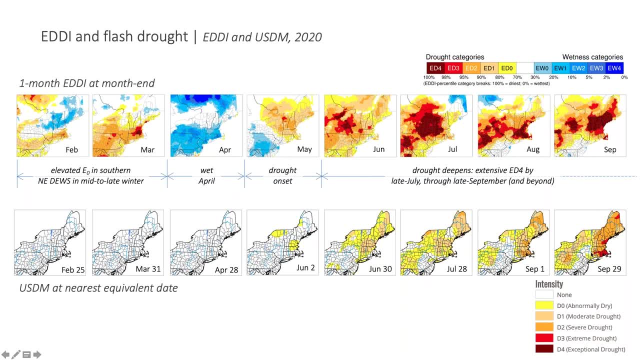 And then we looked at the last two weeks. And we looked at the last two weeks From February, over on the left, to September on the right of last year, 2020.. And you can see, the US Drought Monitor is perfectly neutral until about June, where you see abnormally dry conditions showing up. 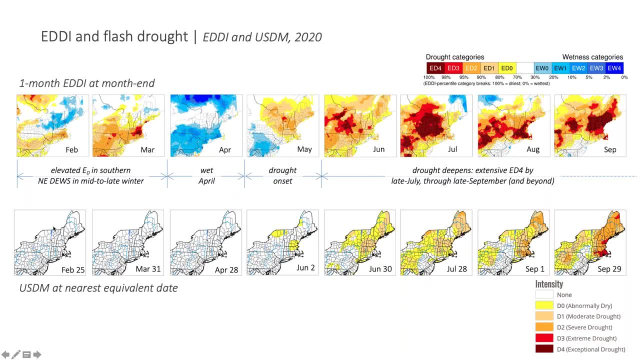 But what you see in eddy of the one month of the similar dates is you see elevated evaporative demand in southern New England and the southern Dews region in mid to late winter. Then you see a wet April And then you see drying onset again. 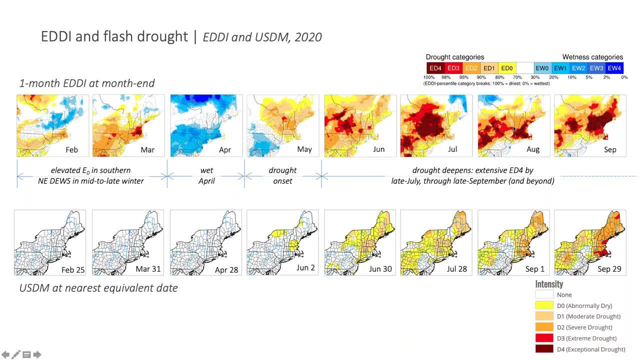 And it very rapidly deepens in July, August and September through ED4 all over the region And US Drought Monitor catches up slowly. I'm not saying that by any means. I'm not saying this replaces US Drought Monitor. 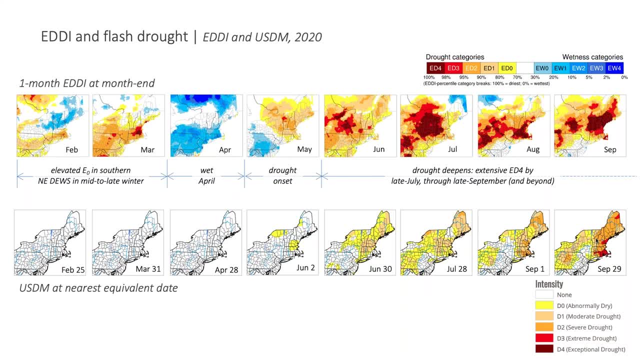 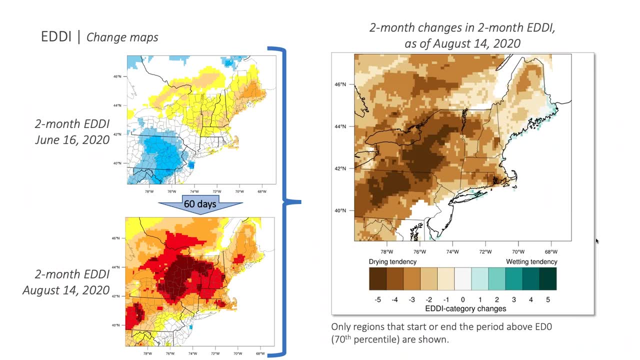 It's a leading indicator that is now being incorporated into the US Drought Monitor. So let's keep going. So onto how you can use eddy as a tool. One of the things that we've done is do these change maps. 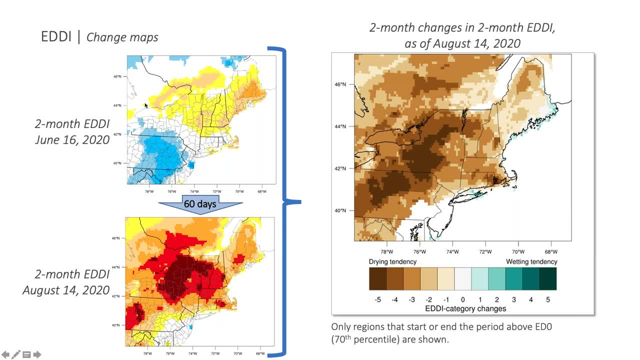 And you might have seen these in the US Drought Monitor, These change maps. This is between a two-month eddy timescale. over how much did that two-month eddy change? from June 16th to August 14th, That's a 60-day period. 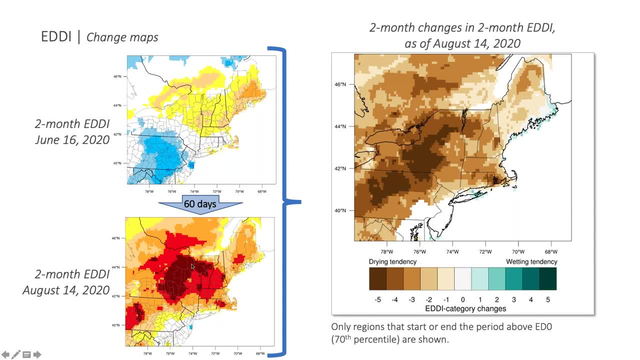 So this is a two-month eddy, changing over 60 days. Then this is that same flash drought period And you can see this very rapid. If you look at the change maps, you can see this very rapid intensification in central New York. 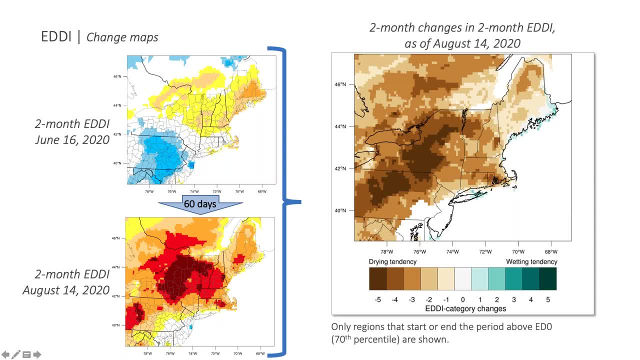 In Pennsylvania and over here in the Rhode Island, Massachusetts area And this shows a number of categories of eddy- that the drought deepened by drying tendency during that period. So this is a sort of an ongoing taking the pulse: How much is eddy changing? 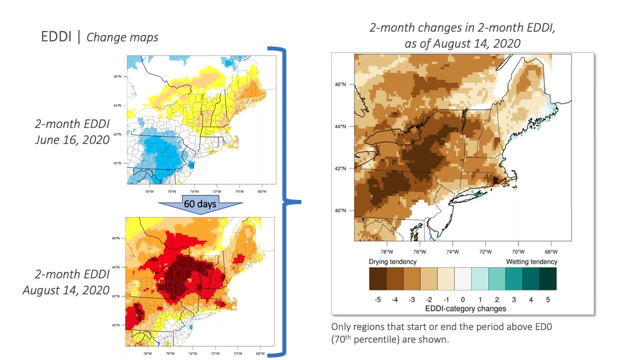 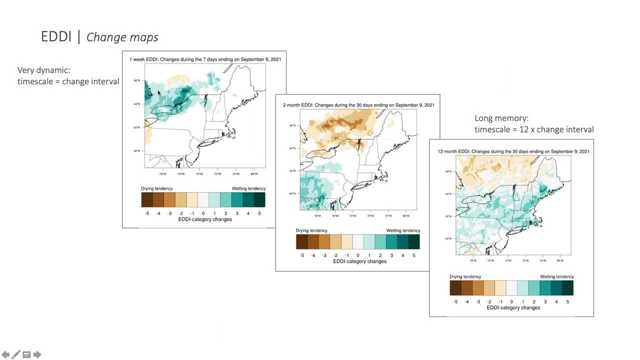 How much is the atmosphere drying over any specific period? And I produce these maps for a bunch of different timescales and a bunch of different change periods And it only shows those periods. It shows those periods that either start or end in drought. So, like I said, you can see these at. this is three maps for the same thing, the same date, September 9th, at a bunch of different timescales. 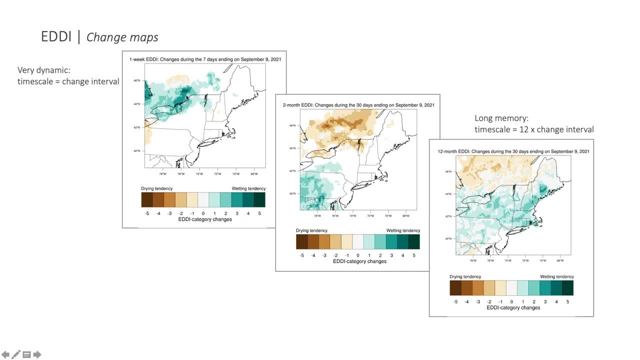 So here's a one-week eddy, which is sort of weather scale eddy. It only looks at the last seven days, And over here is a 12-month eddy. How does one-year eddy compare to last month's one-year eddy, for example? 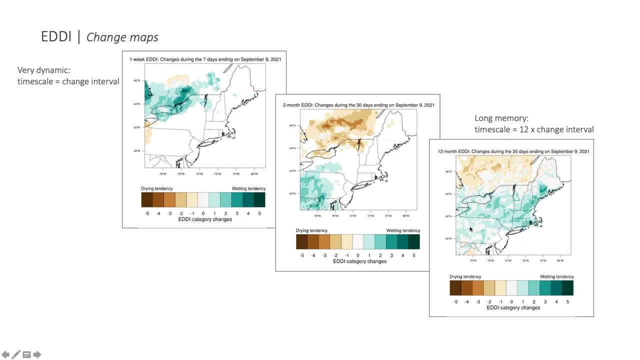 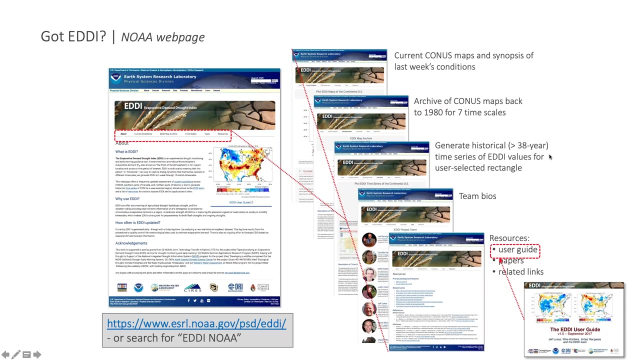 This is a long memory thing And you see a lot of wetting now compared to where you stood on September 9th 2020.. So these maps are all available on the website I will show you in a minute. So for general information about eddy, if you're interested in eddy, go to this NOAA webpage. 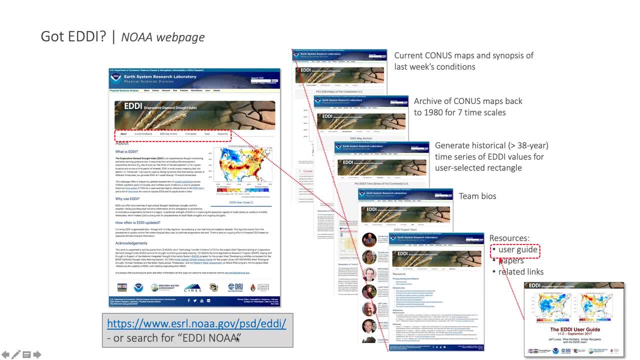 You can just Google eddy NOAA and it should take you there. Or you can email me and I'll point you there. And it's got current CONUS maps. It doesn't have a synopsis of last week's conditions. Instead, we've replaced it with those change maps. 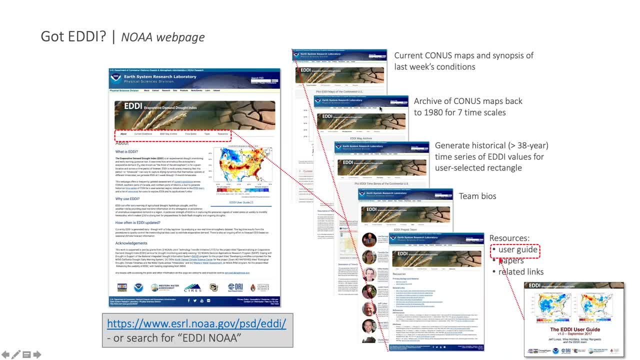 Which seem to get more play with stakeholders. It has an archive of CONUS maps back to 1980 for a bunch of different timescales. You can generate time series of eddies if you have a user-selected rectangle. That's on one of these other pages. 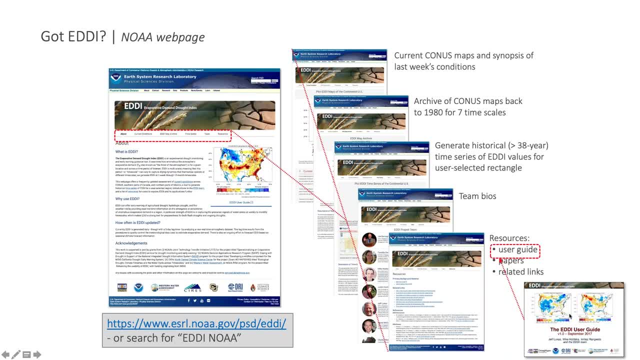 There's a bunch of team biographies And there's this very handy user guide that's available on the Resources tab. Jeff Lucas and the Western Water Assessment put this together And it's a very user-friendly step-by-step guide through what eddy is. 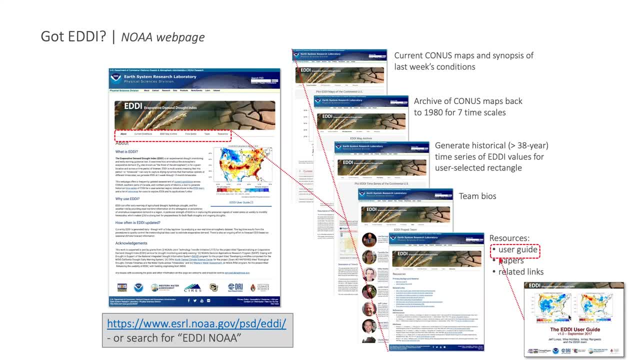 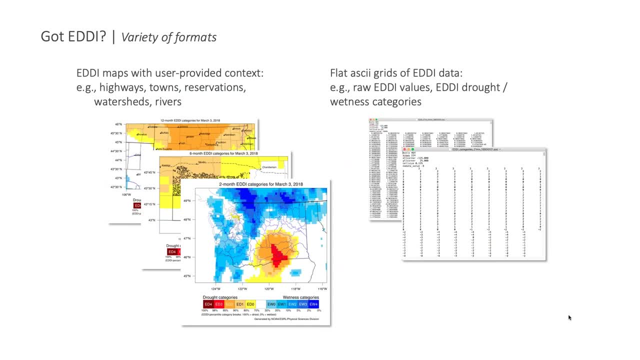 And how you can use it. More specifically, how you can get it from me. If you're interested in getting specific regions or formats or values added to the maps, I can do that for you. For example, here we have South Dakota. 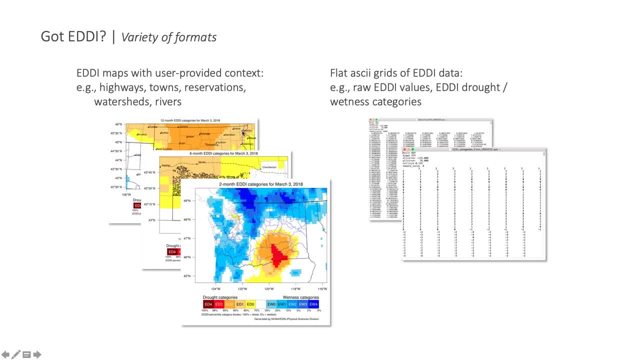 For some reason they wanted to have their towns and major highways shown on the map. The Rosebud Sioux here wanted to show the reservation boundaries on the map. Washington State wanted to show the. I think these are HUC 2s, HUC 8s, I think. 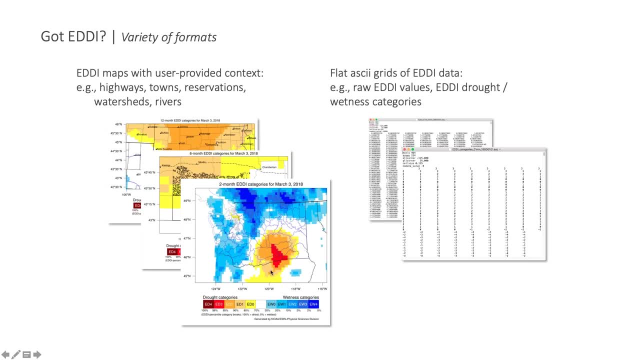 Or maybe HUC 6s Across Washington State on their map, Or you can just download the raw data, Either as in this example, as the actual eddy values, The standard normal ordnance of eddy Or the categories of that map. 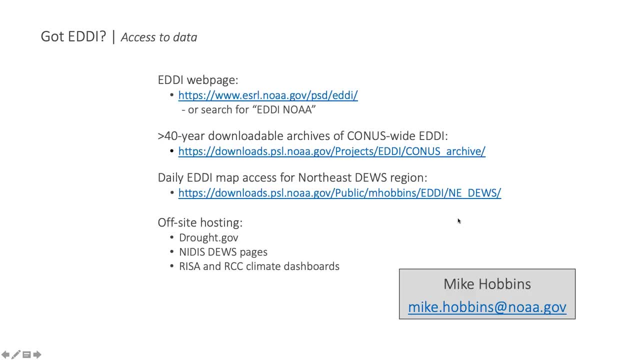 The categories that that converts to, And you can get them at these places. This is that web page I showed you earlier. Like I said, you can just search for eddy NOAA. You can get an over 40-year downloadable archive of CONUS-wide eddy. 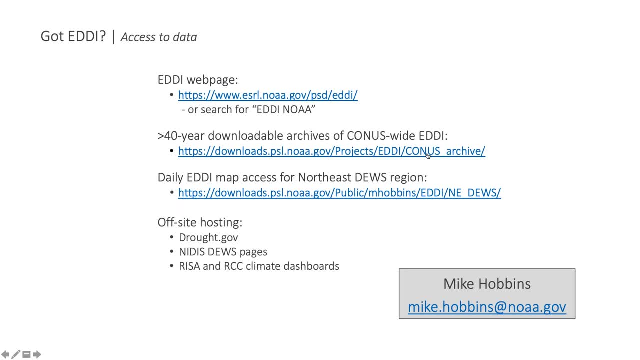 Maps or data At this website here Which you don't have to scribble down, I will email. You can email me and I'll send it all to you. Or you can get specific maps for the Northeastern Sioux region at this website here. 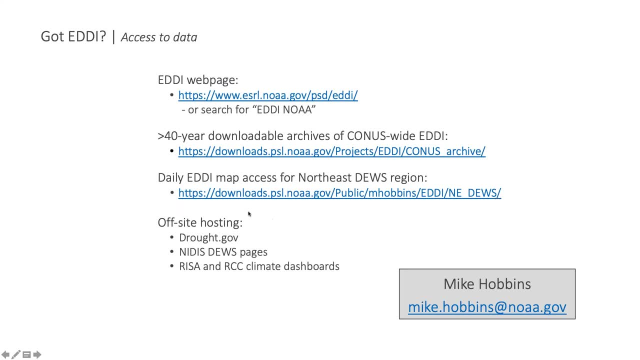 Again, I can pass these on to you. You can also find it on a bunch of different off NOAA sites Or NIDIS dues pages Or various climate dashboards. If all else fails, just email me MikeHobbins at NOAAgov. 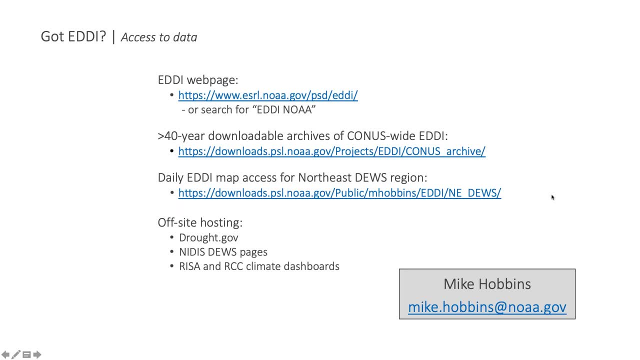 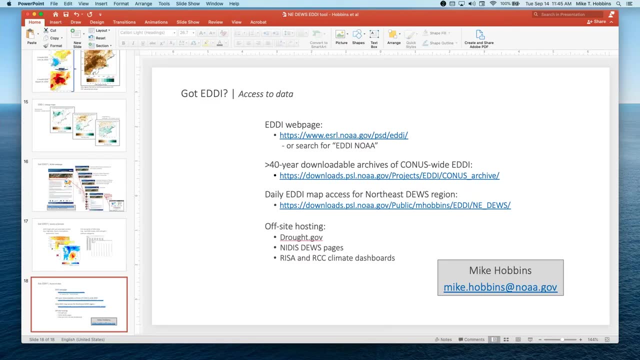 And I will point you in the right direction, And I think that's it. Thanks so much for listening. Thank you very much for that, Mike. As I mentioned before, we're going to hold all the questions Until after Imtiaz. 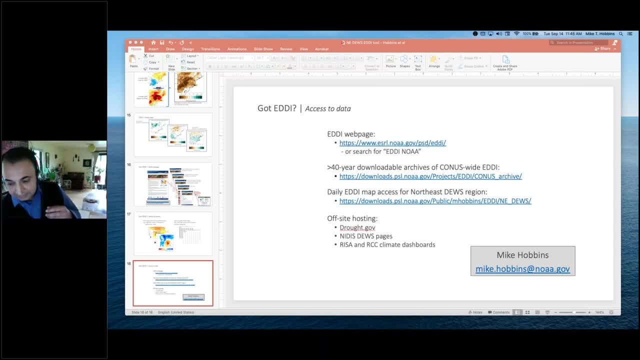 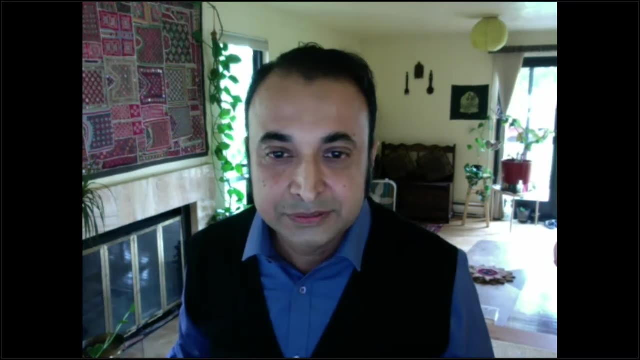 And then hopefully have a good Q&A and discussion. So I'm going to pass the baton here to Imtiaz. Well, great, Thank you, Dan, And greetings everyone. I'm just going to make sure to show my screen. 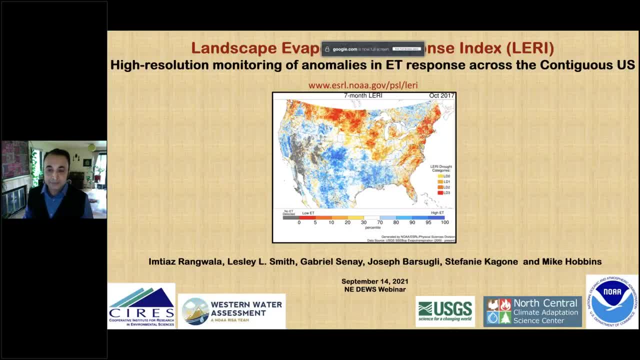 Hopefully you can see my screen and my slide in the presenter mode Looks good. Great Thanks, Dan. So I'm going to talk about two different web-based tools that Dan mentioned earlier. I'll start with the Landscape Evaporative Response Index. 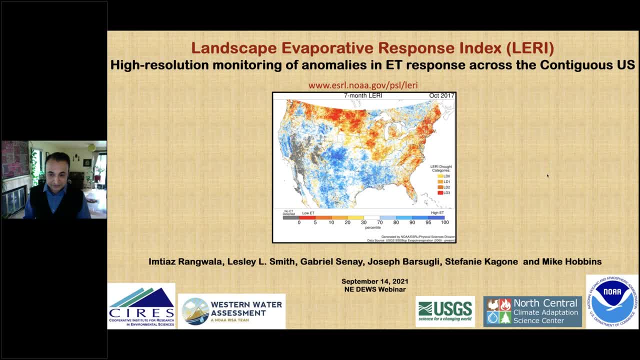 Which is kind of a newish drought index that our team created some time back. It was released in 2018.. It was a kind of multi-partner, multi-institute effort. I really want to recognize North Central Climate Adaptation Science Center for funding the project. 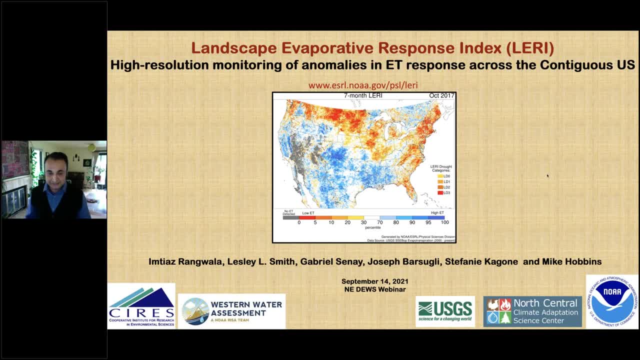 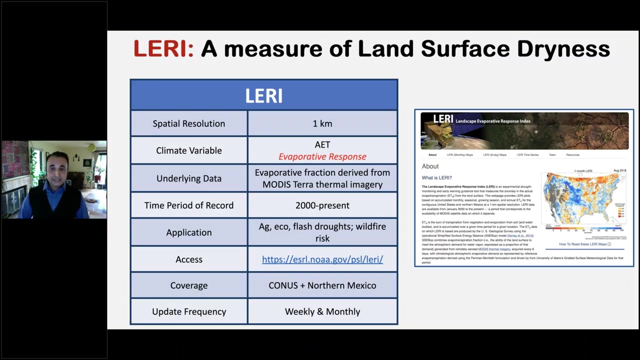 And NOAA's Physical Science Lab for providing the technical capacity and kind of the web platform to make this web tool available, And really want to recognize Leslie Smith, who was kind of the primary person to develop this tool. So what LERI is is essentially a measure of land surface dryness. 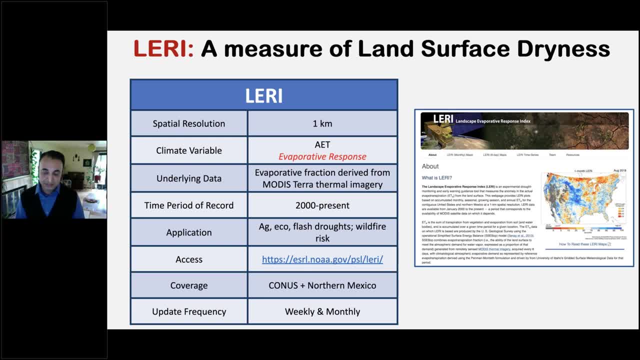 Mike talked about EDIT. It was the atmospheric dryness he was talking about, And so LERI really complements EDIT. We kind of call it its younger cousin, But in a very complimentary fashion. So what it's working with is evaporative response and not evaporative demand. 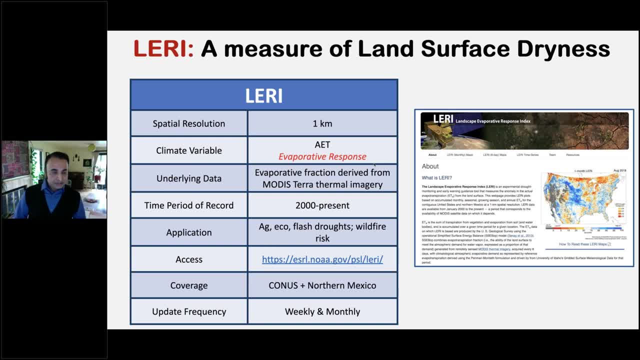 Dan mentioned in his talk that LERI is based on the underlying data. for LERI It comes from MODIS Terra Thermal Emittery, So mostly it's looking at the. So mostly it's looking at the land surface skin temperature and deriving the land surface evaporative response. 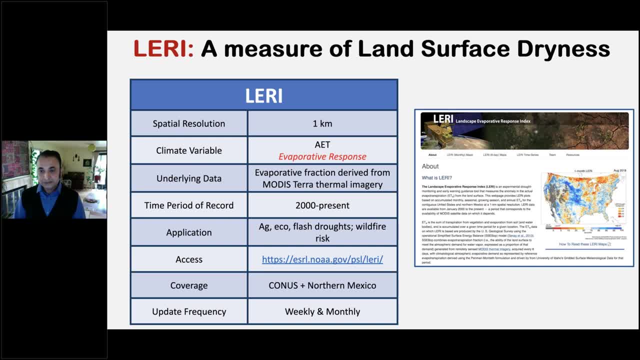 Essentially, what it's trying to estimate is the ability of land surface to do ET. So, based on its mathematical design, it's really that the measure of how moist or dry land surface is And, related to that, its ability to do ET- evaporative transpiration. 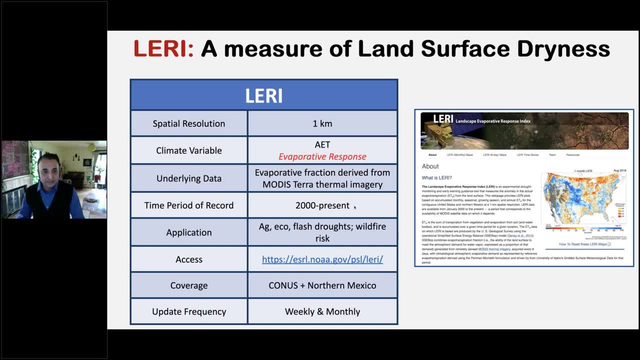 The time period of record that we have for LERI goes back to 2000.. So not as far back as EDIT, which is 1979.. Applications: almost all that EDIT does. should you know, LERI should provide some value for those applications. 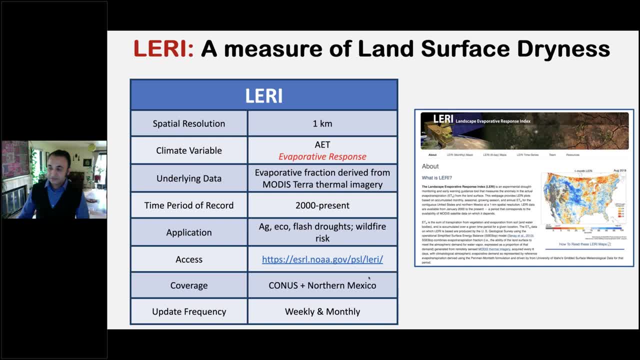 And I see that Sylvia has already put the link for LERI, The coverage for LERI, The area of LERI, The area of coverage covers Conus and northern Mexico And the update frequency for LERI during the growing season it's weekly. 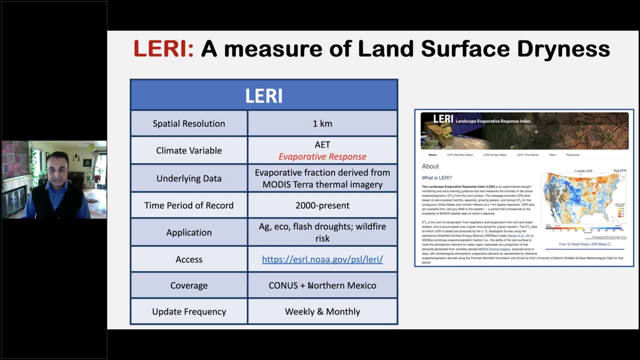 You have both weekly eight day assessment and monthly updates, But outside the growing season it's mostly monthly And again it's governed by the data available from MODIS, And so we get the best eight day data And that is kind of the rawest data that's used. 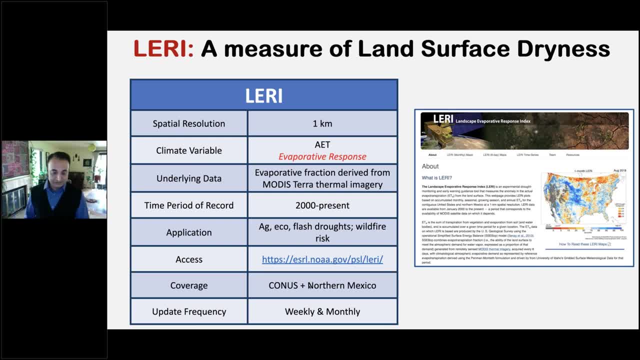 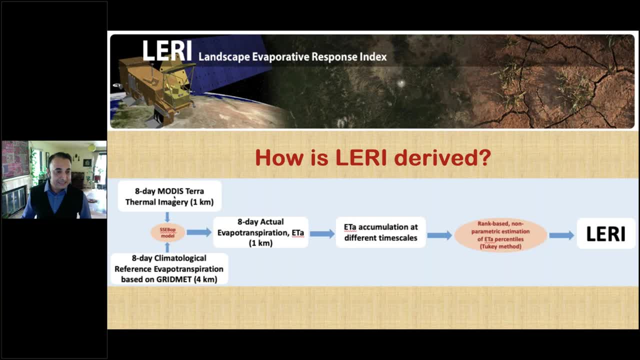 So that's really available at the weekly time scale And using that data we get the weekly and monthly products So quickly. how LERI is derived? We use the best eight day MODIS thermal imagery data which is available at one kilometer. 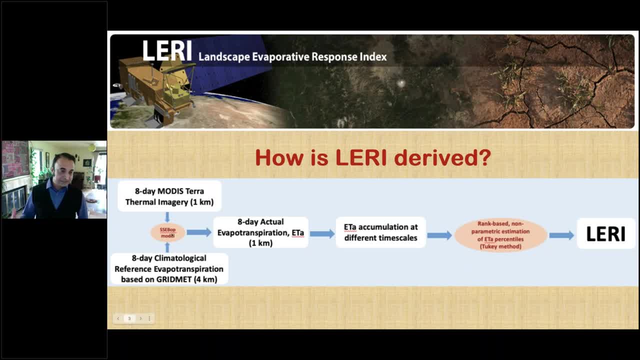 That goes into this CBOB model, which is a surface energy balance model that you know just calibrates that skin temperature into evaporative fraction, So which is based on how hot or cold the temperature is relative to a climatological value. 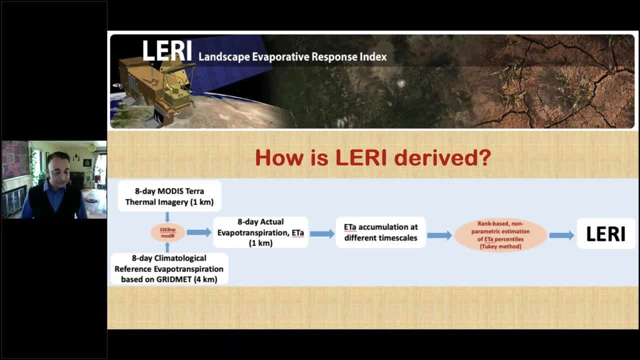 It estimates the ability of land surface to do ET or it's evaporative fraction, And that's kind of the primary estimation that's then used, that the product of that with a reference ET available from CREDMED, a climatological reference ET for that eight day period. 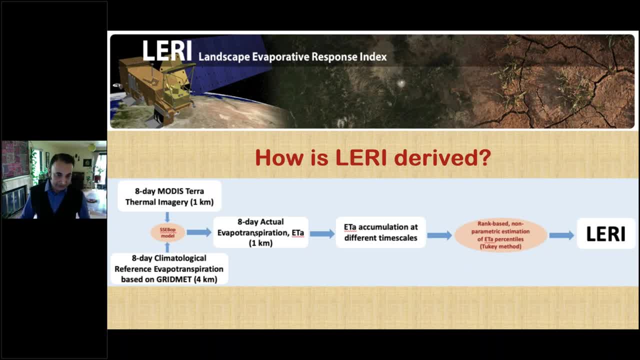 And gives us the actual eight day ET value And that eight day ET is then accumulated at different time scales from months to seasons, And that ET value, those ET data, is then taken through the rank based nonparametric method that we use for EDDIE. 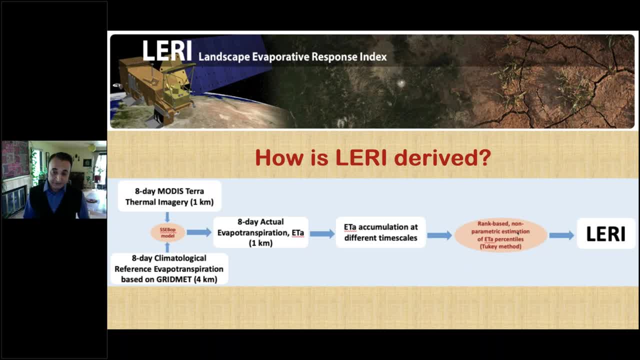 So Mike explained that in detail. The same exact method is used to derive LERI And I must say that because we had the skeleton for EDDIE as a web tool, it was very efficient for us to develop LERI web tool. 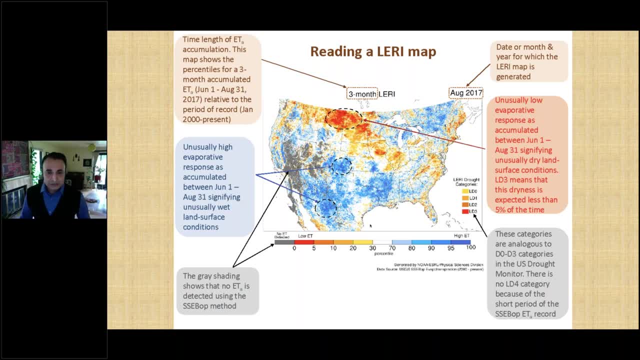 Apologies for this very busy slide, But all I wanted to show was it's like any other drought index And you can read LERI pretty easily in terms of The percentile categories of dryness and wetness. Dryness shown by the warm color shows low ET. 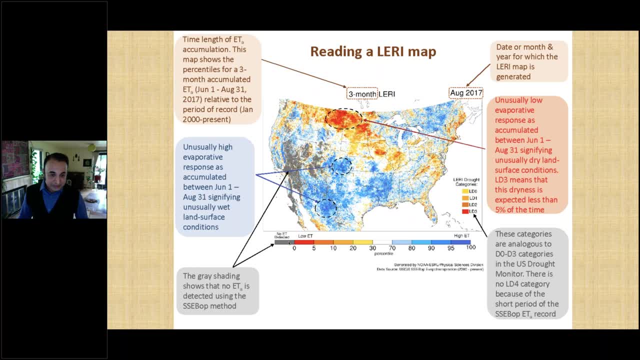 Wetness shows high ET. We also have this gray area here in LERI And that's if you're not detecting any measurable ET using our methodology, that goes into gray And usually you'll see these very dry places on the continent show up gray. 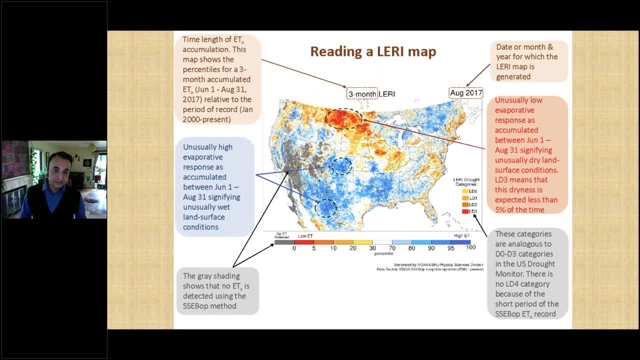 But the gray expands and contracts depending on a LERI map, And that kind of shows you how sometimes very extreme droughts move across the region, But mostly it's in this part of the very dry region of the continent. Another piece to note here is we do provide drought categories using LERI, as Mike showed for EDDIE. 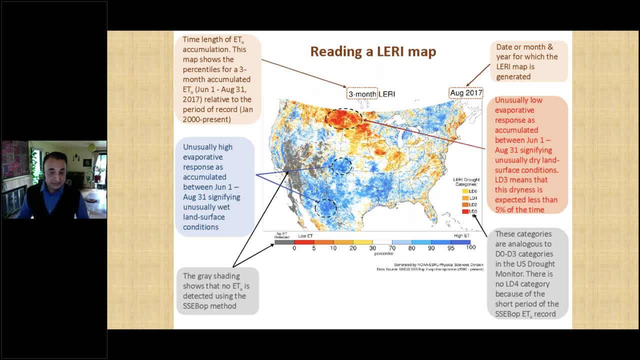 We do not have LD4 here, So we have LD0 to LD3, but no LD4. Again, from a short period of record we cannot get into the two percentile category. So we get to extreme drought but not to exceptional drought in the LERI world. 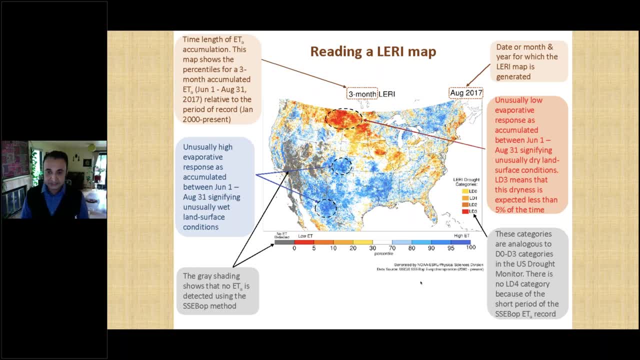 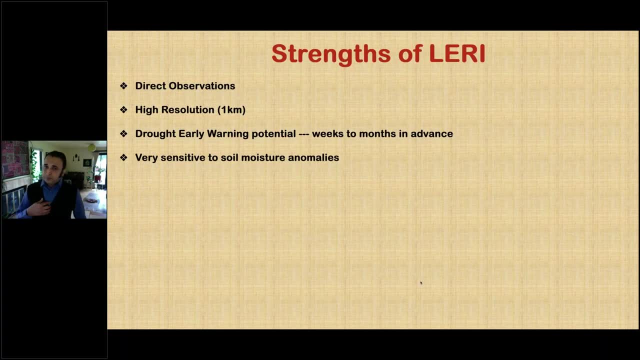 Yeah, I think everything else is pretty straightforward. if you are used to using other indices, I'll just keep moving. I just want to point to some strengths of LERI. I think the biggest strength is it's the direct observation from the satellite at a very high resolution. 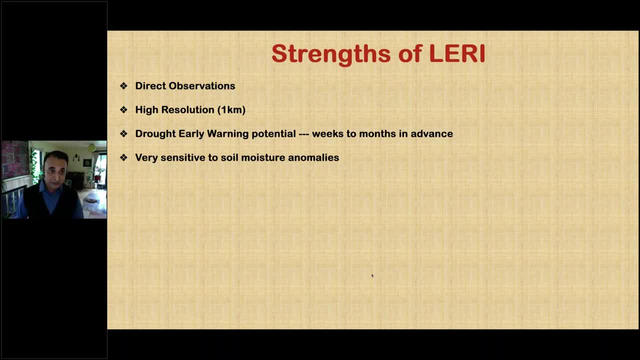 So I mean you cannot beat direct observation with any model. But, as I just pointed out, you know, observations have their own issues And we believe, although the research is still undergoing, that it has early warning potential from weeks to months in advance. 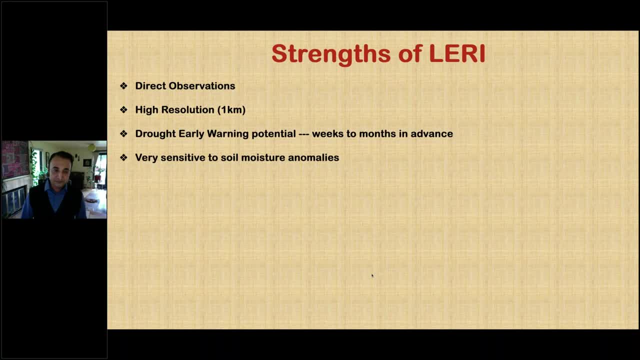 And, as I said earlier, it's pretty sensitive. It should be, in theory, very sensitive to soil, Very sensitive to soil moisture anomalies, And I'll show you some evidence of that shortly. I should also talk about some potential limitation. I mentioned the short period of record. 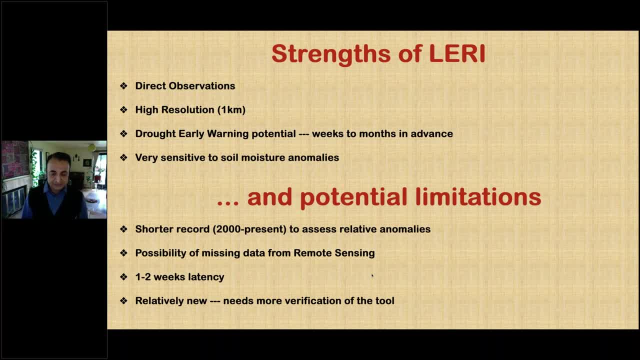 It could be an issue, especially in terms of assessing these relative anomalies in terms of how extreme the situation is currently. The remote sensing, the issue of cloud cover and other missing data issues show up. That definitely adds to The problem of missing data. 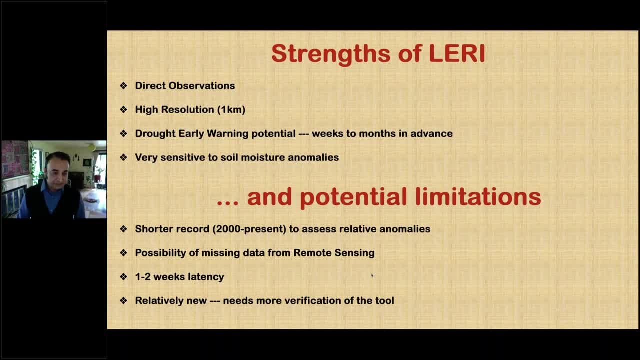 Yeah, sometimes the issue of latency is greater in LERI as compared to EDDIE, for example. So usually it's one to two weeks in a good case scenario that we don't have the newest data, But it could be something more than that. 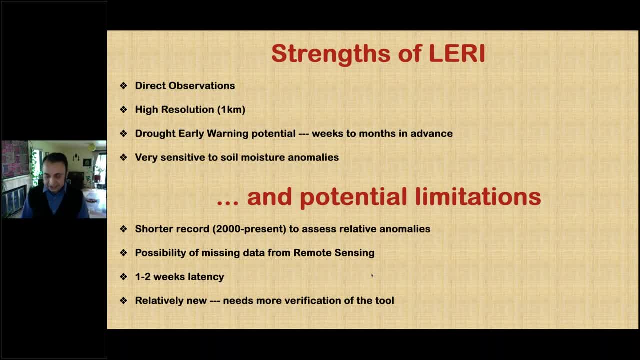 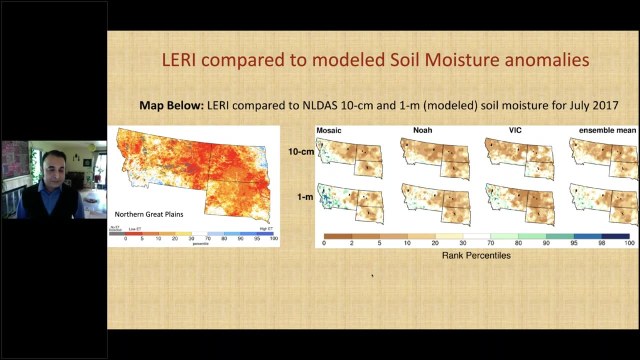 And because LERI is relatively new, we're still kind of looking at the tool very fine. It's ability to do drought, early warning and other added value. So yeah, as I said earlier LERI, we expect it to be sensitive to soil moisture anomalies. 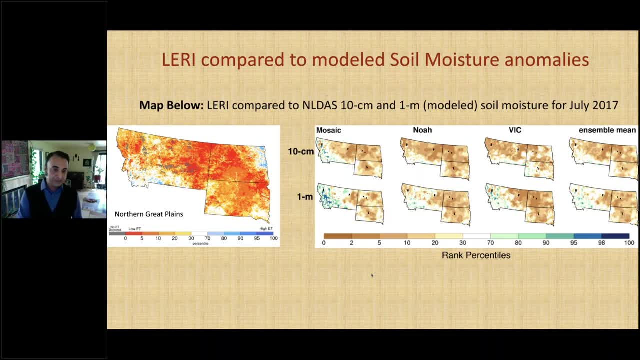 And here what I'm showing you for the Northern Great Plains region: a comparison of LERI, the different model soil moisture data set. And what I'm showing here is the NLTS forest Soil moisture modeling model products from different land surface models at top 10 centimeter and one meter. 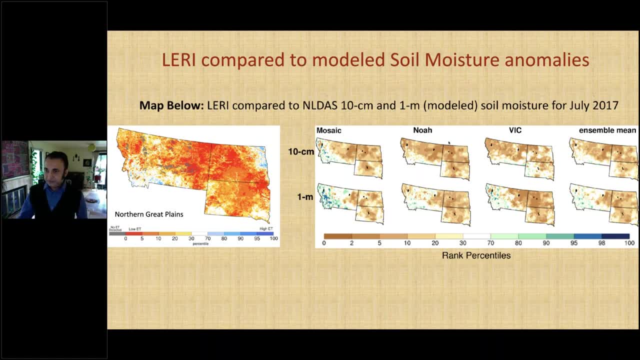 For July 2017, which was kind of a major drought episode in the region. it was a billion dollar disaster And again it's basically- this is just a point- that LERI kind of collaborates very well with these different soil moisture products. 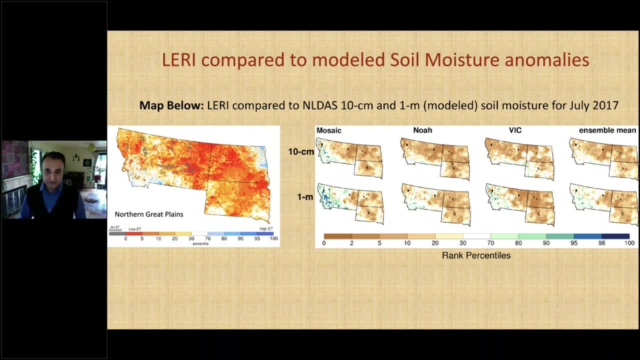 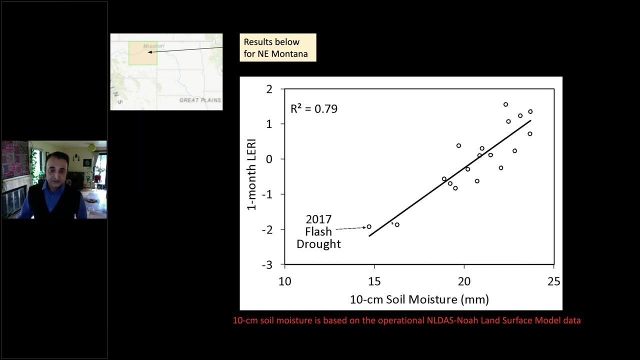 Interestingly, you know, even though these models are forced by the same atmospheric forcing, they show quite a bit of difference in terms of their spatial modeling of soil moisture. There's another way to look at it, Just comparing July soil moisture values with LERI. 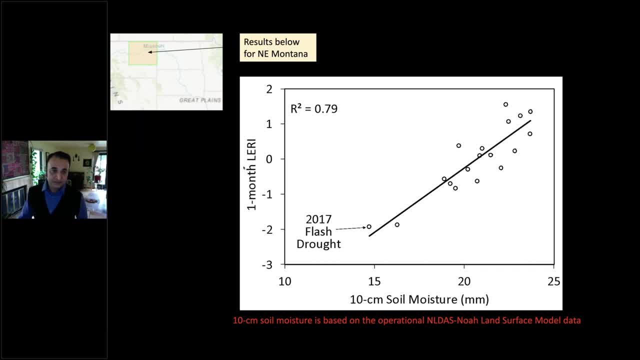 So just one month, July, soil moisture top 10.. And then July: soil moisture top 10 centimeter, compared to one month LERI. And the soil moisture comes from one of those land surface models I showed earlier. This is the NLTS NOAA. 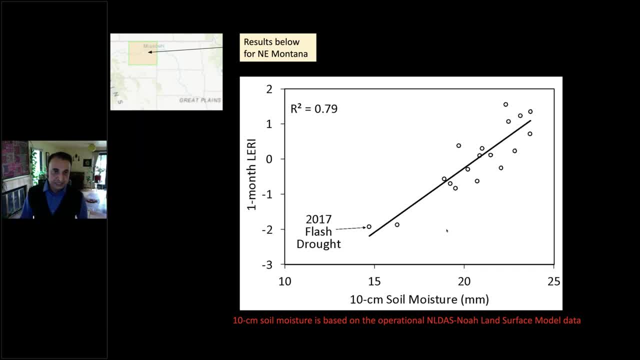 And just to point out again, this is the high correlation between the two. Of course the question here is, you know, are the model soil moisture good enough? But these kind of corroborations do help. to point to, LERI has some ability to sense land surface moisture conditions. 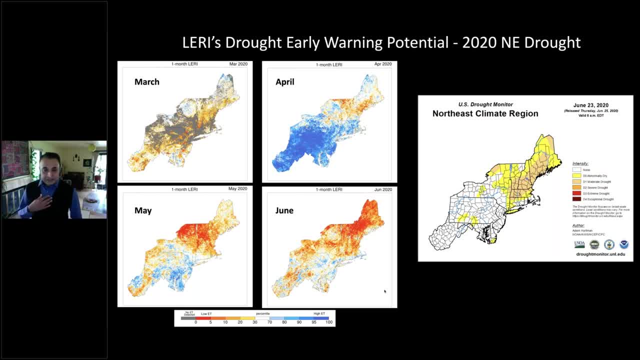 So I want to quickly get into talking about LERI's drought only running potential with regards to the recent 2020 drought, And were there signals that were of value, And what I'm showing you here are one month LERI values, from March through June. 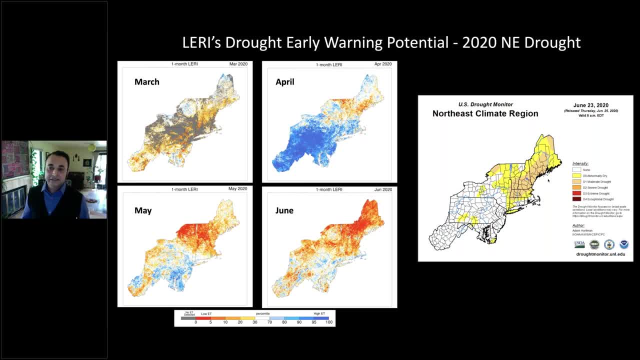 Comparing that to the June 23 USDM map. And this June 23 was the first Date on which we actually saw any D1 categories on the USDM map. Before that you only had D0. So if you look at the one month LERI, you do see signs of drying as early as March in parts of New England and other parts of the Northeast. 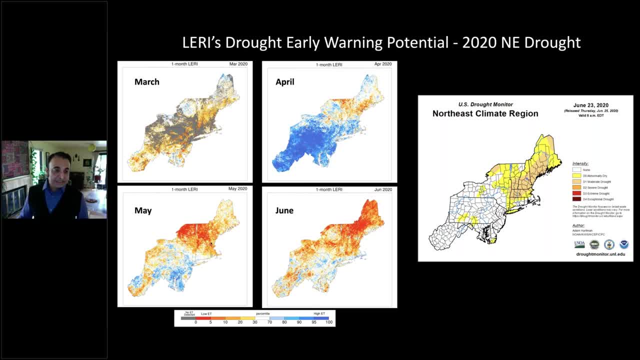 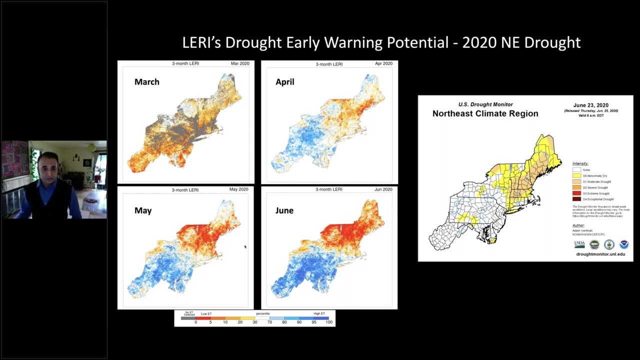 And they kind of persisted into April but really intensified in May, into June, And so Just looking at this one month LERI maps, one can see there was, There were signals of dryness appearing, you know, weeks to months ahead of perhaps when the impacts were started being felt. 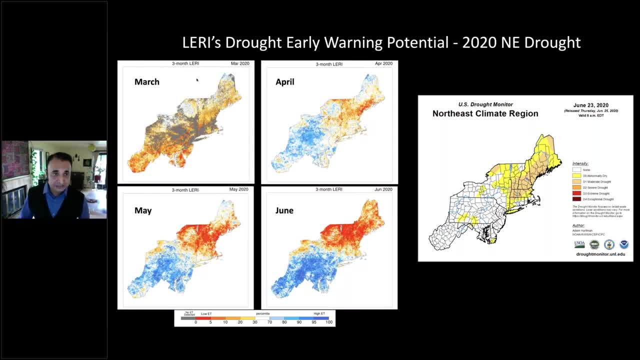 So the same kind of map, But now I'm showing three months LERI and just pointing that perhaps there is maybe a little more signal here in terms of Persistence of drought, especially in the region where, ultimately, the USDM started to show a lot of stress. 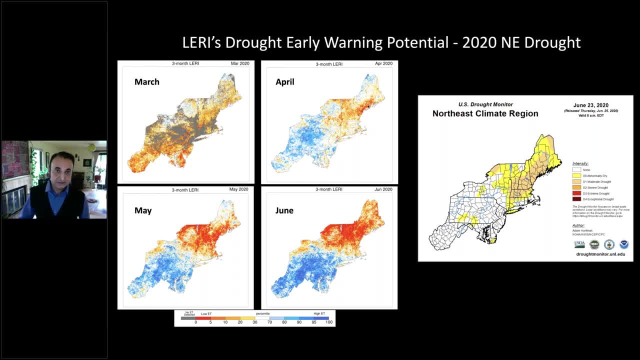 Again, maybe as early as April. we were able to see a lot of extreme conditions from LERI's perspective developing in April but really intensifying into May. The one thing I wanted to point out was this region in northern Vermont, And I also saw in Eddie maps that Mike showed earlier. 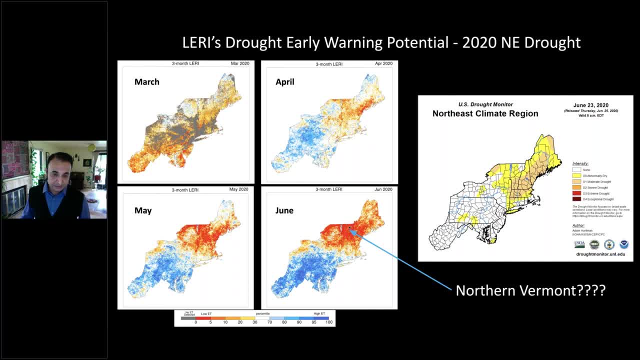 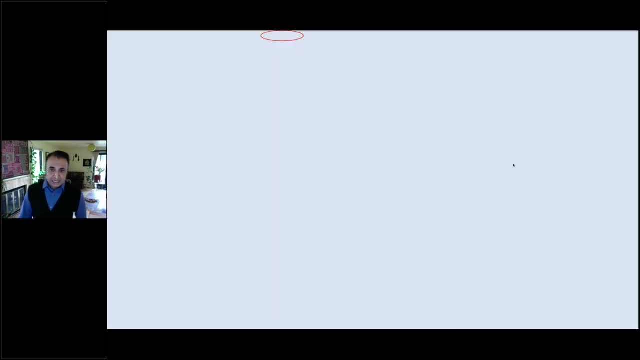 A lot of dryness Showed by at least these two indices, but not really captured here in the USDM, And I'll get back to that earlier. but just kind of curious why that place was getting mixed in kind of a big way. 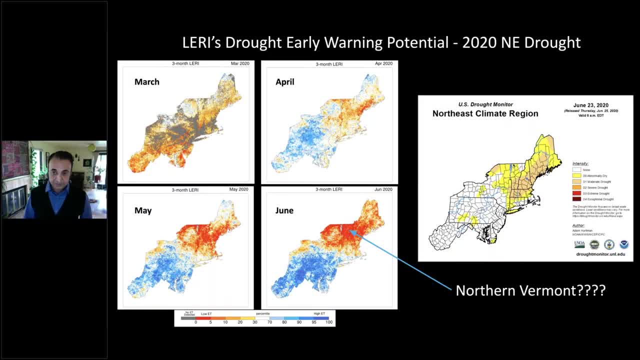 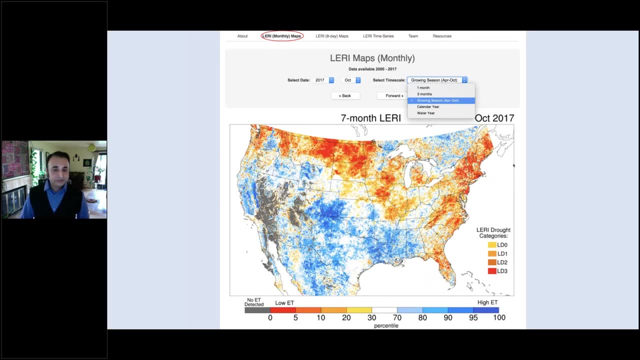 And was it a problem with LERI Eddie, or was it something that, because of the remoteness of the location, that did not get captured in kind of the assessment in USDM? So I'll quickly talk about some of the utilities on the web tool. 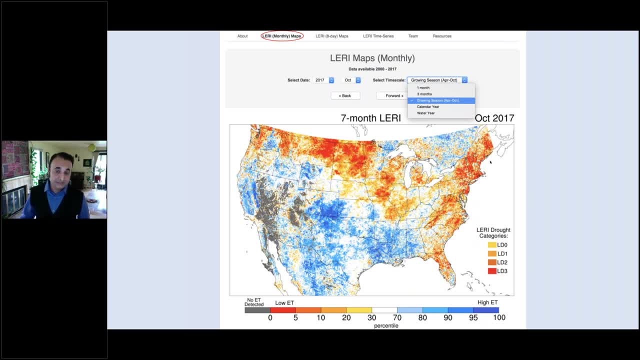 You can, as with Eddie, you can do monthly maps With Eddie, with LERI, and these monthly maps are available at one month or three months time scales. You also can get maps for growing season calendar and water year. 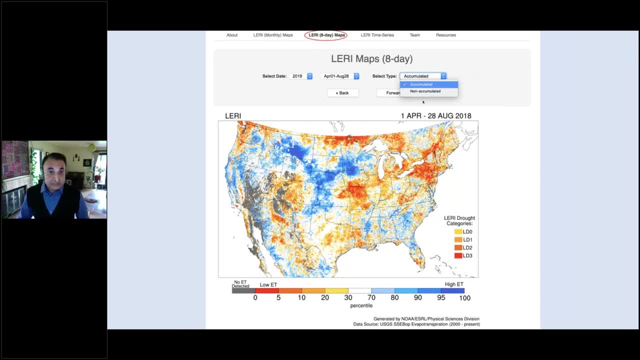 Okay, During the growing season we also have the ability to get eight-day maps, And these you can do it accumulated, starting from April 1st all the way to the end of October, Or you can do non-accumulated, so you can just get eight-day maps for LERI. 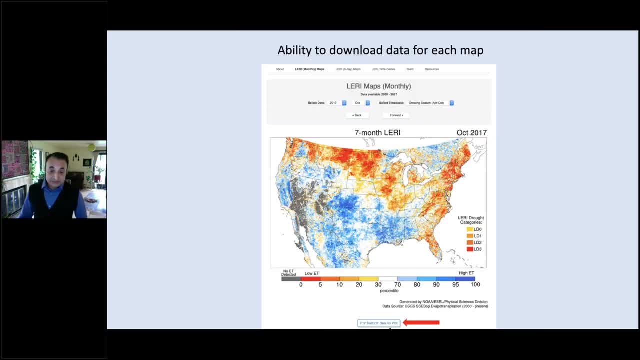 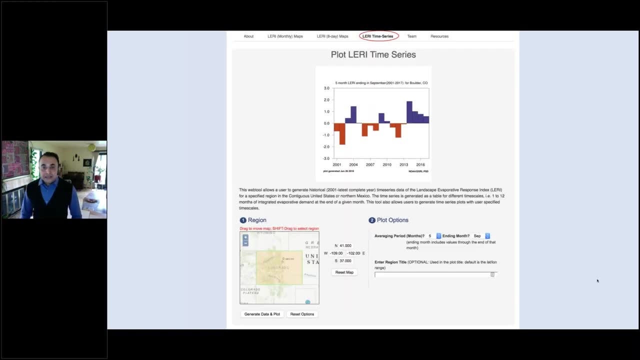 And for any map that you can plot, you can download the data as NetCDF. Okay, Thank you. And lastly, LERI also provides you the ability to do time series, So you can select a rectangular box anywhere for the region that LERI is available. 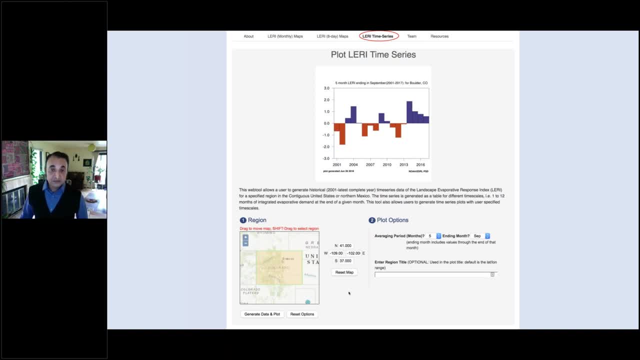 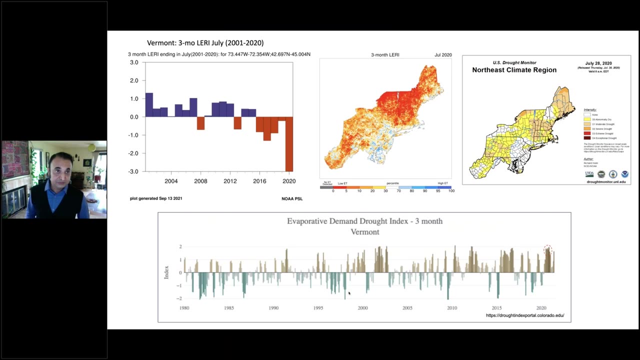 That's CONUS and Northern Mexico- And plot. So these are only monthly data, So you can plot, you know, integrate different months and plot the time series, And so what I've done here for you is plotted. I've plotted a three-month LERI, ending in July, for Vermont. 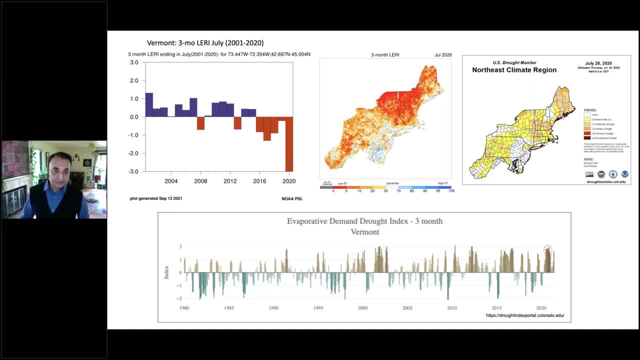 And what you will see is a pretty remarkable value for 2020 for Vermont, almost getting to negative three standard variations. So I'm just showing, at least from LERI's perspective, extreme dry conditions in July, Again shown here in the map. 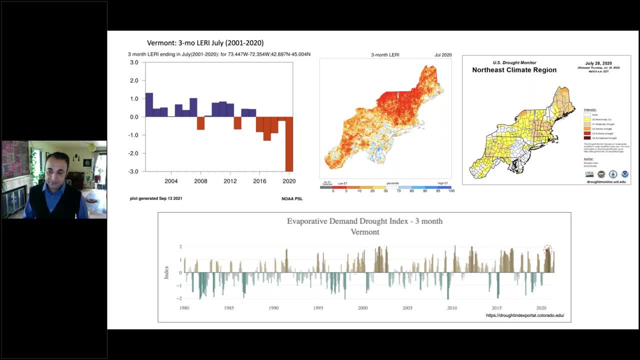 And I've just plotted Eddie down here showing you around. those times starting in July, Things are pretty high. So if our demand was very high, our response was very low. Again, it doesn't show up that strongly on the USDM map. 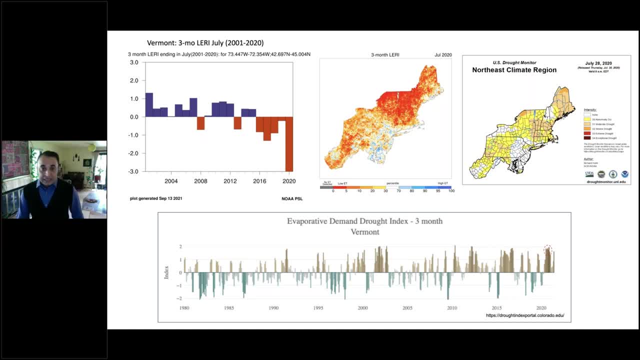 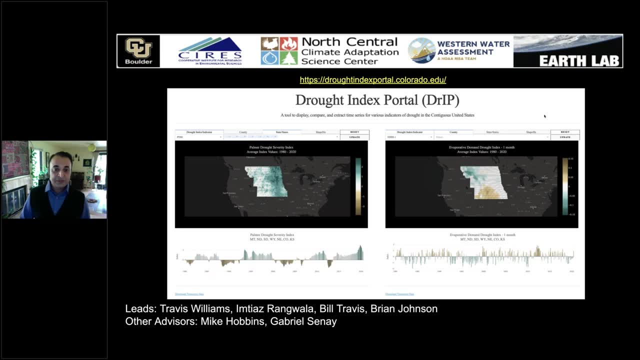 So, yeah, something to ponder about. I'll change gears quickly and talk about for the next five minutes this other tool we have called the Drought Index Portal, Again a multi-institute, multi-partner effort. I wanted to acknowledge funding from Western Water Assessment and North Central CASP. 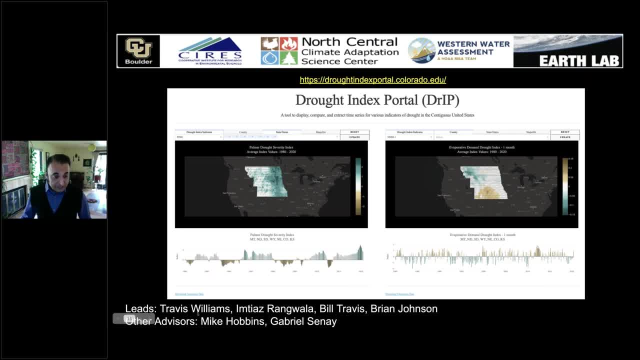 I also want to acknowledge Travis Williams, who was again kind of the main person behind developing this project and advised by many other folks. So I think I must mention that the strength of Drought Index Portal is, you know, just very efficiently produced data sets, especially time series data sets. 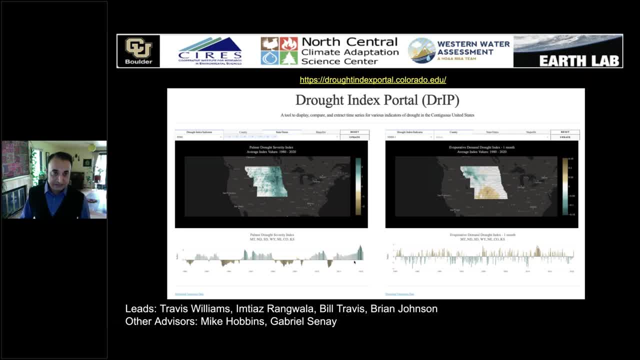 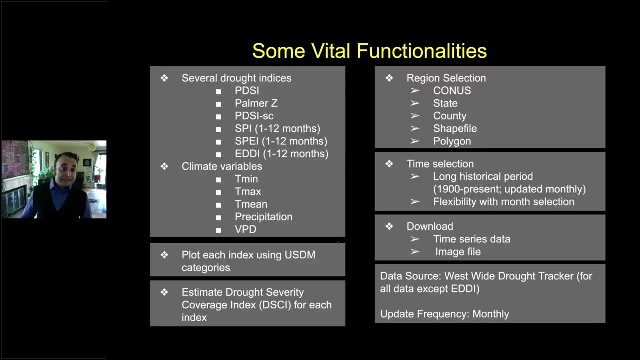 Long time series data sets for different indices and ability to compare across four different regions. So a lot of flexibility in selecting a region and getting you a long time series of these data sets. So different indices: as part of the portal include all the polymer indices: SPI, SPEI and EDDI. 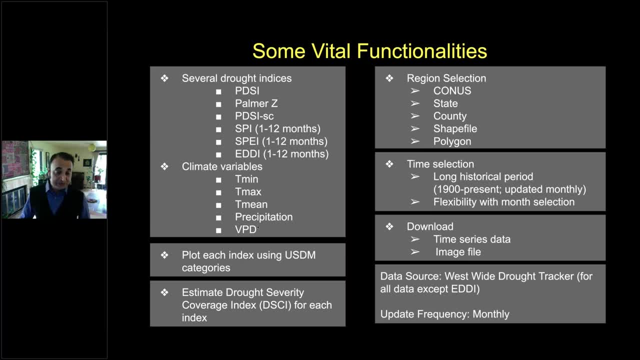 Also has some of these important climate variables that you can quickly download Using DRIP, So Drought Index Portal, short for DRIP. I know there are other DRIPs out there, So this is our DRIP. Let me get to the regional selection. 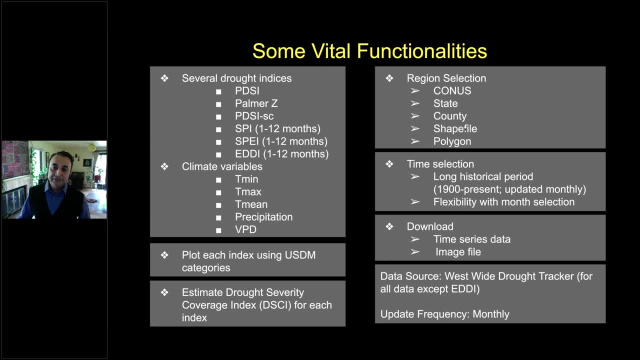 It's just pretty flexible and nimble in selecting different regions, So you can select state and county very quickly. You can also do polygons- user-defined polygons- And then it has a shapefile option. You can insert your shapefile and it will extract data for that. 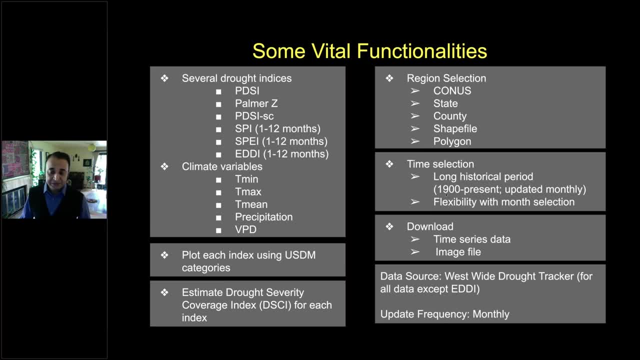 Also very flexible in terms of time selections and doing particularly these time series and mapping, But mapping is not as cool as it's in the climate engine tool And one of the main purposes for this was to make sure that we were able to do a lot of things. 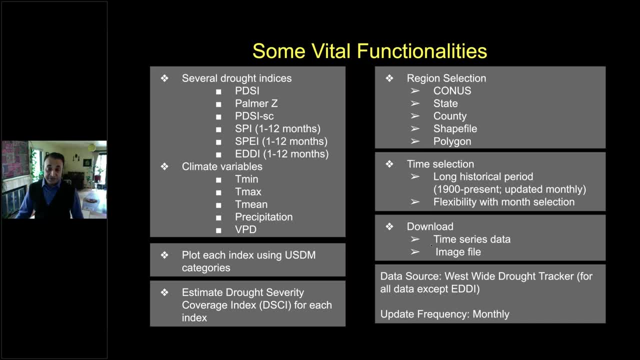 But one of the main purposes for this was to help with research, And so yeah, I mean, the ability to download time series data is facilitated here. I just want to mention the main primary data source comes from the Westwide Drought Tracker. 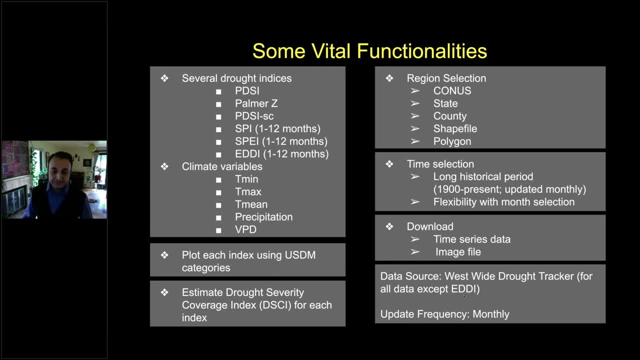 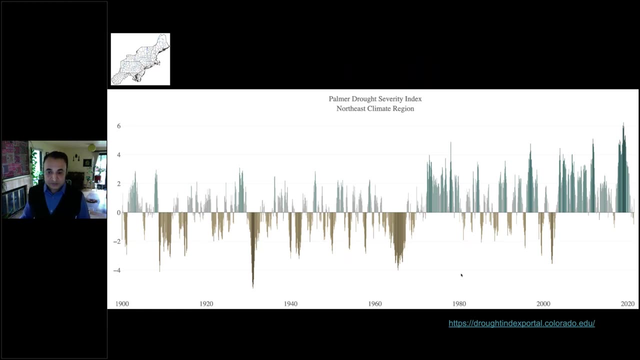 That's Desert Research Institute, except for EDDI data that comes from the NOAA site that Mike talked about And the update of all these data sets on a monthly time scale. So just a quick glimpse into what you can produce. And you can produce these graphs, these long-time series. 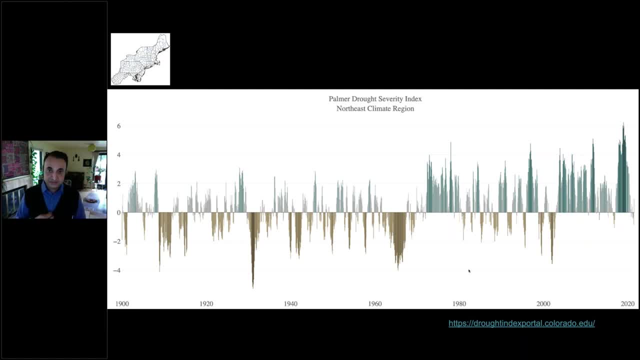 And here I'm showing Palmer Drought Severely Index for the Northeast RCC region. Again, a long perspective of drought really helps, And so it can put into perspective where our current drought is in context of some very historical drought. Palmer Drought is very sensitive to long-term trends in precipitation. 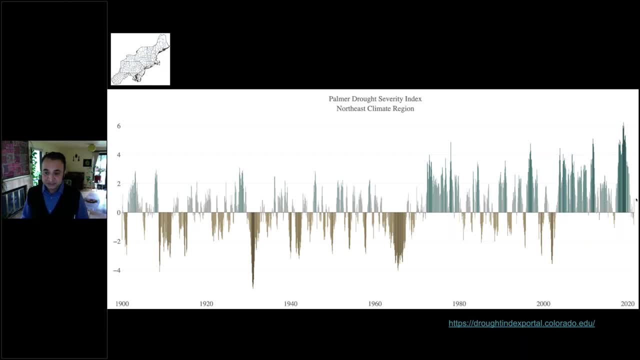 And you can kind of see it here that in the Northeast region it kind of shows that wetting trend and less of these extreme droughts persisting. Again from the lenses of Palmer Drought Severely Index. Same thing I could do with any other indices available. 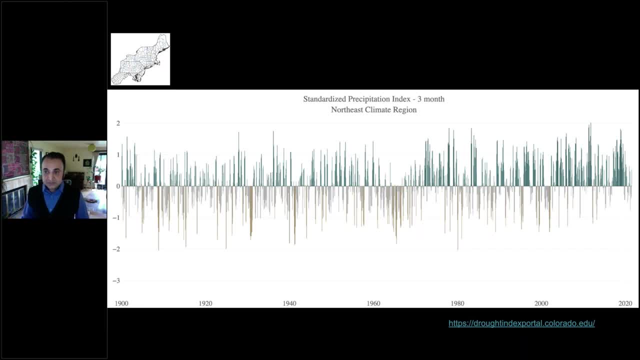 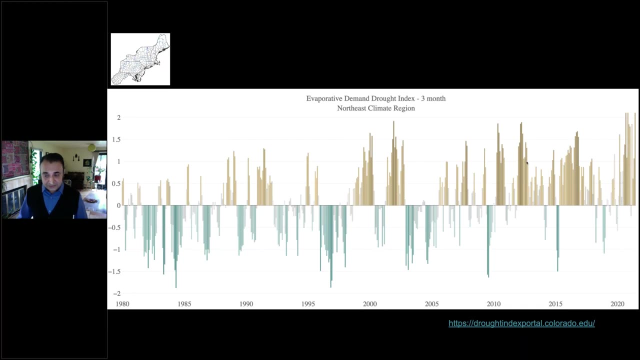 Here I'm showing a three-month SPI, Kind of a similar message: more green than brown, which is dry, Again showing a wetting trend in the region. On the other hand, if you look at the Rapid Demand Drought Index, you see kind of a different trend. 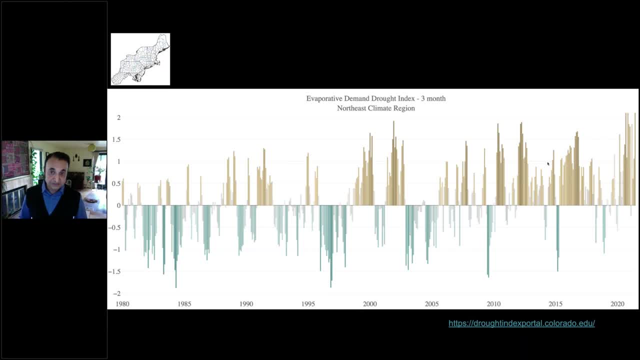 And we're really starting to see more, as it's getting wetter, the temperatures are also rising And that's in part- I think, maybe in the main part- contributing to the increase in the rapid demand And you kind of see it in the eddy trend, which is like more positive, more dry. 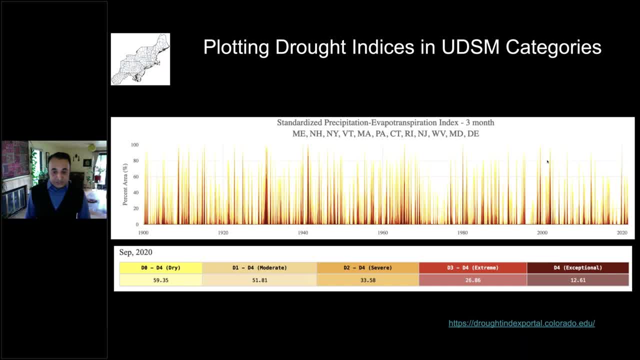 Another thing, very cool thing you can do: You can produce, plot these time series in the USDM categories. You can take any of the drought indices and plot them in USDM categories And not only stop at 2000,, where the USDM stop would go all the way to 1900. 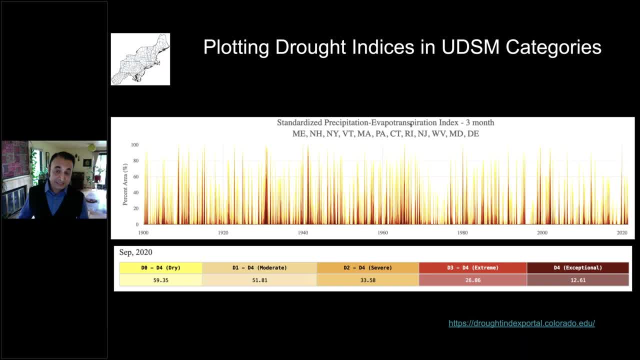 So here I've taken three-month SPEI and just plotted in the USDM categories using the categories recommendation that USDM provides on its website. You can also quantify for a particular month, you know area in different drought categories, And so that's just again very efficient way to quantify that kind of information. 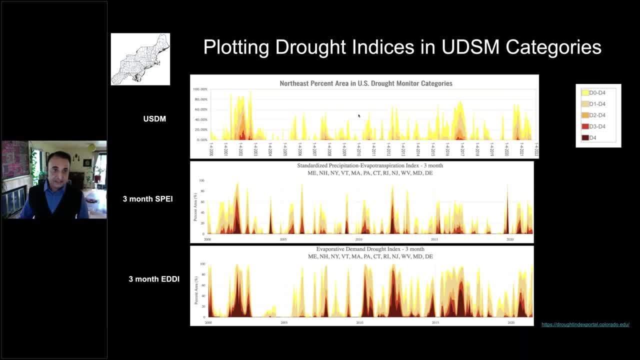 Here I'm showing, comparing this for the Northeast region, USDM and other drought indices for the same period. And this is another cool way to compare. you know USDM and these different drought indices, How they look like in kind of a USDM space or colors. 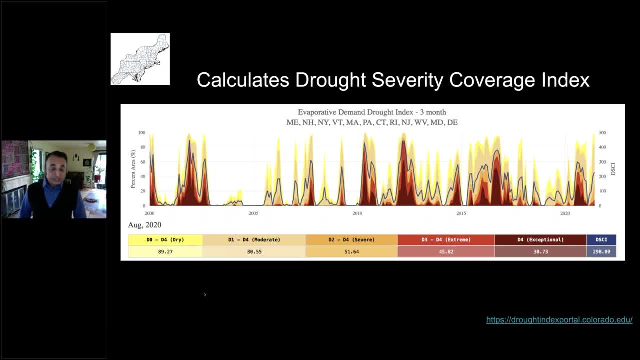 Or you can also do a calculation of drought severity coverage index. Again, some may really find it useful, But again, it's the product. It's kind of the integration of how it works, The integration of how much areas in drought and how extreme the drought is. 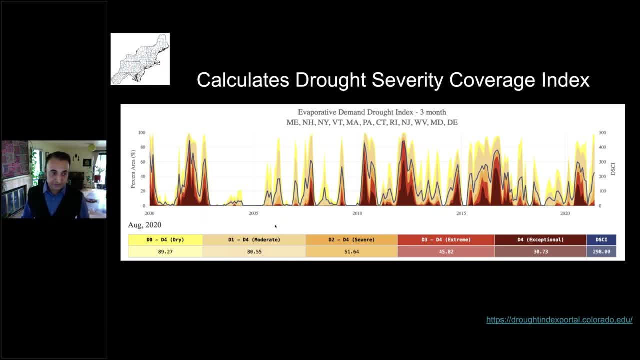 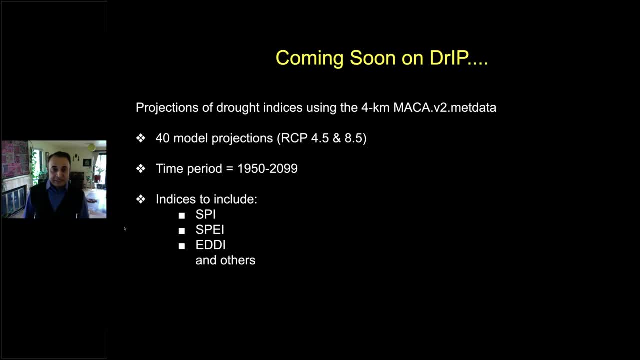 And again very quick quantification of that metric for any particular month that you're interested in. And I'll end with this specific information that very soon, on DRIP, will also try to include ability for the user to kind of get the data projections of these different drought indices. 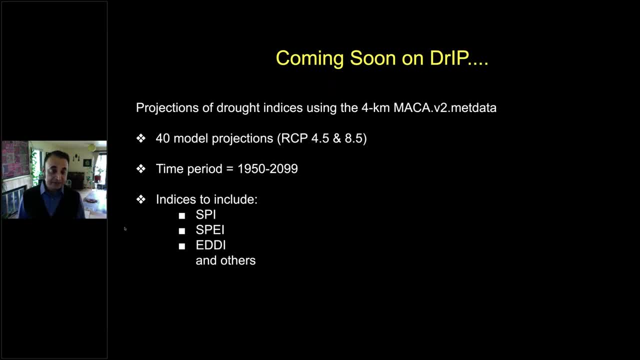 Okay, Thank you. So again, this is the audience who are listening. It's all the way up to the president. We're going to try to keep it a bit longer. Yeah, I'll explain everything and just a little bit more about the DRIP work. 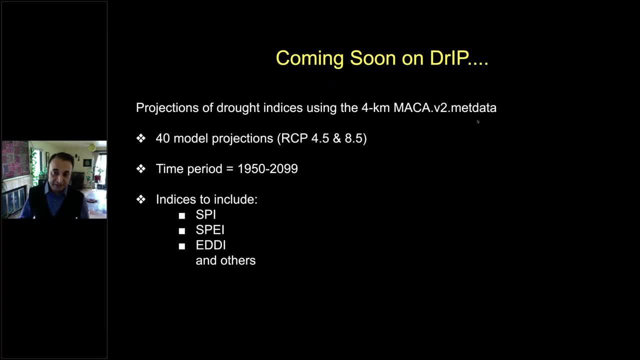 So DRIP is a big piece of data. You can check it out there. You can see on the slide. you have it дced at a four-kilometer spatial resolution. Yeah, So we will be. we are developing tools using the Maca V2MET data downscale climate projections. 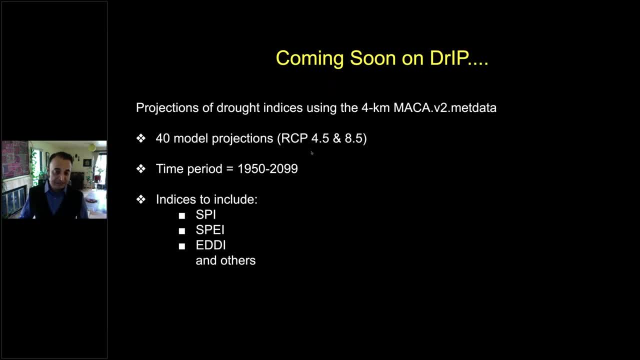 just by 40 models to emission scenarios, moderate and high emission scenarios, and time figure going all the way to 2099.. So you know, we have plans to basically put the indices available at 50, 400, 500 hundred. 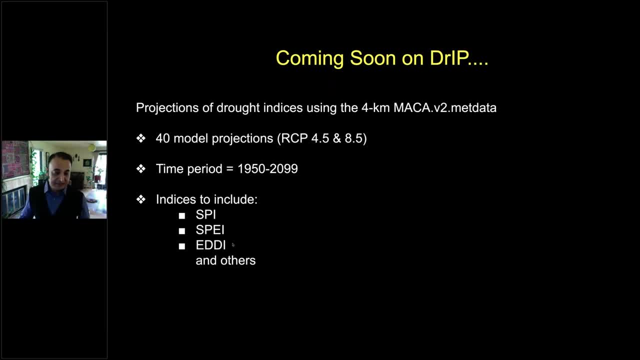 UNDRIP, but primarily SPI, SPEI and EDDI. you'll have these projections available. So you know, maybe it would be useful to a user like yourself who are interested in exploring scenarios of future drought trends. So that's all for me, and thank. 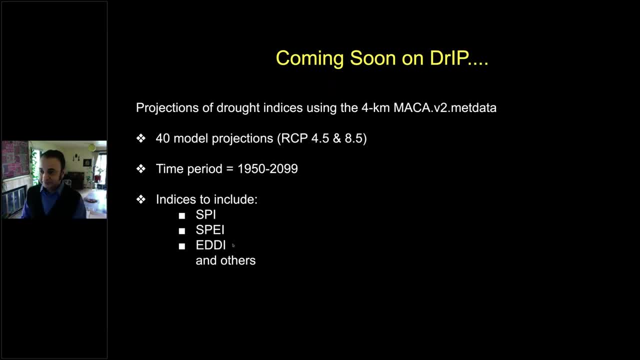 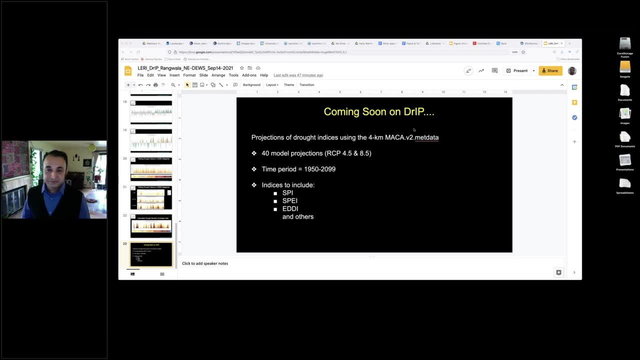 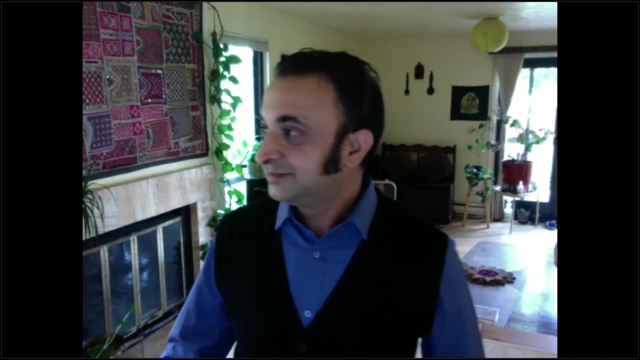 you for listening. I'll hand it back. Great thanks so much for that, MTS. A ton of great information there. and thanks, Mike, And I think we're going to move on to Q&A. It looks like we have quite a few. 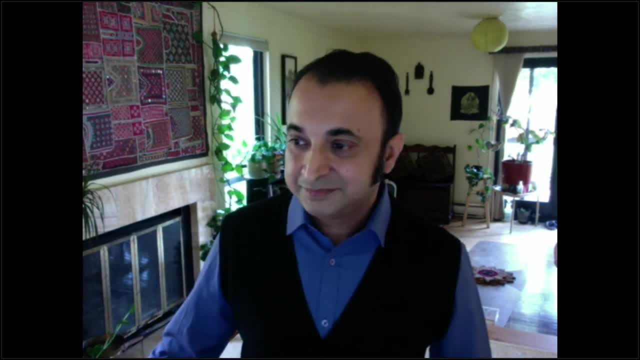 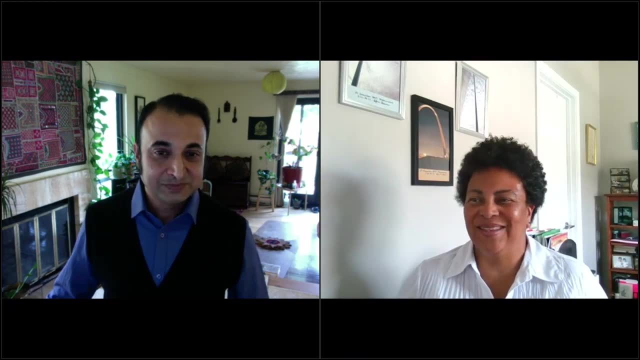 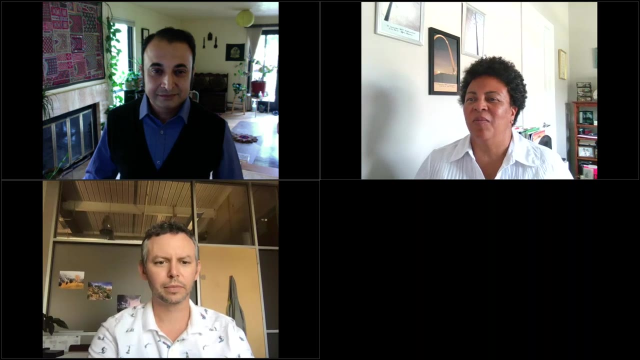 questions in there. I think we'll try to get them. get to as many of those as we can. And there is Sylvia. Hi again everybody. It's been busy in the chat box as well as the question box. Let's jump right to it. I'm going to start with Carlos Velasquez. Carlos. 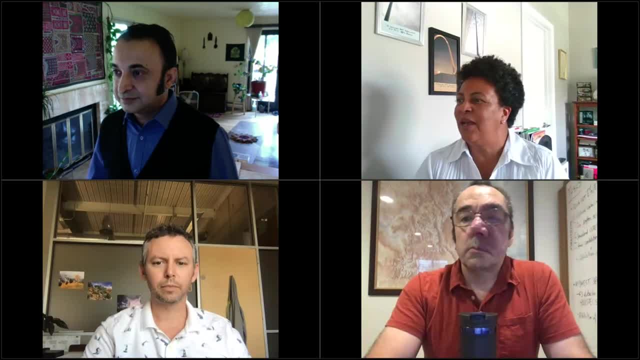 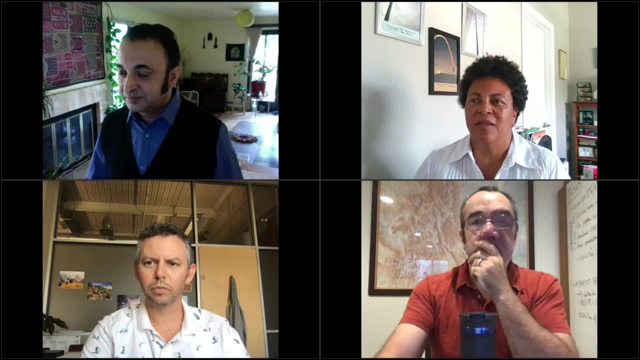 raised his hand very early on in the presentations, but I didn't see his question until later, or maybe he has to. Carlos, I'm going to unmute you if you want to go ahead and ask your question. Can you hear me? 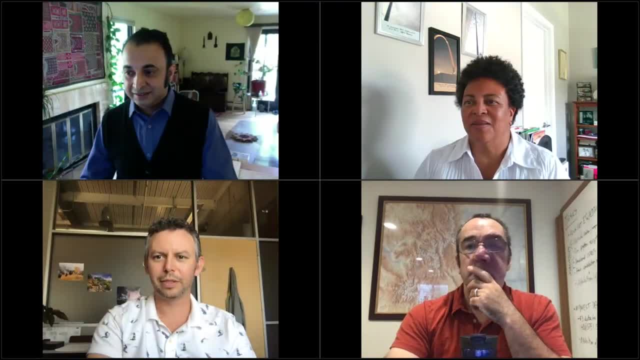 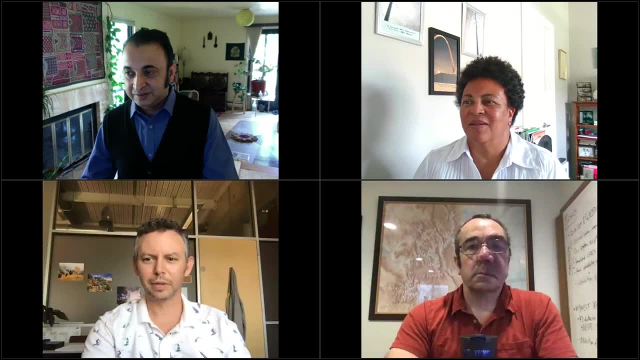 It's a bad echo, Carlos. He's self-muted. Maybe he'll come back. Hang in there, Carlos. I will go ahead and start with a couple other questions, And I think we'll start with Glenn Kohler's question. Can? 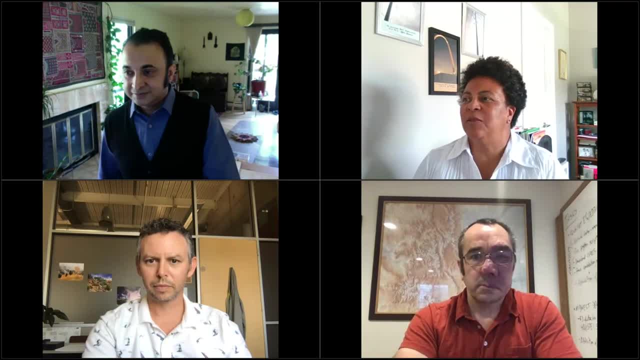 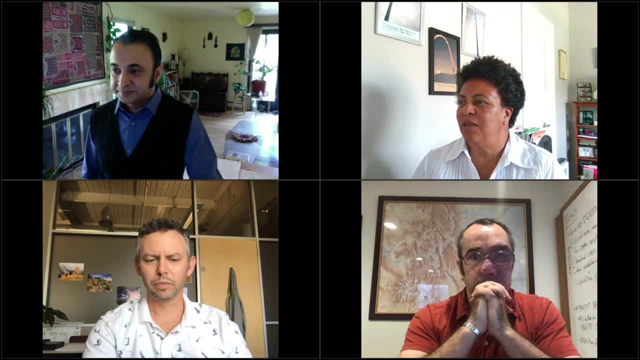 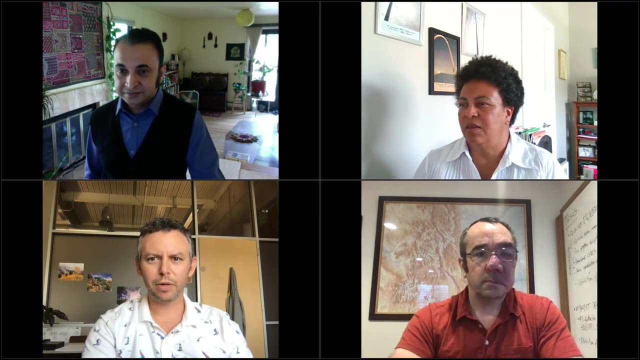 you generate a trend for number of days per year over 90 degrees Fahrenheit, And I believe this came in during the. was that your presentation, Dan, or was it Mike's? Yeah, I did show a trend map for the land surface temperature. Yeah, so with the trend, 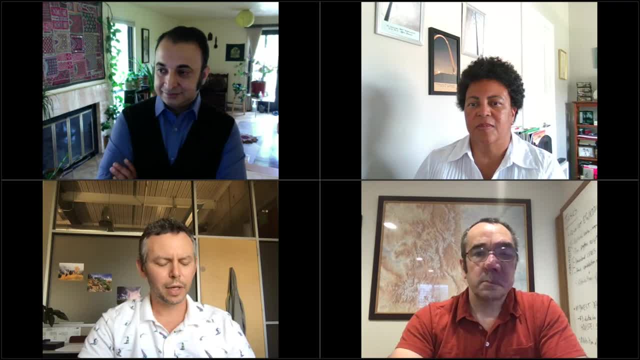 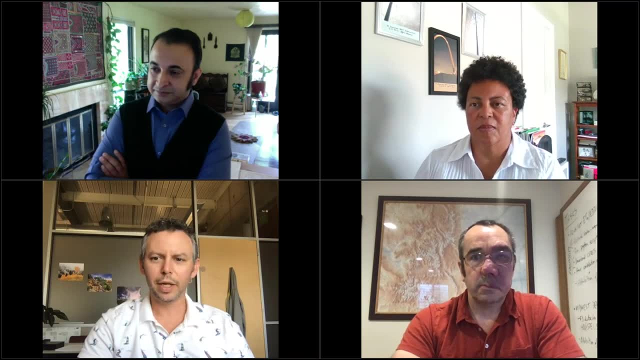 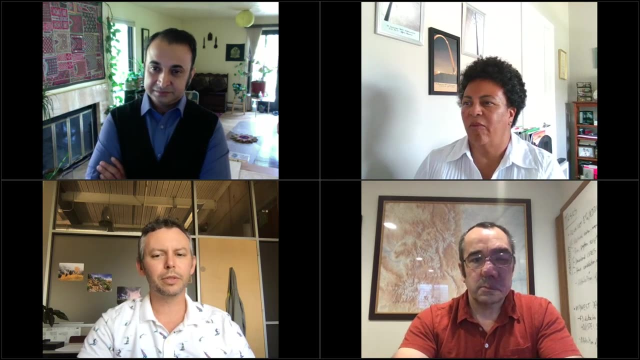 spatial trend analysis and climate engine. right now, you basically select a time period, whether it's a month or a week or a year period. I don't think we currently have the option to select thresholds, but that's a great. that'd be a great addition, And I will just 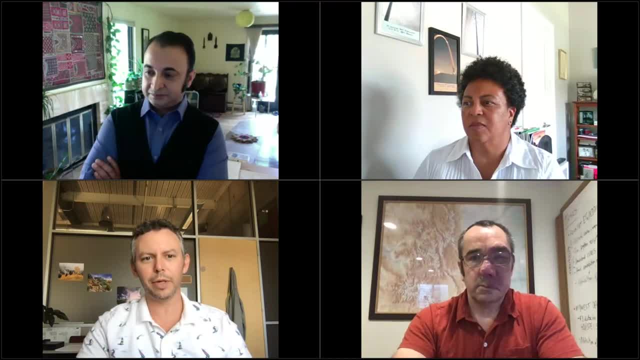 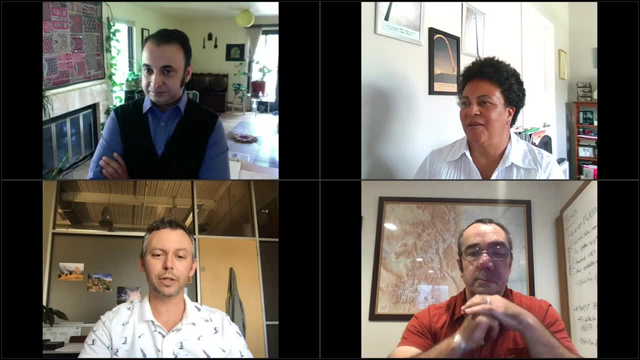 mention that part of how we get these new things in the climate engine is just like things like this: We hear these ideas and get requests from users and we do incorporate them in. Yeah, bring it up to the development team. So thank you. 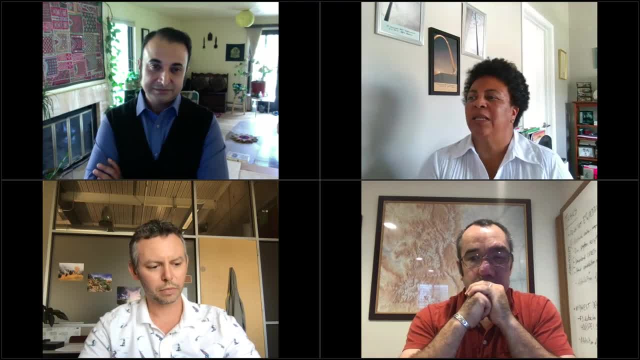 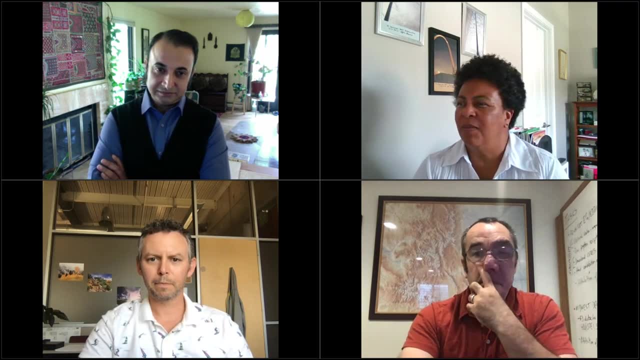 Yeah, Glenn also asked if there was any chance of getting an EDI or an ESI forecast map for week one, one month, two months, et cetera, Although I think Mike might've answered part of that, So I don't do forecasts. 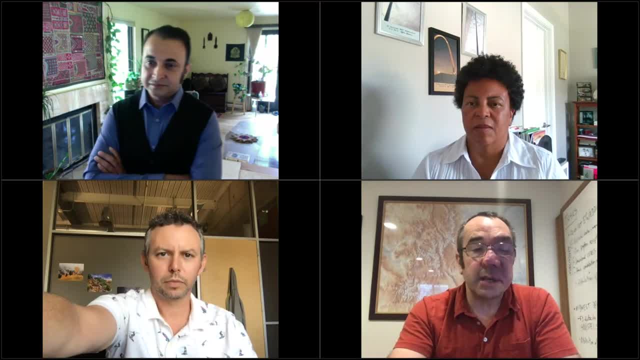 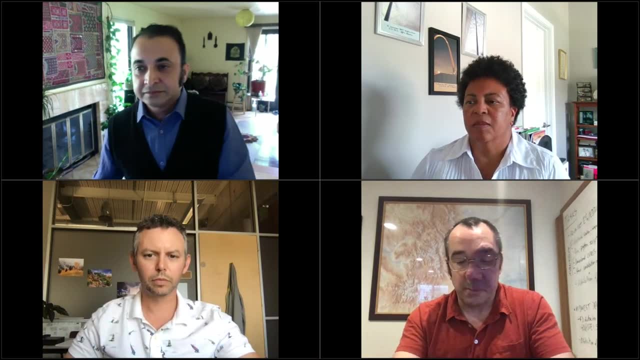 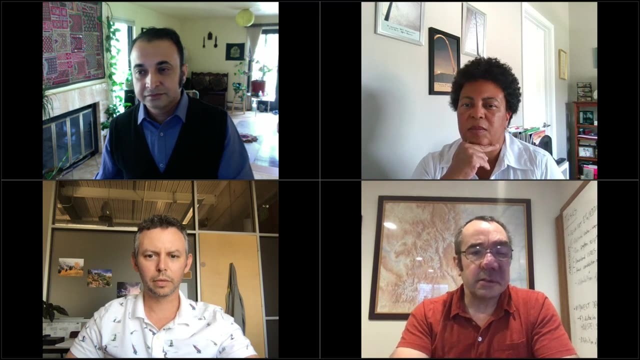 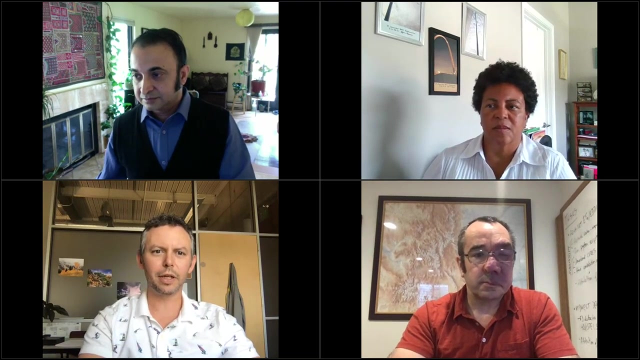 EDI is ongoing monitoring, So it relies on reanalysis data that assimilates observations into like a surface map. But I think Dan's shop is looking at forecasts of EDI, So I should actually let him answer. Yeah, so I did mention we have the CFS downscaled. 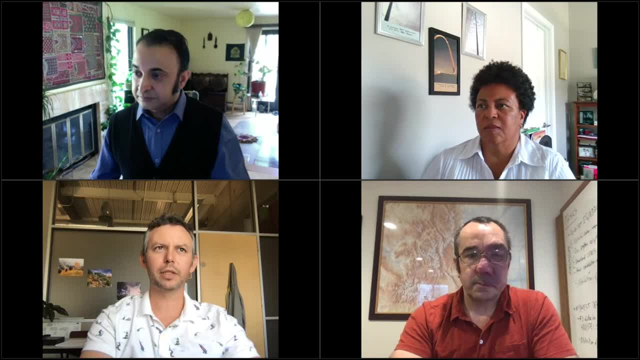 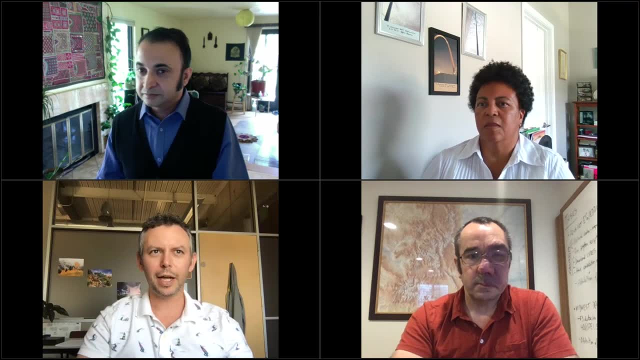 climate forecast system downscaled from one to four weeks out to one to four weeks in climate engine And we do actually have EDI forecasts in there. Yeah, I didn't have time to cover everything that was in climate engine, but if you do go to the forecast section, 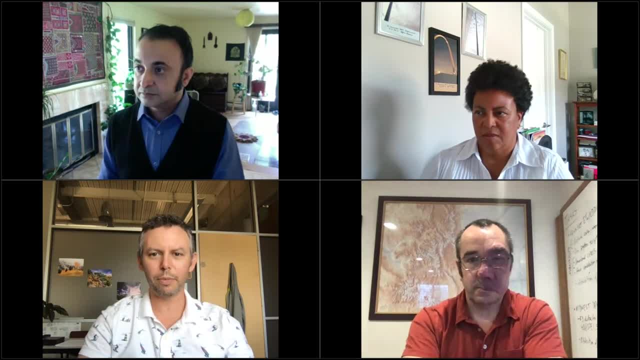 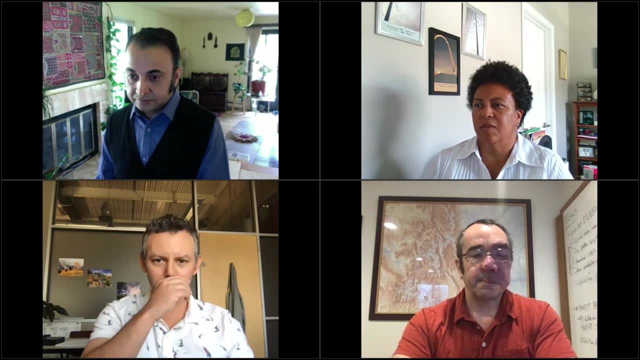 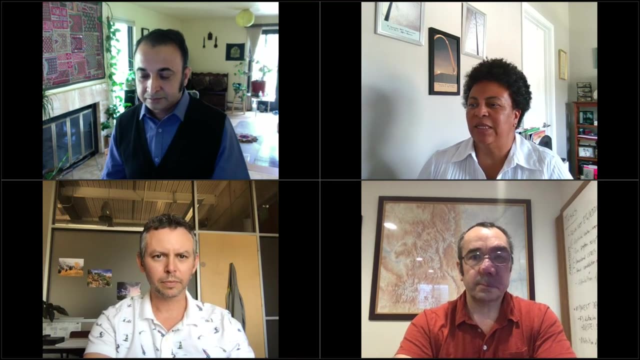 in the dropdowns. there you can find weeks one to four separated out by week. if you want ensemble media and EDI forecasts Got it And let me just stick with Glenn's question. When we got to Larry, his question is: 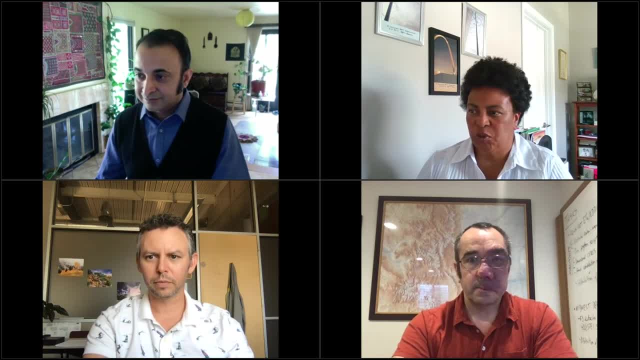 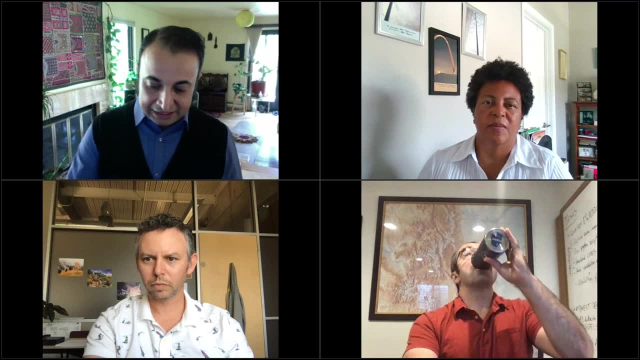 what soil depth does EDI have? What soil depth is Larry tuned to or best represent? Yeah, that's a great question. So Larry's based on the land surface temperature. that's really looking at the kind of skin thickness, which is about five centimeter. 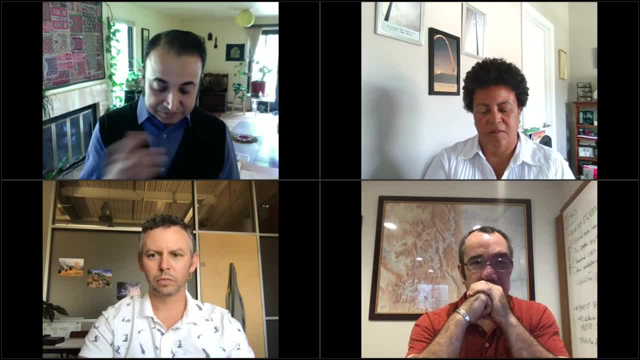 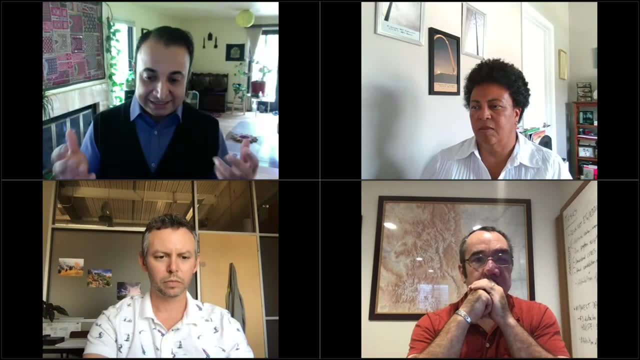 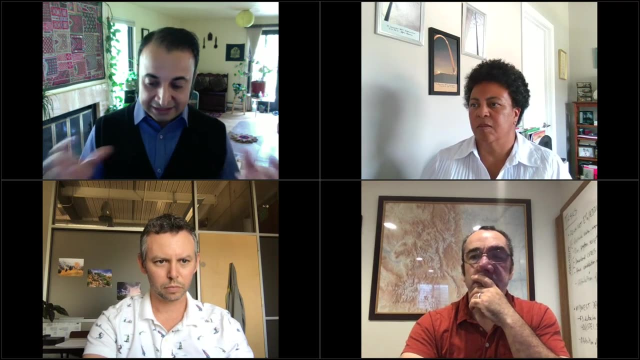 Our sense is that it's more sensitive to all that part of the root zone that is involved in ET process, because that ET's- the whole of ET fluxes, which is maybe going down all the way to the root- is influencing land surface in temperature. 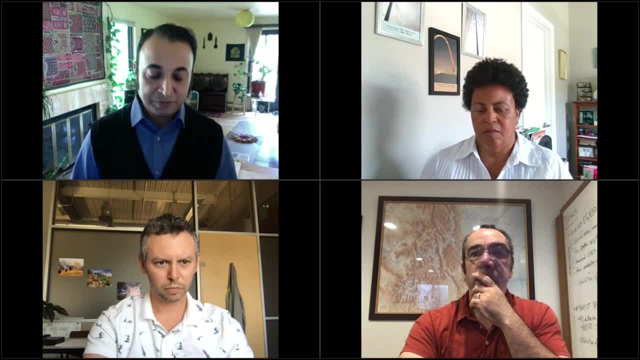 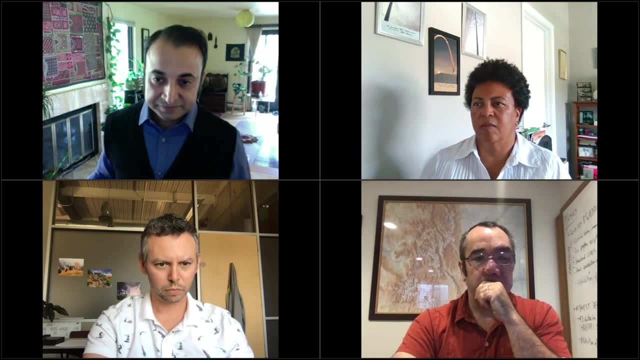 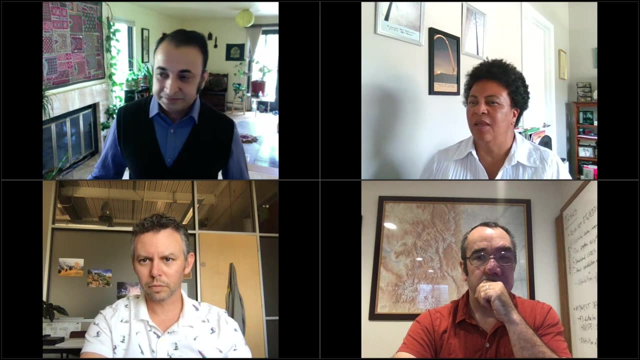 So I would imagine like at least from zero to 40 centimeter, if not more, But we see skills at the depth as deep as one meter. Got it, And let me try to unmute Carlos one more time, And if not, I did get at least one question for him. 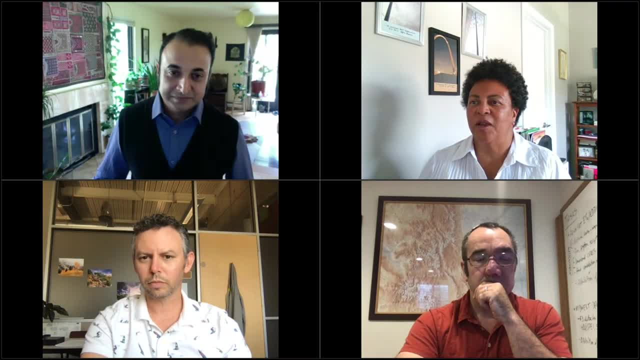 which is an interesting one, Carlos. can you hear me, Carlos, I'm unmuting. We'll try it one more time. Uh-oh, looks like that's not going to work today. The one question that Carlos did get into the chat boxes. 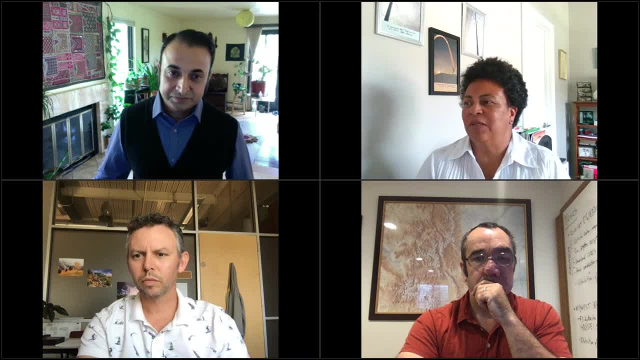 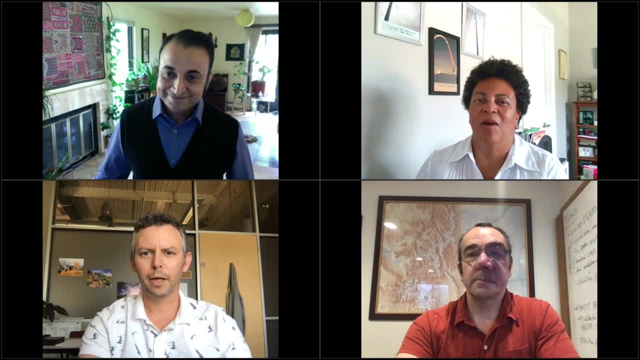 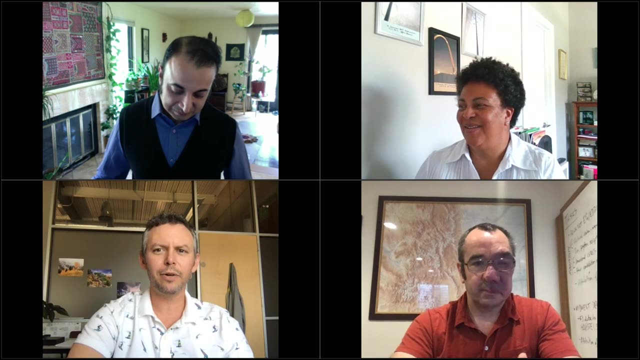 is a really great one. Could drones help us get data with better resolution so that the indicators are more accurate? Whole team try it. Yeah, I mean, that is, of course, a great idea, And I know that drones have certainly been used. 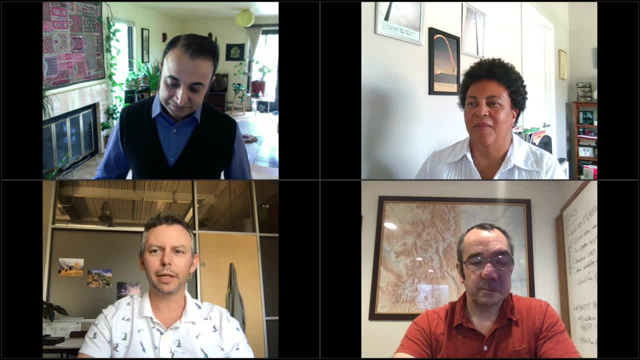 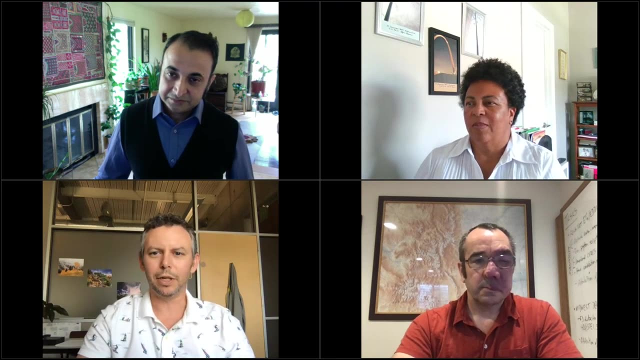 at the research scale for mapping individual fields, and also some snow mapping is being done with drones. It gets very challenging to scale it up to a larger level, to incorporate into something, like you know, a national scale gridded product. But yeah, certainly drones can tell you a lot about. 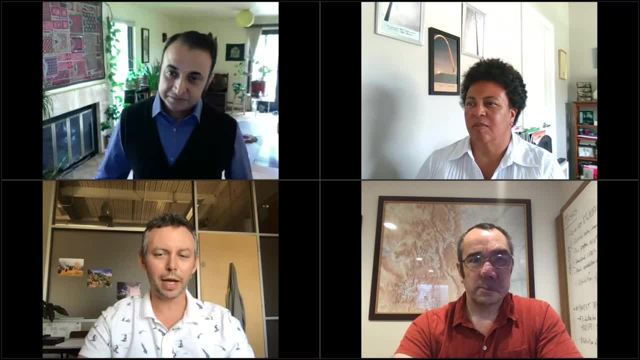 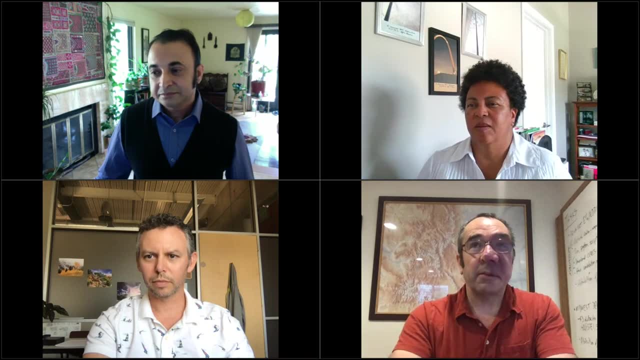 the land surface at very high resolution. And I know, yeah, at the research level it's certainly, they're certainly being used. Yeah, and I would say, speaking from the perspective of Eddie and the evaporative demand, I think the increased resolution. 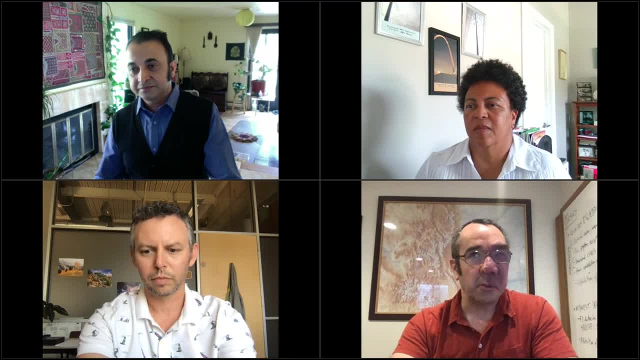 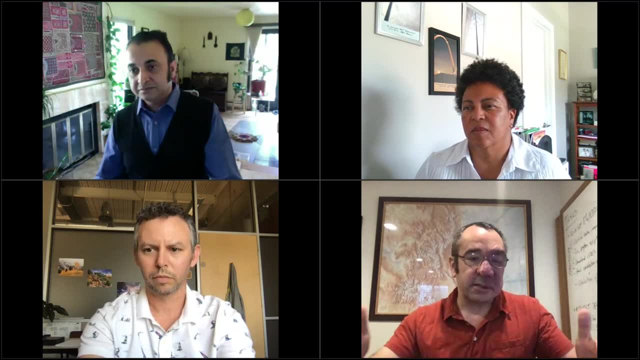 that would be afforded by using drones would be wasted on a product like Eddie, where it relies on a well-mixed boundary layer And so it has this sort of spatial averaging effect. anyway, You wouldn't pick up much more information if you were to use a drone. 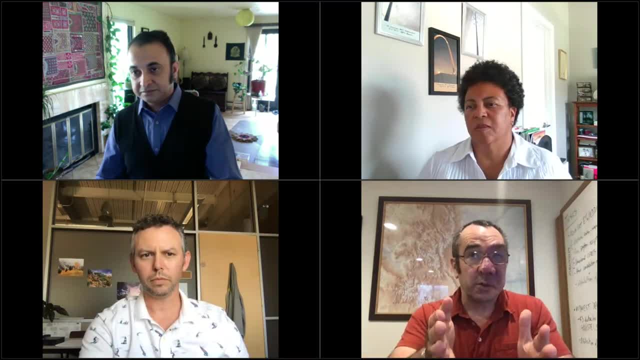 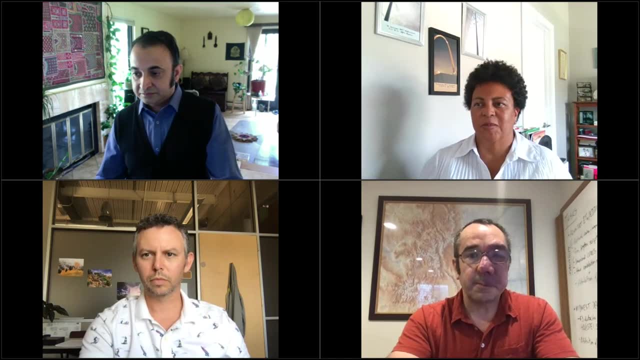 Granted that Eddie's at 12 kilometers. so we would like to go to a finer resolution, but not necessarily to the resolution afforded by drones. I think that wouldn't help. That's a good one, And we have Vicky Zelte. 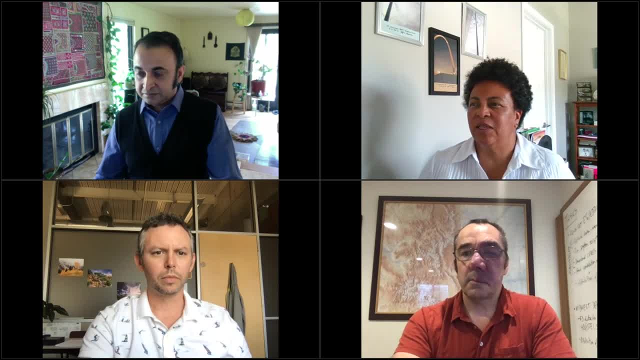 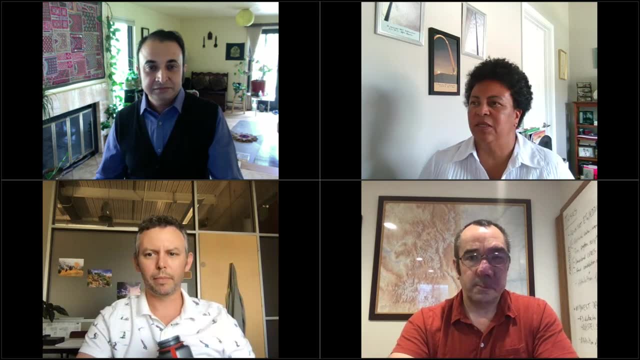 who was unable to stay with us for the Q&A session, had to leave, but she did leave us several questions. First of all, and I think this goes back to the time of Dan's presentation, can data behind the selected grid, met products and maps be downloaded? 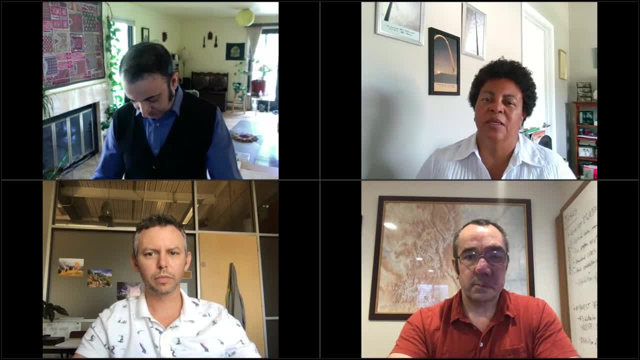 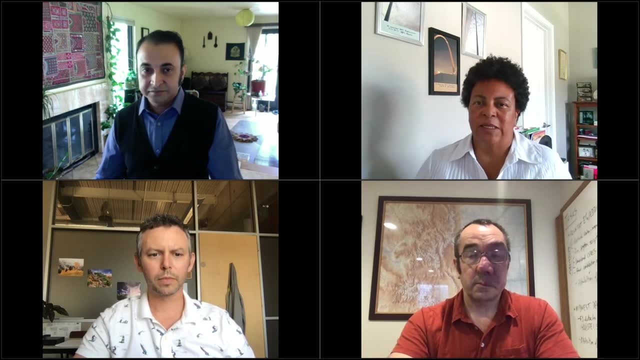 for additional local processing by local drought regions. A lot of our Northeast due states have drought dashboards where they're processing or at least displaying some data, So that's a good question from Vicky. Yeah, that's a great question, And if you just want to use it for a one-off, 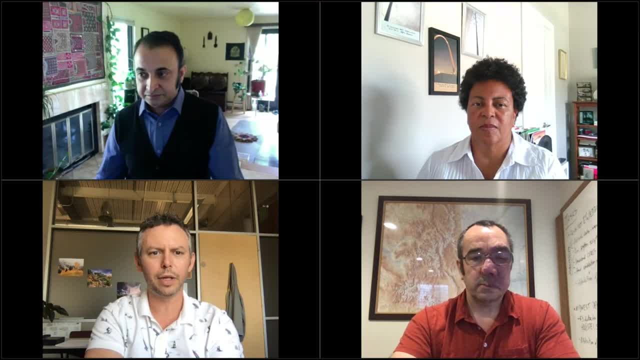 yeah, any of the data in there that I was showing you can download. But time series you can get the entire period or record for any grid met variable. We do have a bunch of different polygon regions in there. We have state level, county level, climate division. 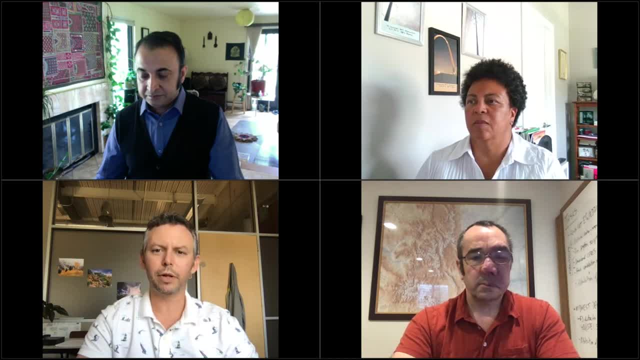 as long as along with a few other different regions. So, yeah, I would encourage you to check out the time series options available in climate engines. We do have a bunch of those regions, But if you wanted it for something like a dashboard, 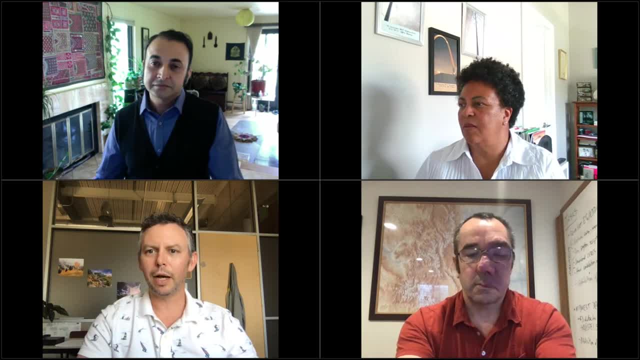 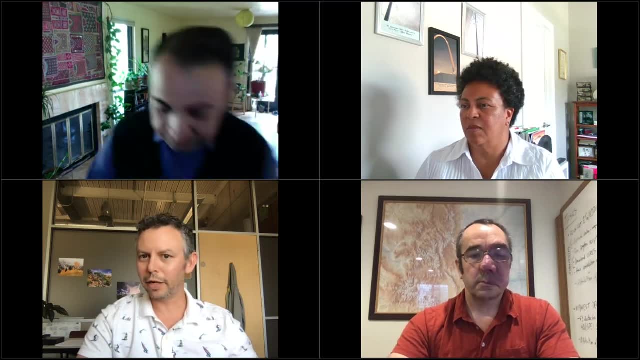 like I showed there in the end with the Droughtgov example, that's where the API would be extremely valuable, So you can basically send a call to Climate Engine each night if you wanted to update your drought dashboard, And the calculations are already being done. 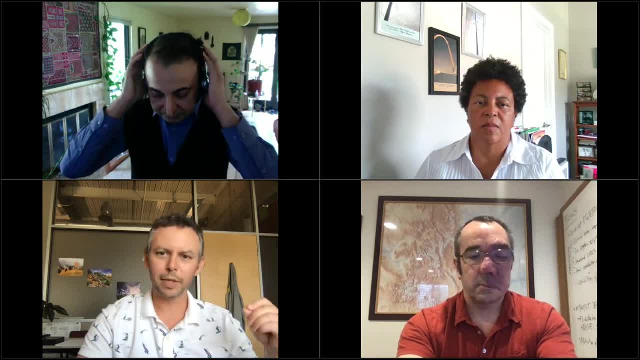 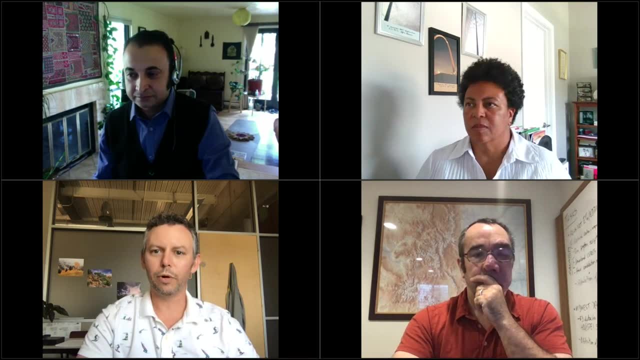 in Climate Engine. So you're basically making a call and saying I want the 60-day percent of normal precipitation and Climate Engine does the calculation and then returns the grid for you. So again, if you're interested in the API, please contact me. 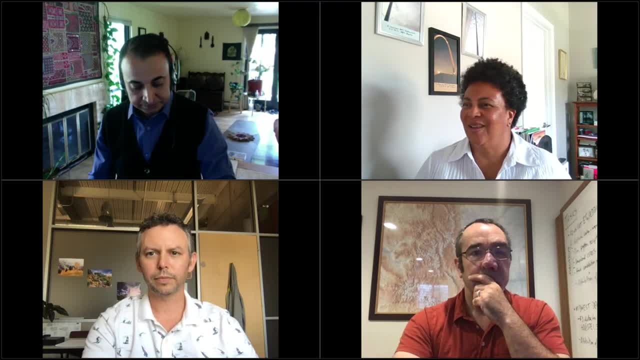 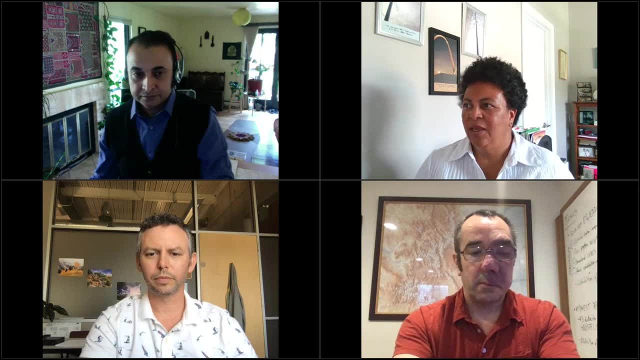 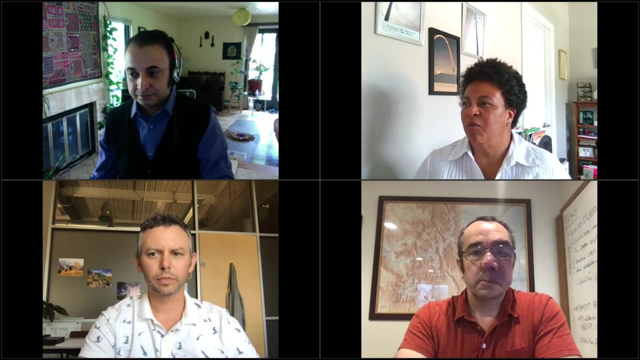 I'm one of the other Climate Engine folks. Vicki also asks or states: we found false positives for eddy? It must be considered with SPI and the other indices. It can certainly warn a flash drought when precipitation is already low, but at times high precip and high heat. 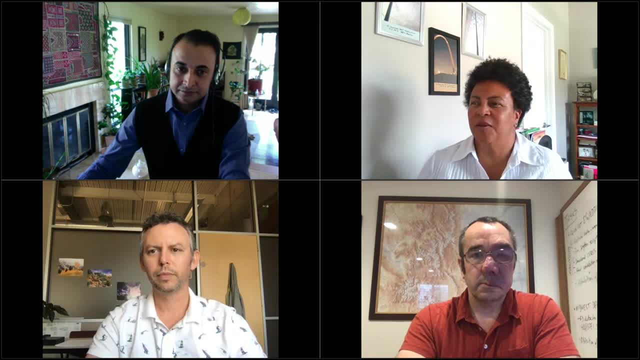 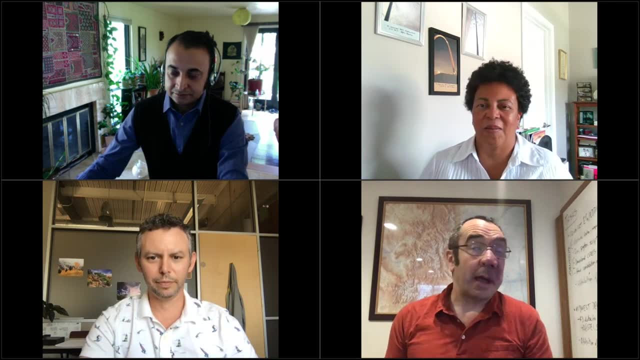 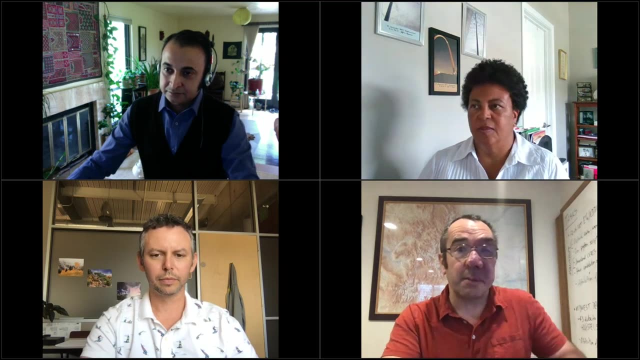 and that will result in a false positive. So I'll hand that to Mike to source that. Yeah, that's absolutely true. So eddy does not have any precipitation input. So if you have a hot period and you get a significant pulse of rain during that period, 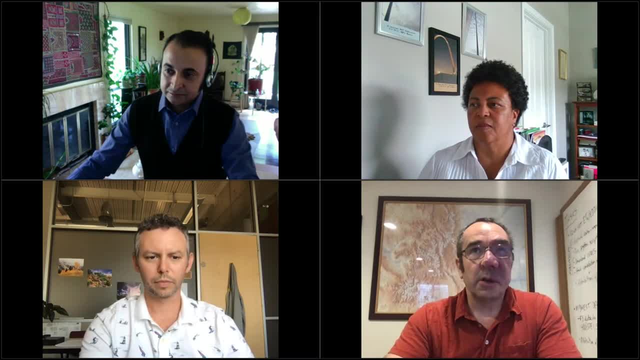 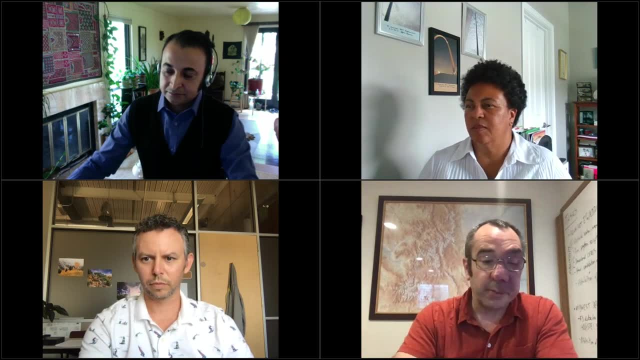 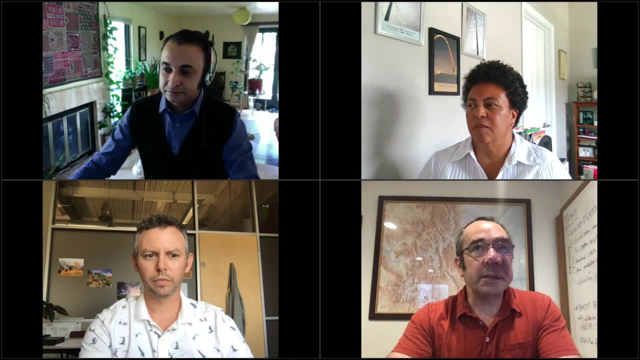 you will get an elevated eddy that is not necessarily reflective of a drier ground surface, but is just reflecting the heat wave, if you like. So I would particularly. if you're interested, you can send me an email. I'll send you a link to that. 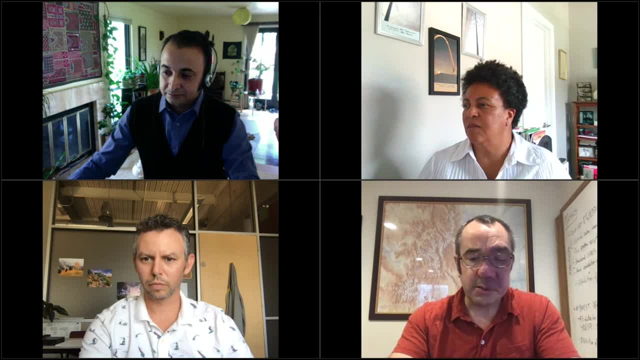 But particularly in the northeast, where you have a more energy-limited environment as opposed to a water-limited environment in the west. I would take a flag raised by eddy as a potential Potential exists for drought. not you're in drought. 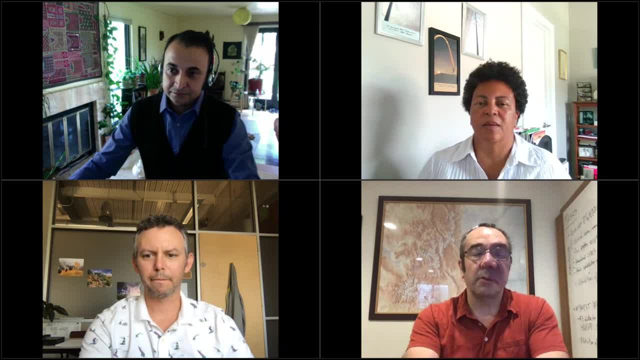 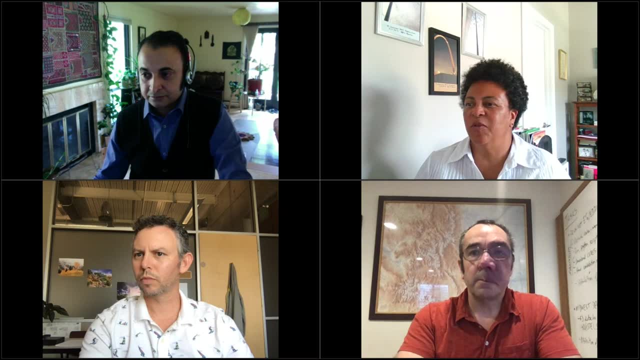 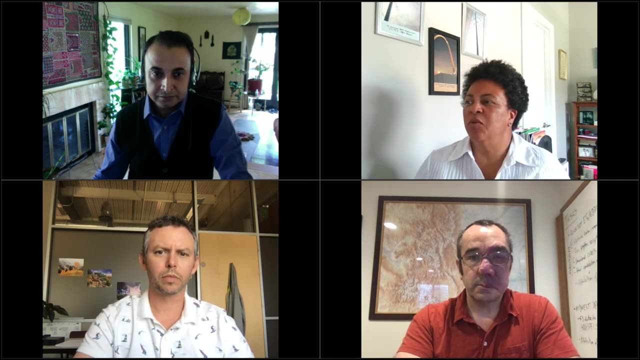 It's definitely a potential rather than a warning. She's absolutely right. Yeah, I think I'll finish up with one more of Vicky's questions and then we'll move on. Could low AET, Larry, mean that it's cooler weather? 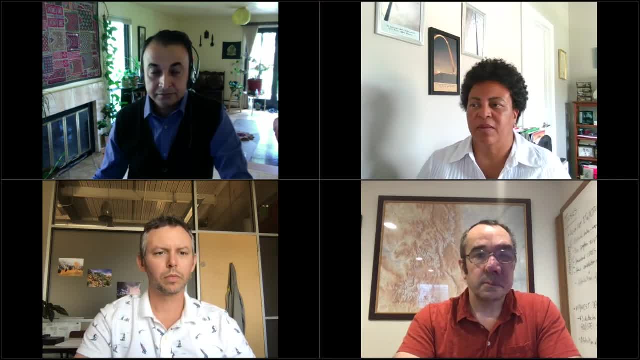 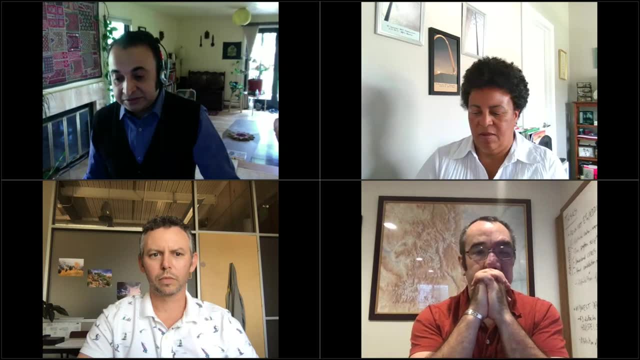 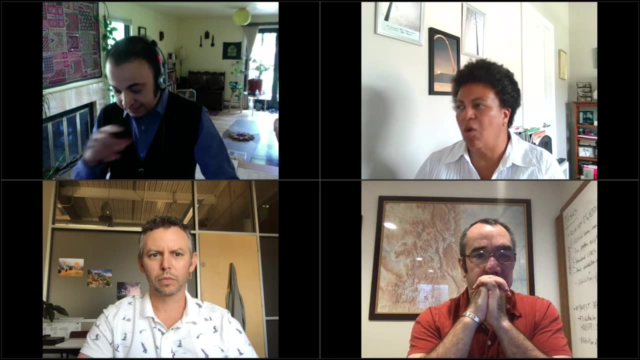 than normal rather than drought. And how can you distinguish that? Yeah, low AET would really mean that the land surface is very hot, So it would not point towards cooler conditions. because, again, Larry's looking at land surface temperature, temperature values and seeing how enormously high 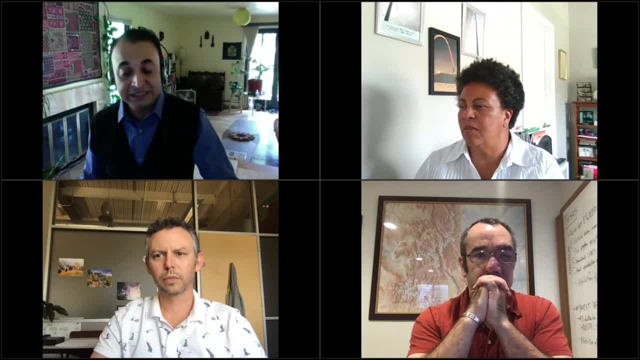 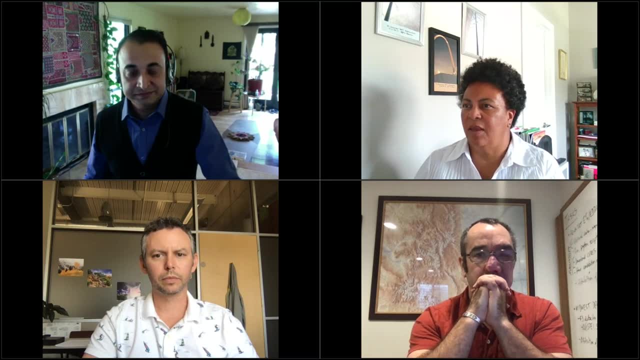 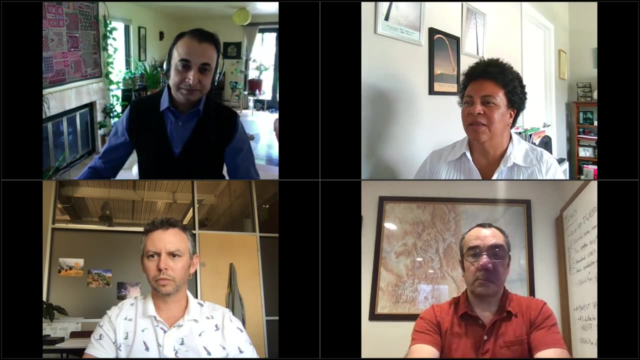 or low, it is from normal. So very high temperature value should give you low AET, And so it should point to hotter conditions and not cooler conditions. Okay, got it. Next some questions. Art Degatano- I can't quite see if Art's still with us. 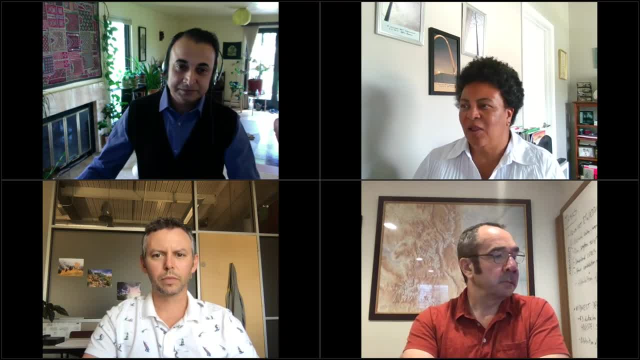 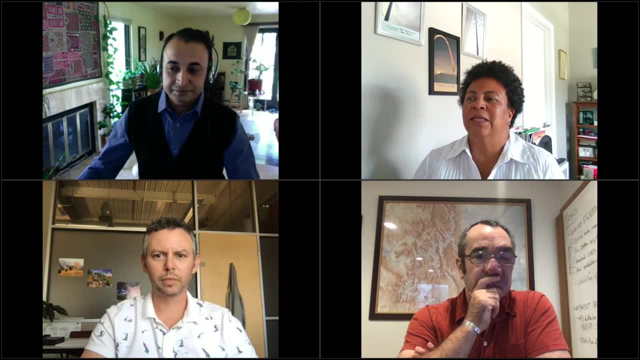 Art asked what happens if a field is fallow in one year and in corn the next? Okay, So if you're in your field, you know the corn is heavily undercooked, so corn would be growing over time. You might see a drop in the corn growth in the winter. 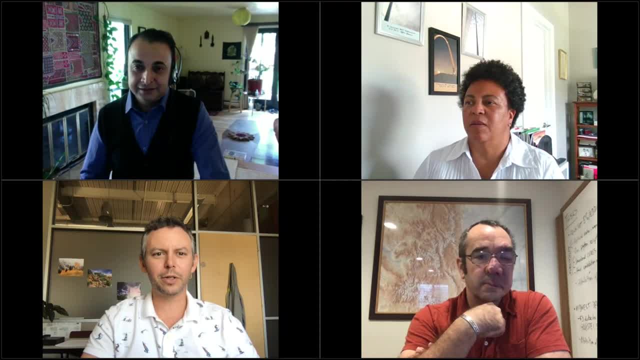 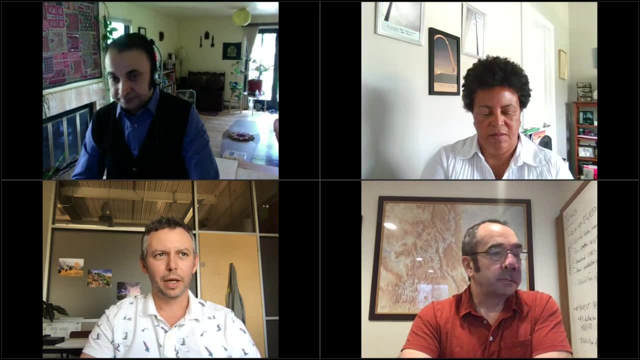 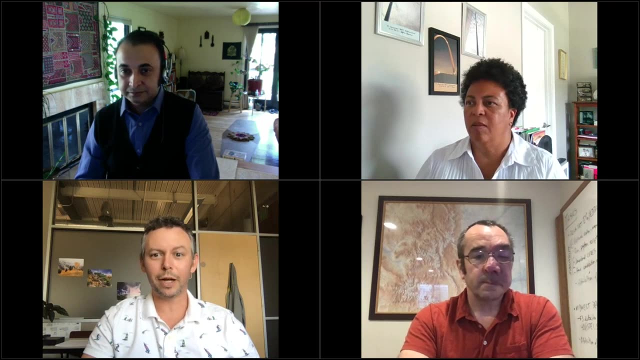 So you have a lot of value for corn. So I think you're very well aware that there's a lot of room to invest in the corn growing areas and I would recommend that to anyone who thinks that the crop type would impact NVDI quite a bit. 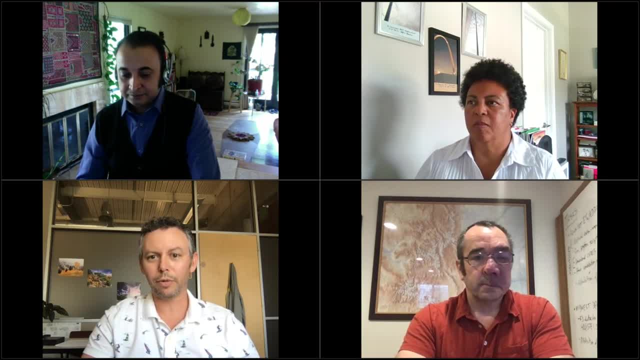 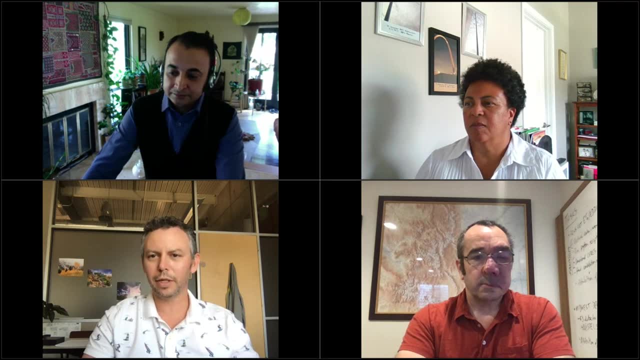 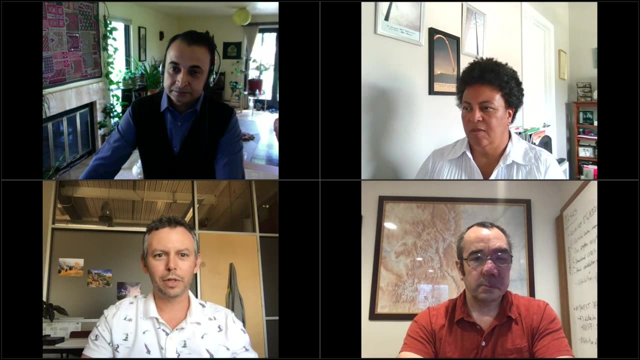 And this obviously can change from year to year how it relates to the climate information, um, because, yeah, certainly, uh, if you have a different crop or, as i mentioned, uh if, say, at the early part of the landsat era it wasn't even a farm at all, it might have been a forest or something else, uh that would all that stuff would change the 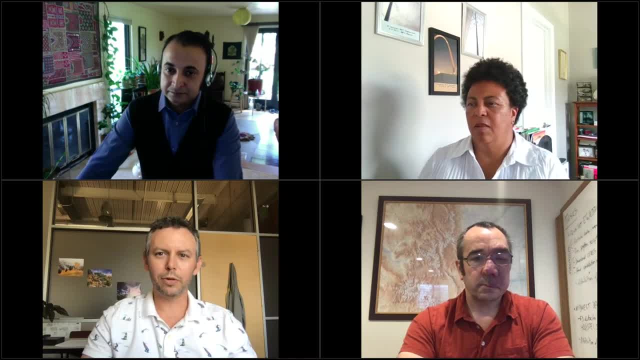 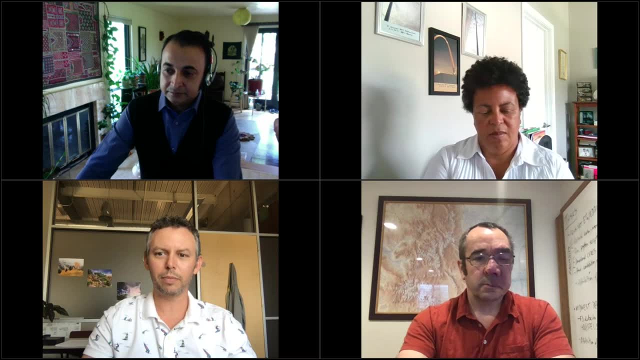 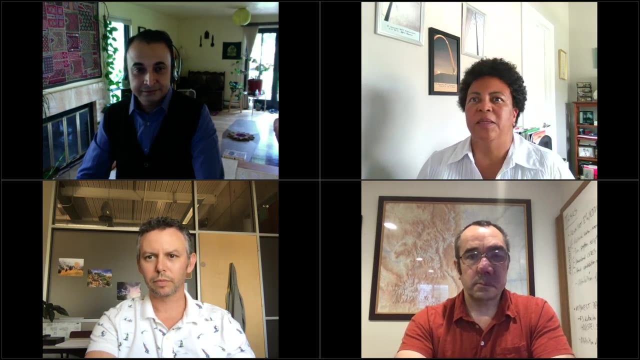 the ndvi values. so, um, it can be tricky interpreting um, unless you know exactly what the, the land cover and land uses. so that's a great, great point. okay, let's go to a question from jeffrey zimmerman. uh, jeffrey asks: are esri web mapping services available for climate engine? 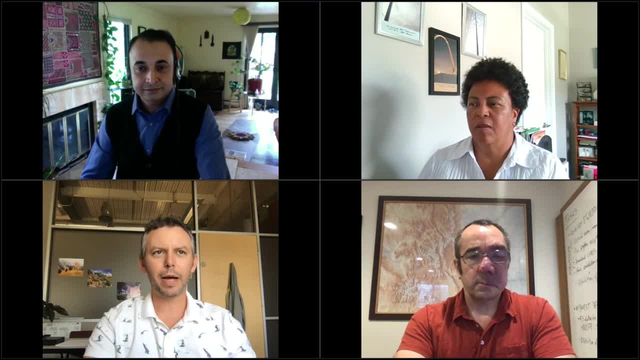 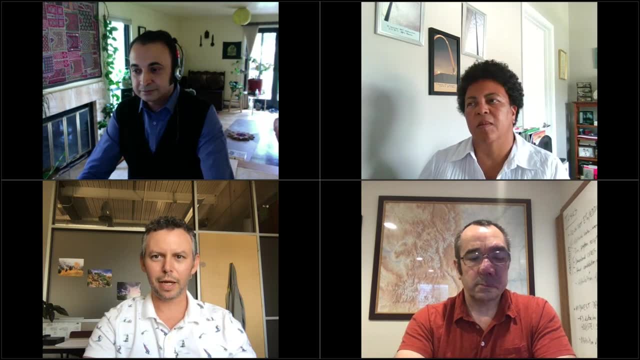 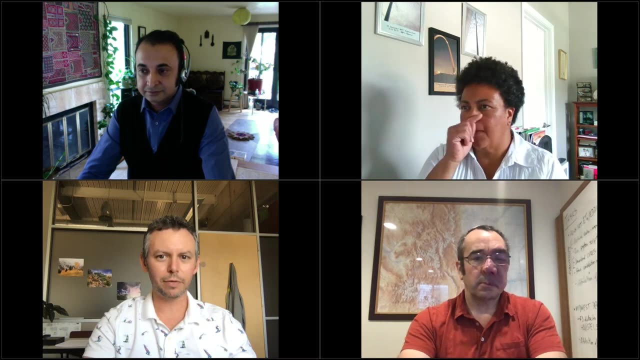 um, i don't think so and i'm not sure i know about enough about that to really answer that that might be an api related thing. um, so, and and if, if this person wants to chime in sylvia- i don't know if they're still on, but 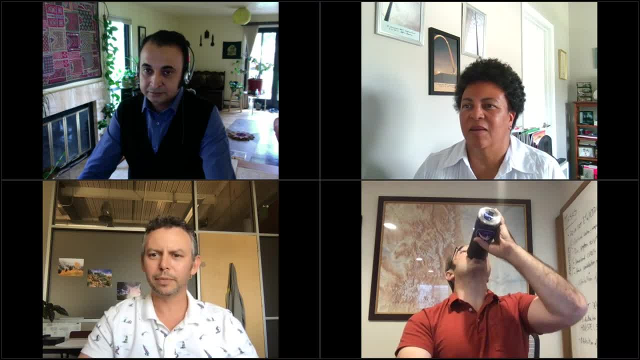 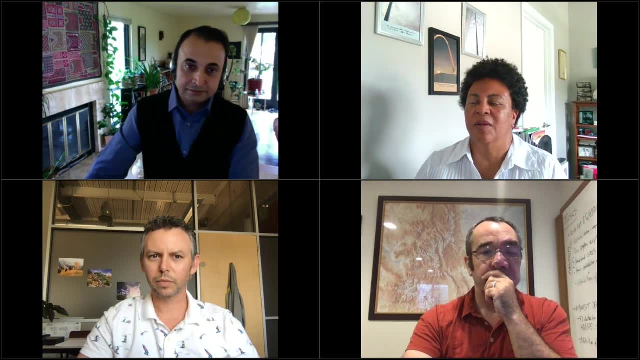 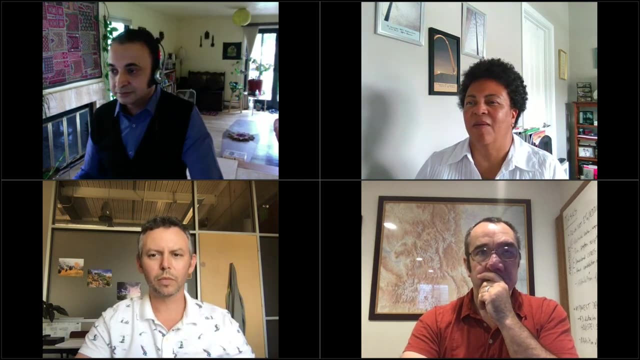 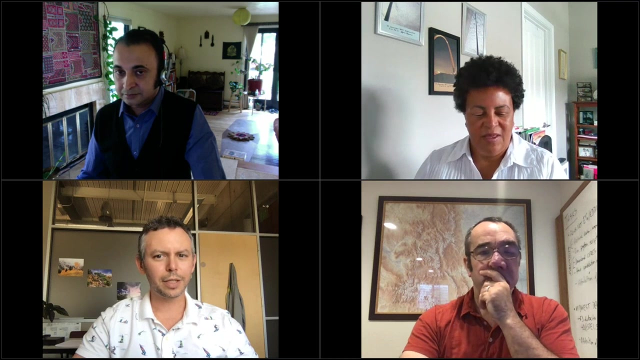 um, i'm not sure if i can answer that question. really, jeffrey, i think i see you're still on. i'm going to unmute you and you might have to hit your unmute button as well. but, jeffrey, i'm not sure if he's still. yeah, i'll say, as far as i know, no would be the answer to that, okay. 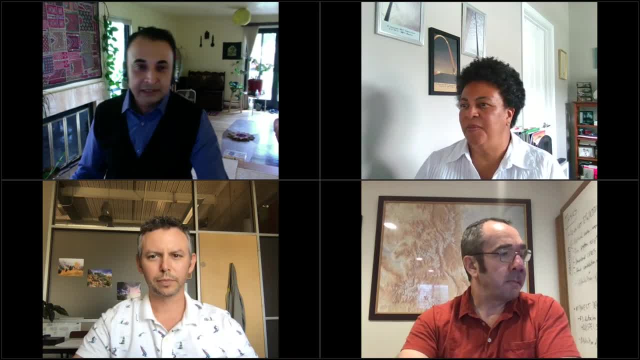 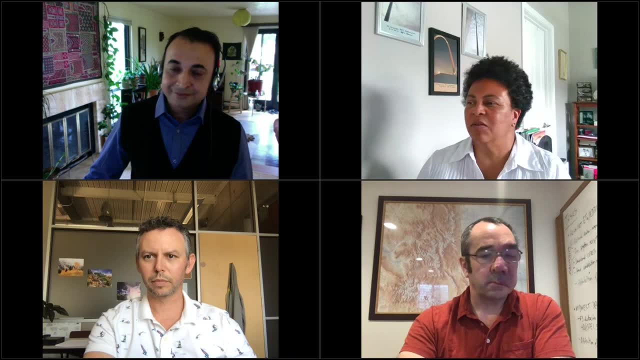 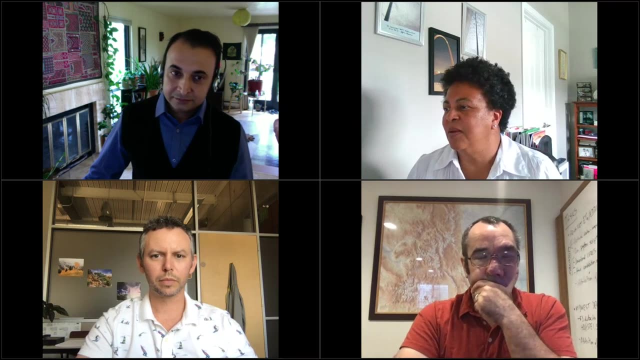 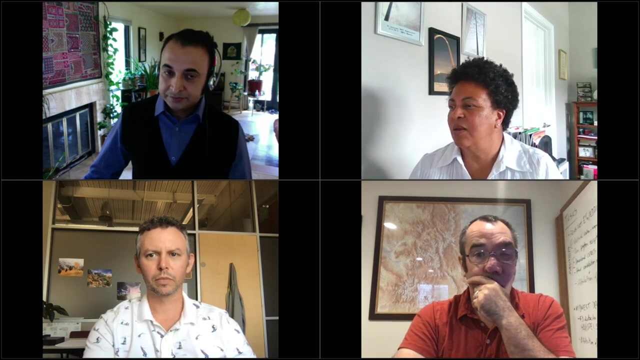 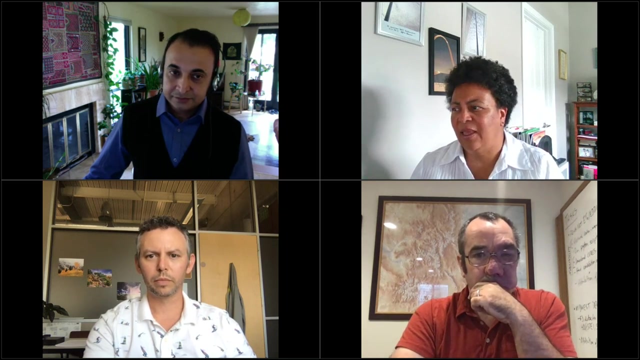 uh, let's go to um. eric b has a question, although he's left, but we can certainly record this answer. um are the three month indices on a one month step, three month running running average index. is that four are the three month indices on a one month step, ie a three month running average index? 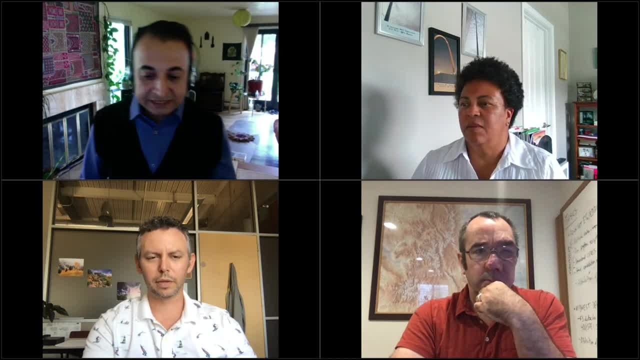 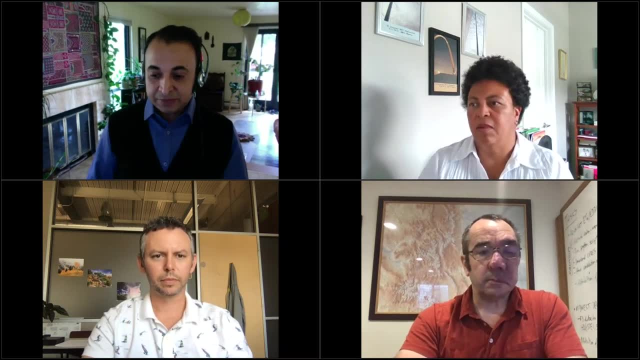 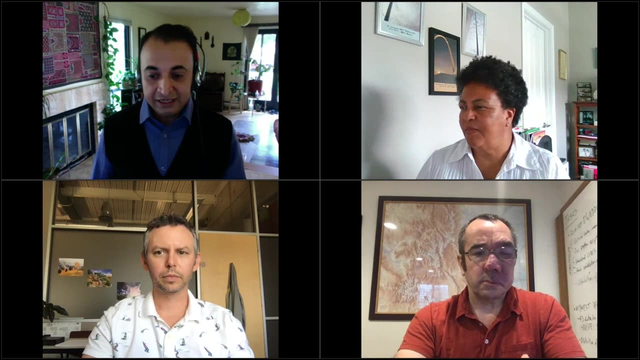 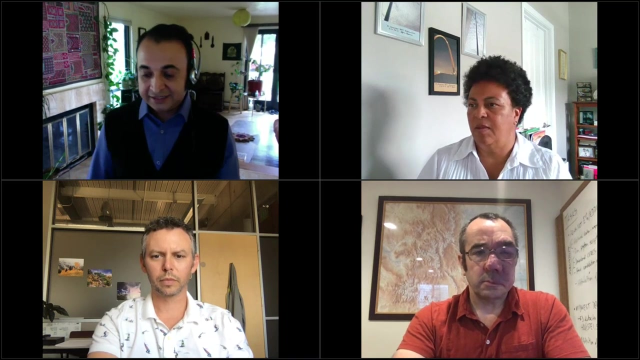 let me maybe answer about larry and eddie. so those are integrated, uh, accumulated, uh over three months, uh for ending in a particular month. so a three-month larry or eddie is really accumulation, three month of demand or response, and says ending in that a team on July Eddie. 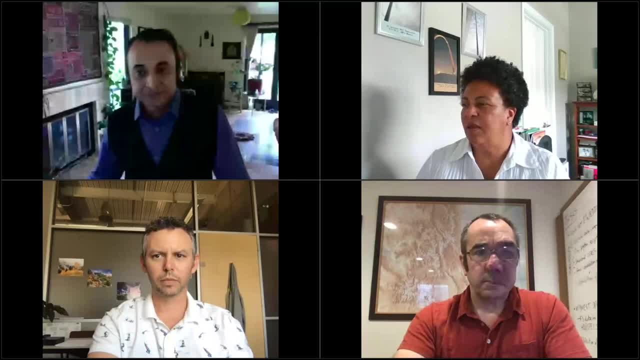 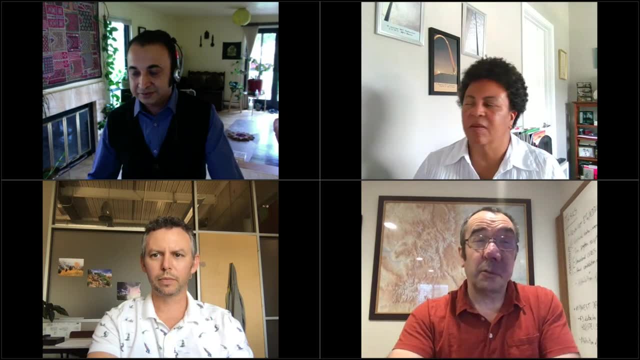 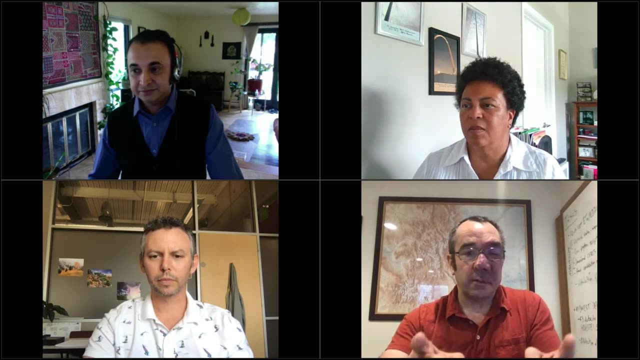 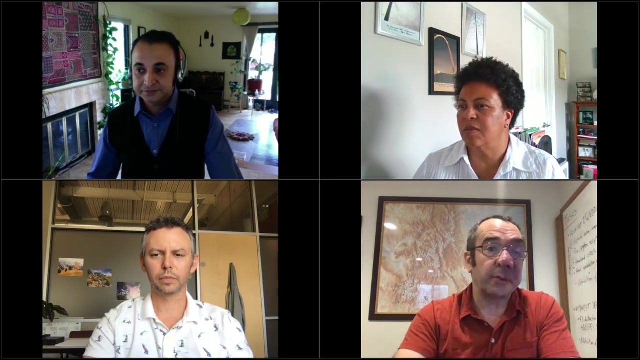 is three month accumulated, ending in July. it's not average running and, to be clear with regard to Eddie, Eddie is updated daily so that three month window advances forward every day and in fact, for every time scale that advances forward every day, and those data are posted to the to the web that I 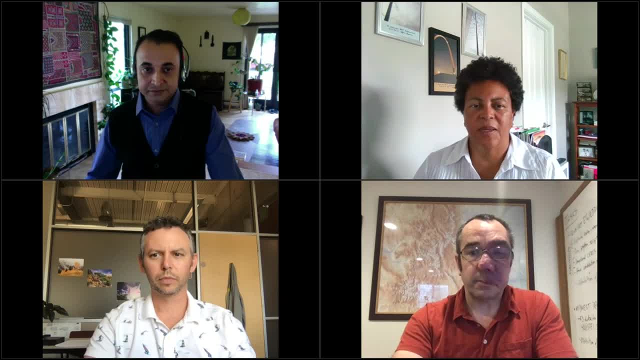 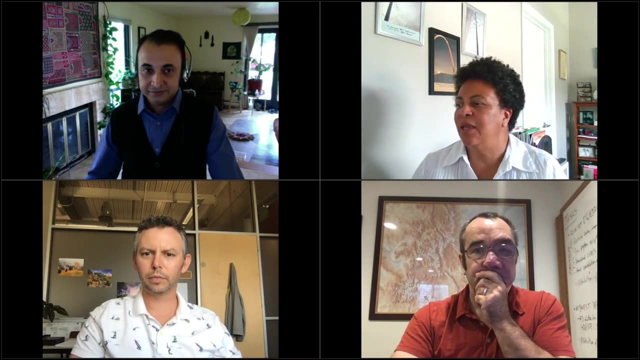 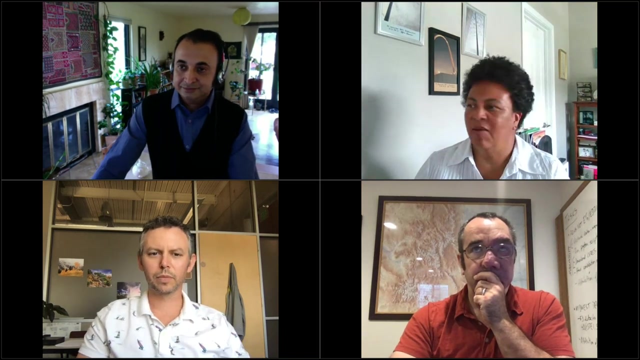 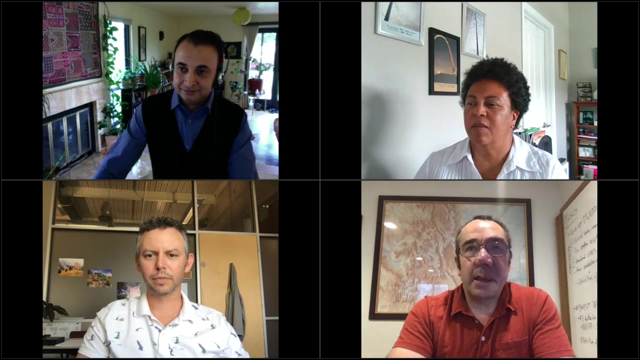 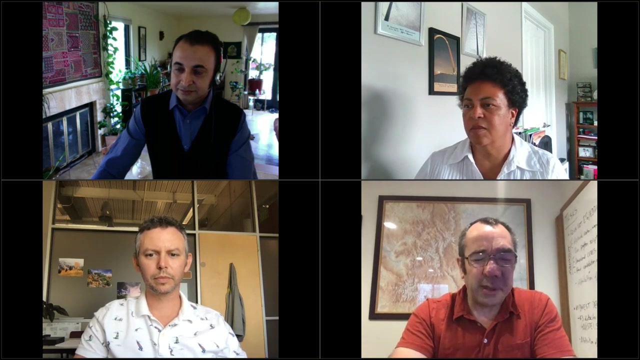 showed in the chat box. really checking the chat box real quick here this is a question from Trevor Edwin. Trevor asked: can Mike discuss how Eddie works in the cooler climates and during winter or non agriculture, non agricultural season? so, Eddie, Eddie clearly operates in the in the cooler climates, Trevor- I think Trevor is are. 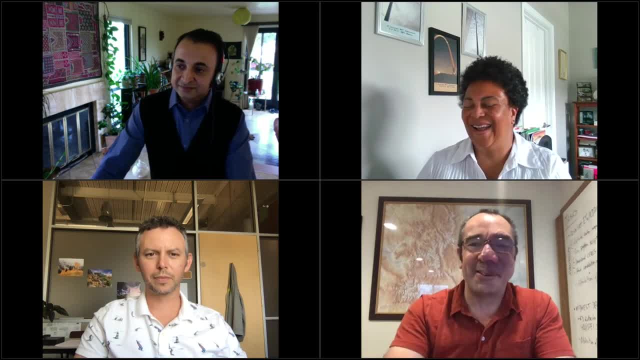 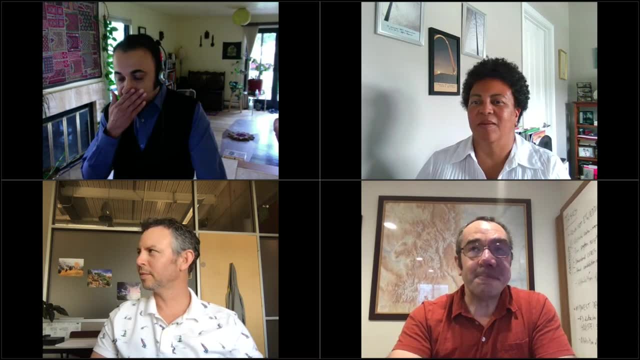 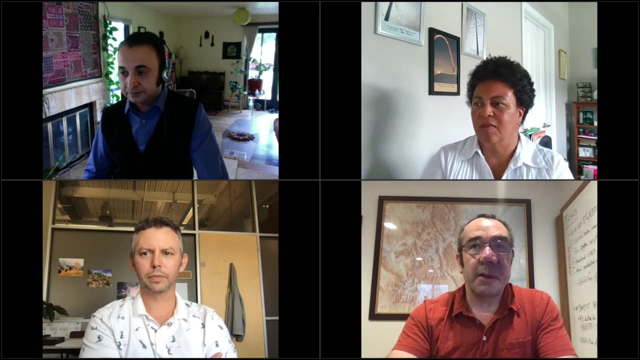 you in Canada. I'm trying to recall. I'm sorry. I'll have you in my email inbox. I'm trying to recall where are you, where you're talking about. but so Eddie covers. well, I have a global Eddie. I did not discuss at all, but eddie covers from 52 degrees north down to 25 degrees south. 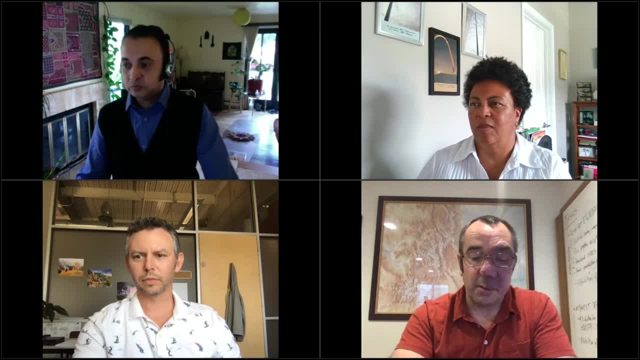 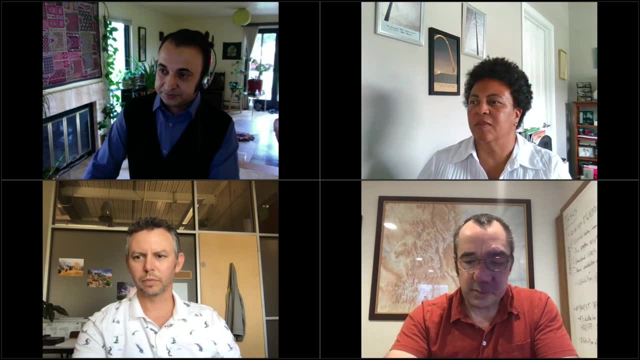 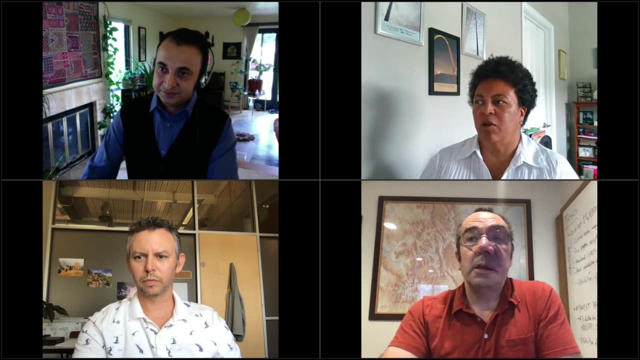 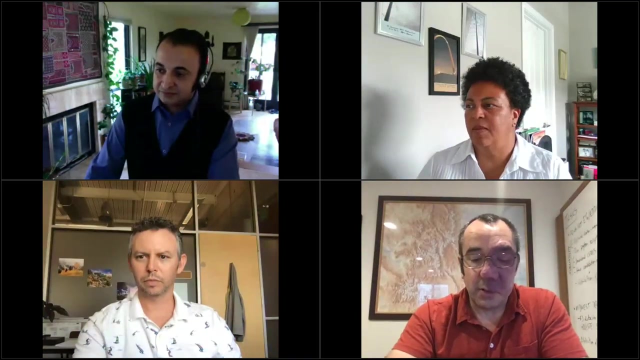 so there is coverage in cooler climates, particularly, you know, up into Canada. what does her classmares question was? I'm talking about? you know, always was better. Does Eddy work in the cooler climates and during winter or non-agricultural seasons? Right, so in the cooler seasons? So Dan actually has done some work in California to show that. 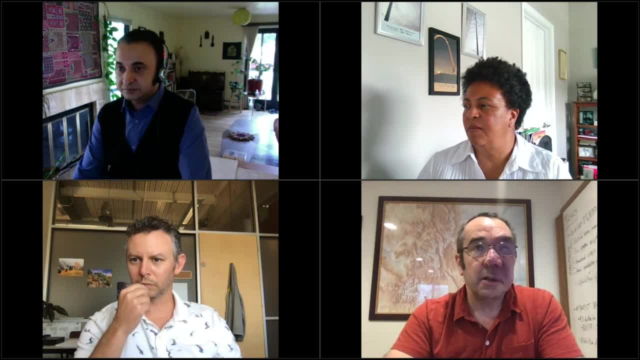 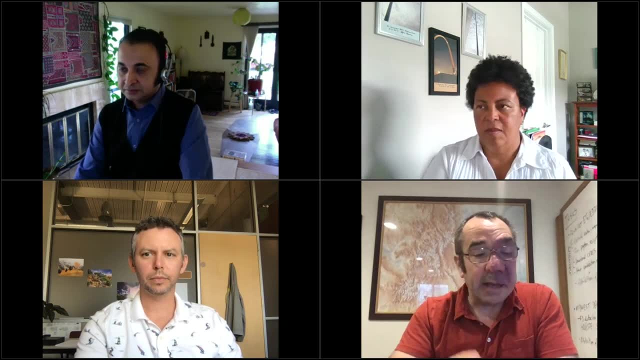 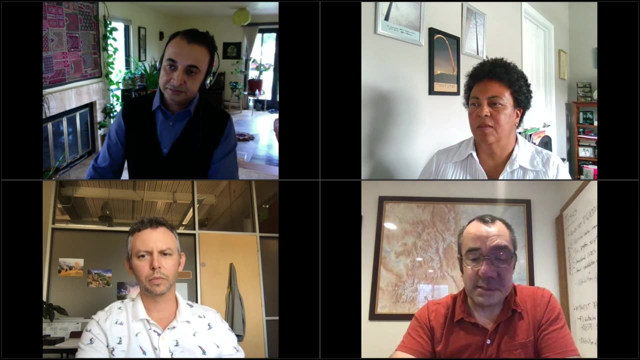 Eddy has a signal during the snow accumulation period in the Sierras. Longer term Eddy- like six month Eddy, for example- has a strong signal that is then linked to the melt off. so the snow melt in these snow melt driven basins And that's a very interesting finding because it indicates 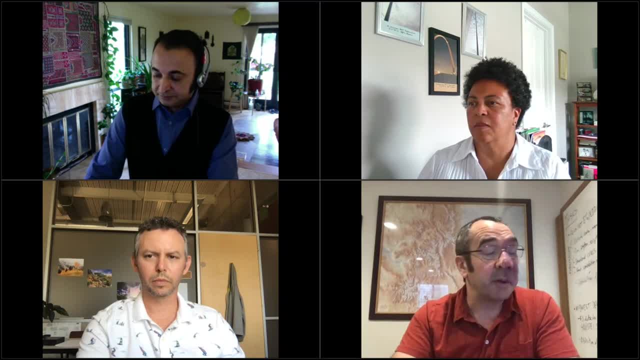 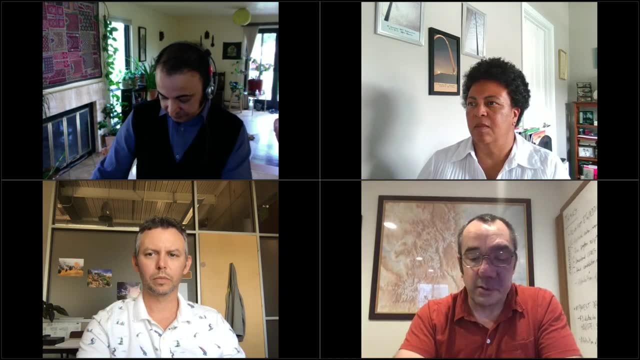 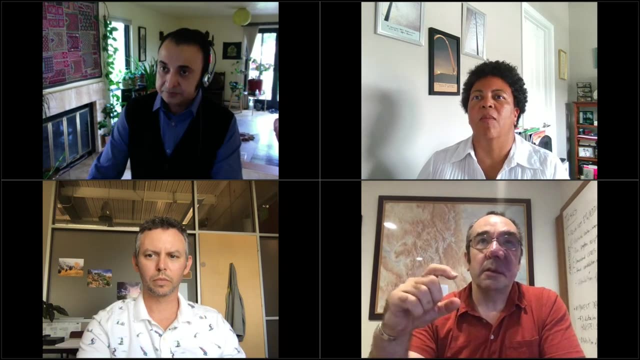 that snow accumulation is reflected in Eddy in exactly the same way that precipitation is reflected in Eddy, So you get a snow covered surface. it cools. obviously. it's cooler than non-snow covered, generally, at least in summer, And the anomaly of evaporative demand over that. 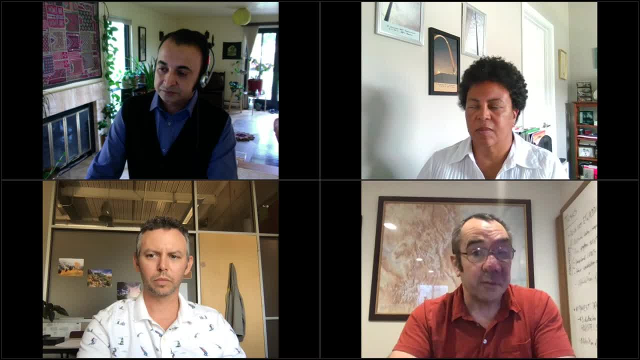 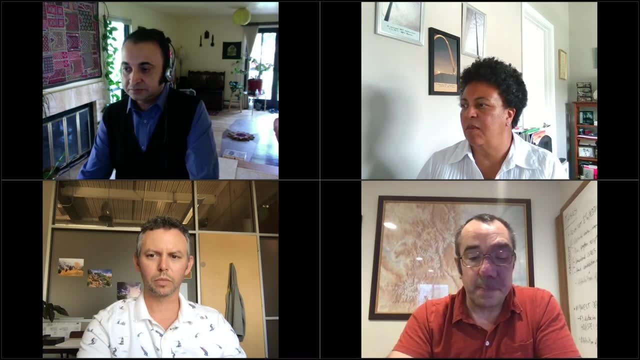 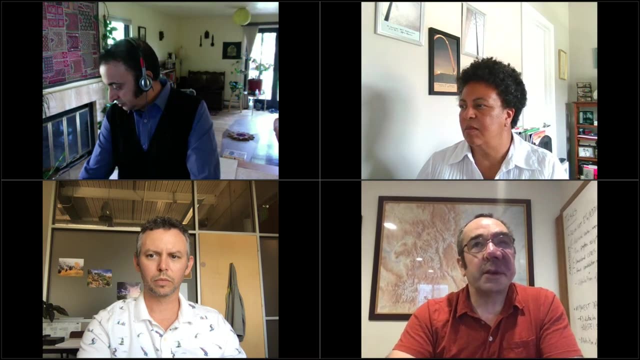 snow covered surface is just as valid as the anomaly over a soil moisture driven surface, for example, So there are indications that it is. it operates well in snow covered or cooler regions, As Vicky pointed out, though in energy limited regions where the hydroclimate is dominated by precipitation rather than evapotranspiration. 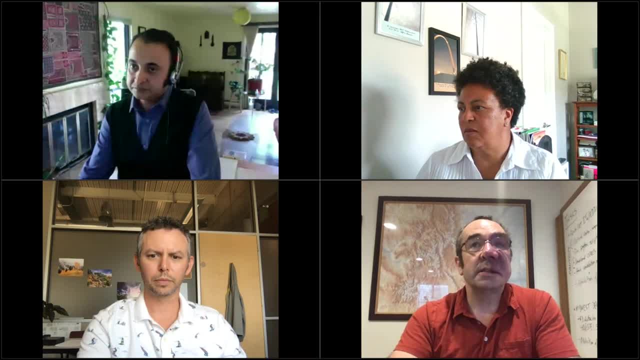 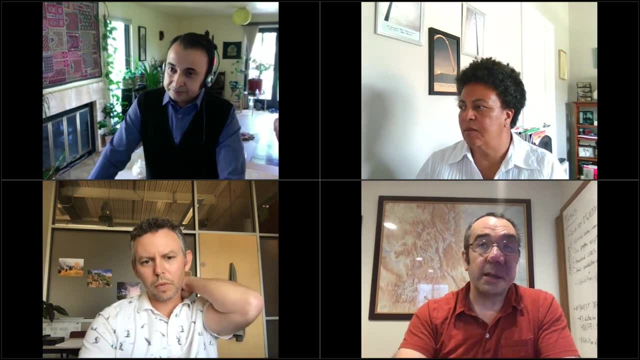 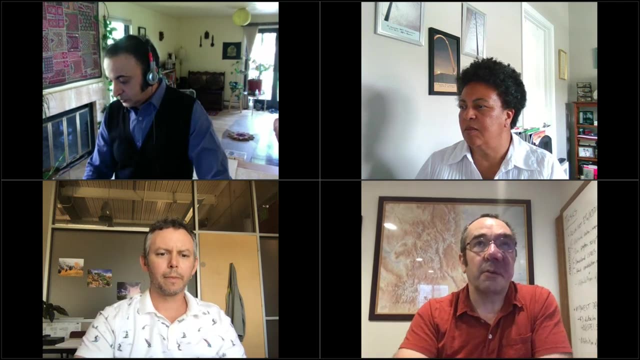 like in the west, you would want to supplement Eddy with other indices that reflect precipitation, And I would say a combination of Eddy and SPI would be good, because it reflects both the downward flux and upward flux of the hydrological cycle. that then indicate can indicate drought. 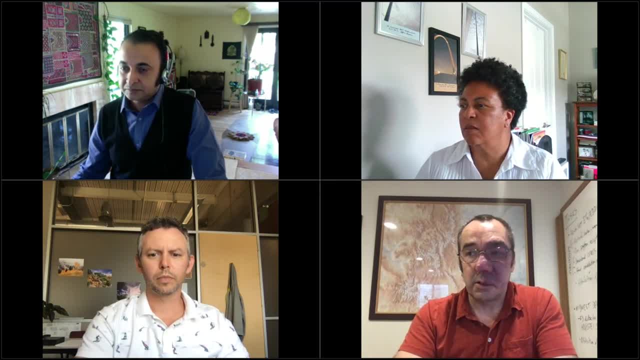 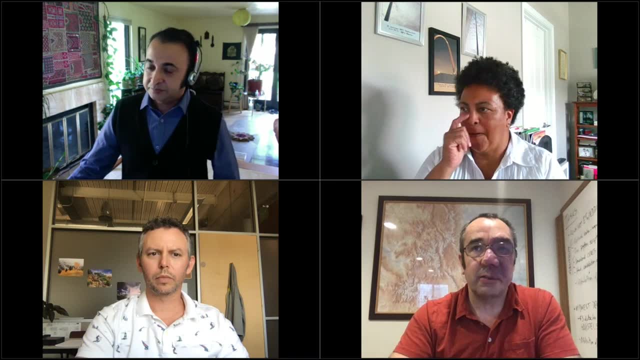 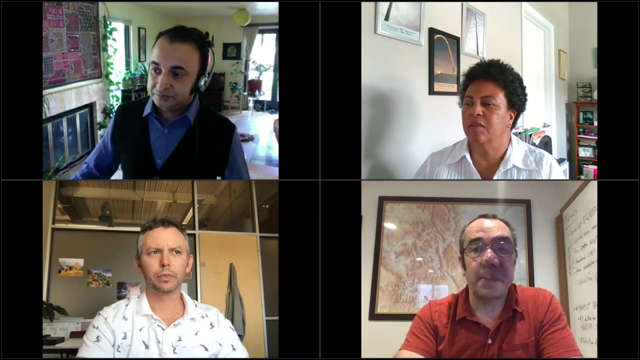 So it does. it does work in cooler climates. it's available globally. but you'd have to ask, you'd have to just email me and I can point you to that data source. And it does. there is a signal in accumulation and snow melt seasons as well that it's useful. that's a very brief nutshell answer. 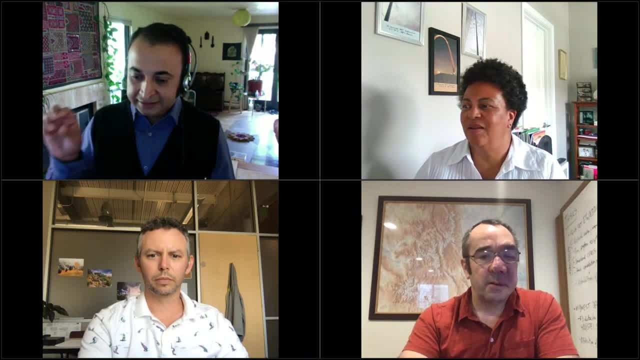 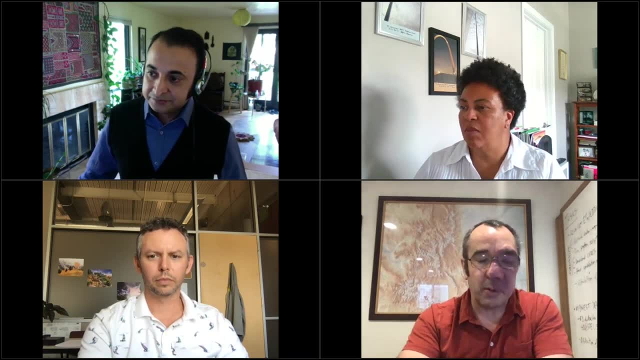 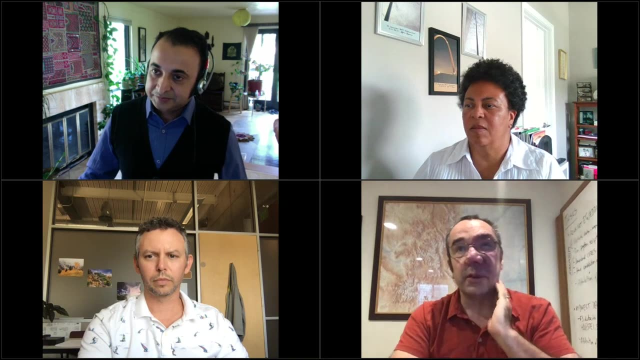 sorry, Trevor, and I can quickly add, if I may, and that during the shoulder season it may have value for wildfire warning. yes, absolutely, oh, I never. I didn't even talk about wildfire, perhaps because wildfire isn't a giant problem in the northeast but in the west. eddy has been used as a or is. 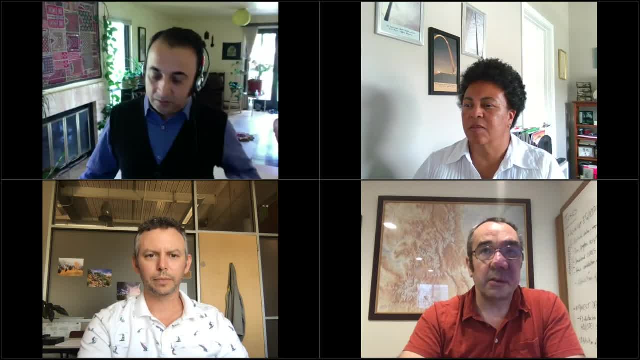 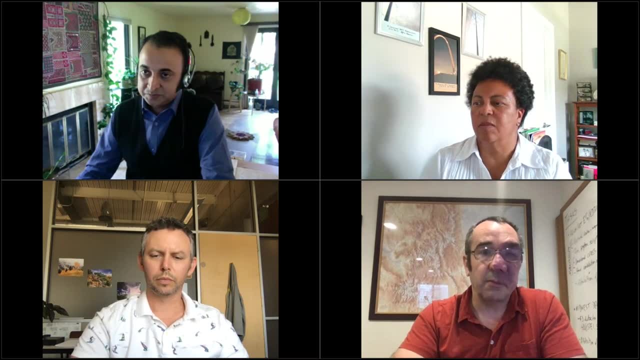 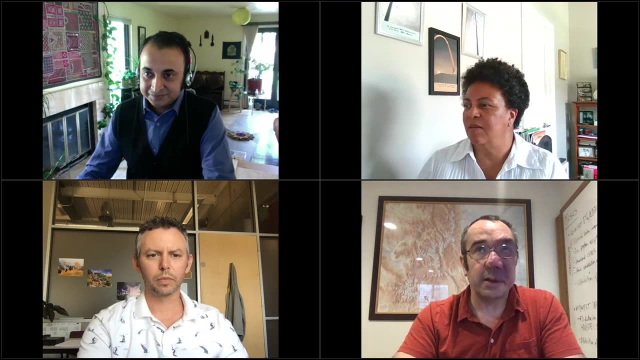 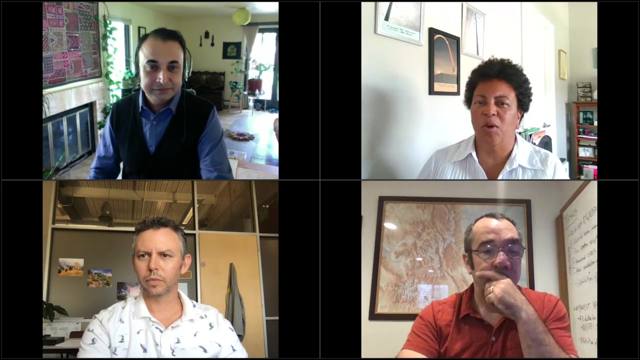 being used in various iterations in in wildfire, seasonal planning and in sort of ongoing meteorological incidents with regards to wildfire, and Dan has done- actually done- some work on on wildfire in California and Nevada. let's go back. I think I missed this one question from Glenn Kohler. 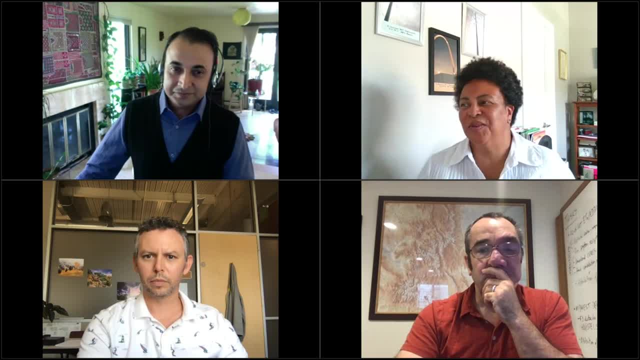 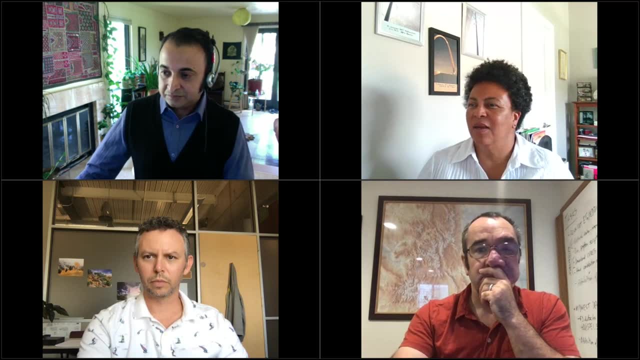 Glenn says it's great to see eddy projections coming soon. how soon weather forecast based or only driven by climate models? is Glenn still with us? I can actually let you wrap that. if you want to unmute yourself, go ahead, Glenn. well, it's just if you're good. I'm really thrilled. 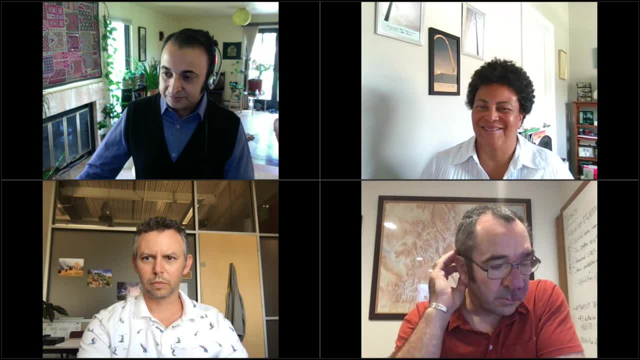 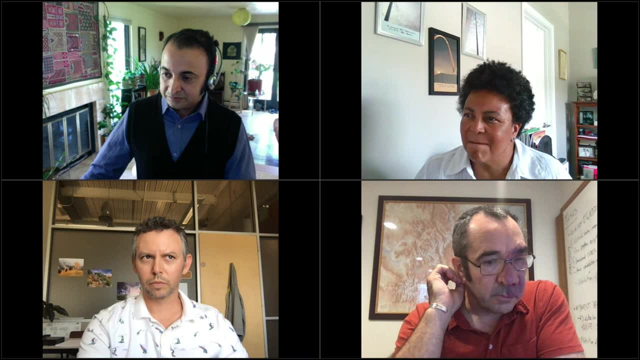 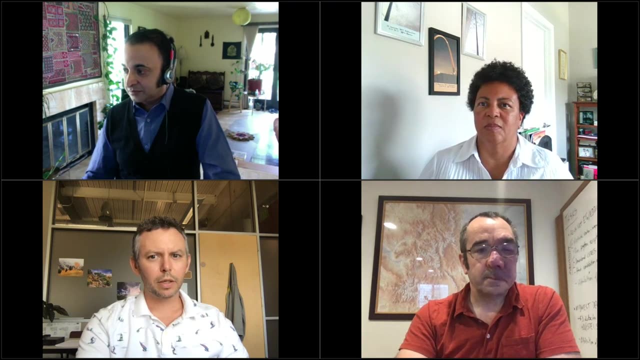 to see eddy forecasting. that's. that's very useful, but is it going to be driven by the near-term weather forecast or is it just going to reflect climate model protections over the longer scale and more? you know, more of a static thing? yeah, so the I did share a link to an 8 to 14 day eddy. 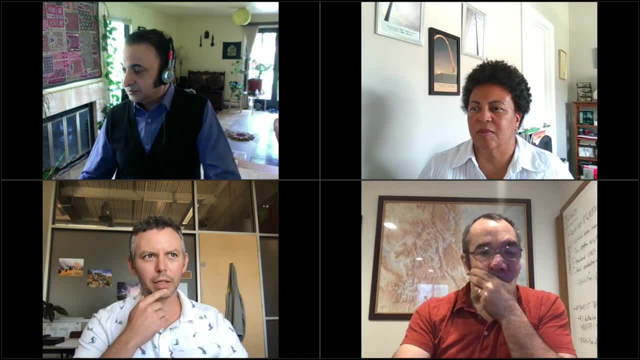 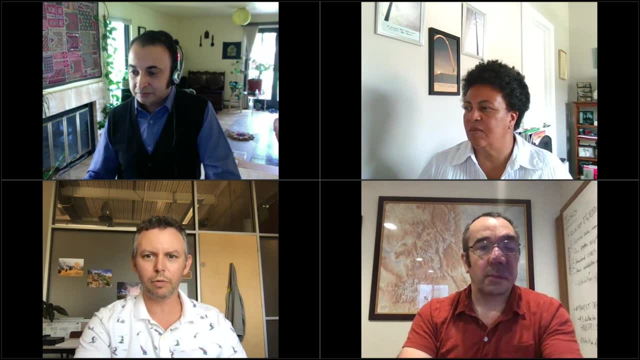 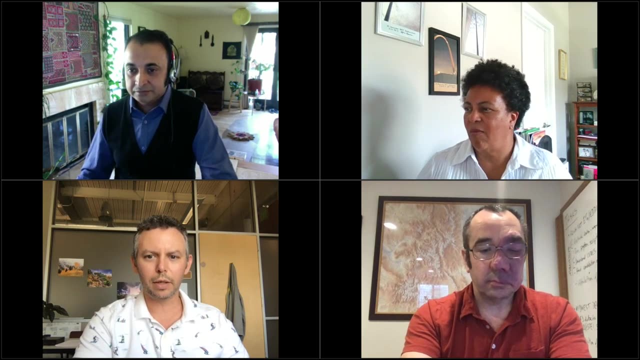 forecast, and so what we have in climate engine right now is based on the climate forecast system- sub-seasonal forecast- so that's essentially a weather model being run out to a sub-seasonal scales, and so it's a global forecast model that has the, the drivers that we need to. 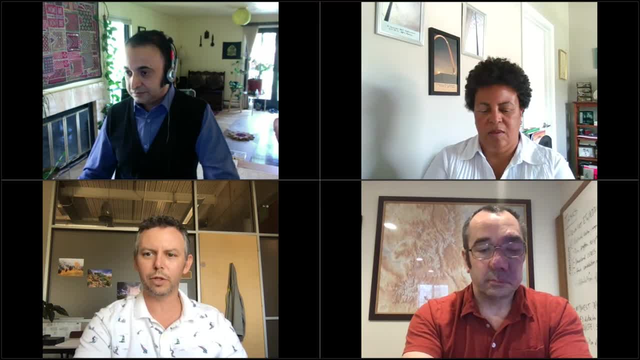 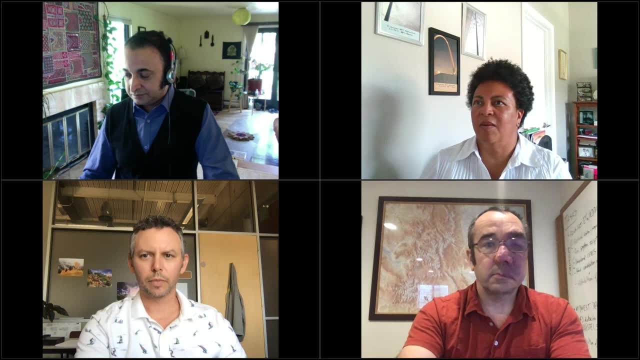 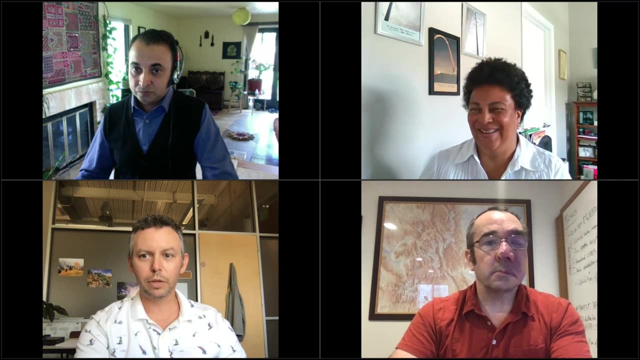 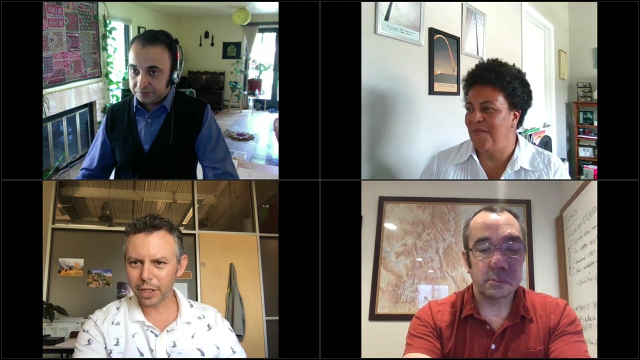 compute the reference et and then eddy from from those drivers. thank you, all right, how soon um those? those are available now um out to four weeks, oh, awesome, okay, thank you, and it's in the chat. and um I did post one link where you can find one of those maps. 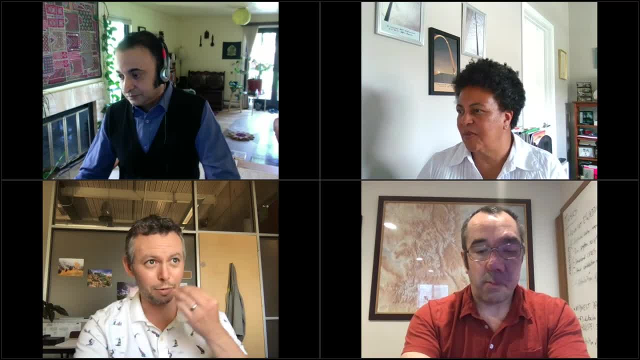 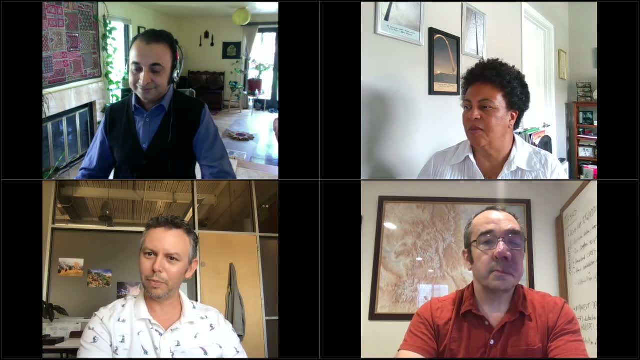 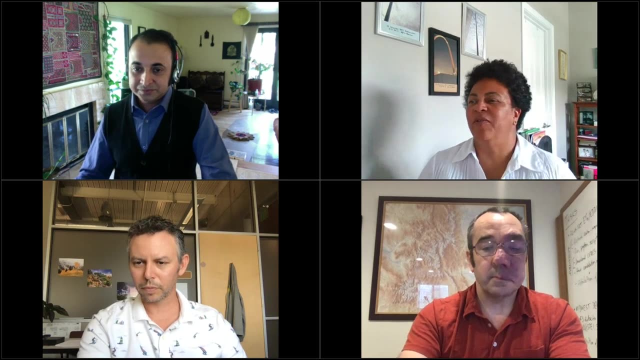 and I should also just mention, I think, um, if you are not registered, so if you click on one of those climate engine links, you're probably going to be forced to to register first. so be prepared for that. okay, and I have another question. I think we can get to from Trevor again and this does answer. 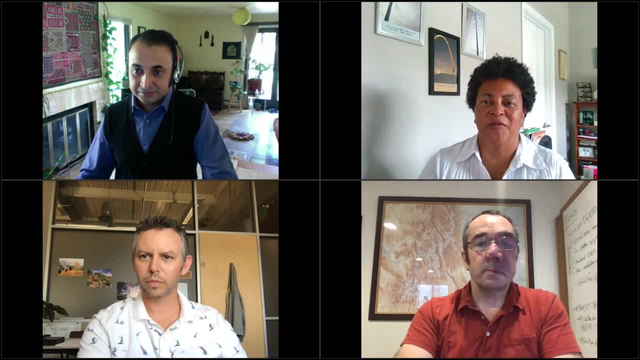 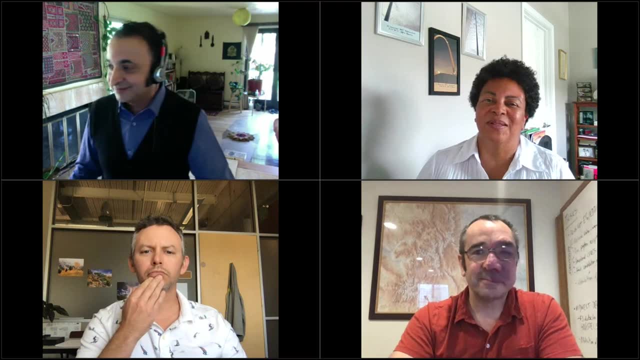 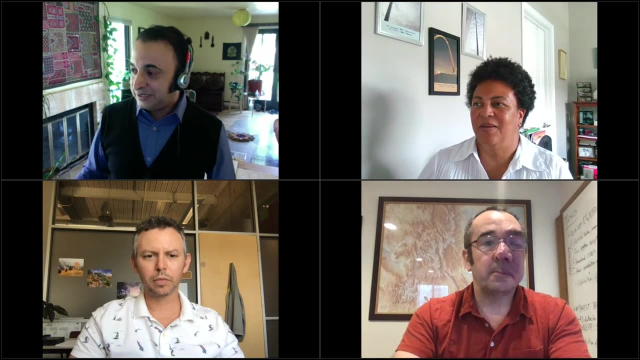 your question about, and your question, Mike, about whether Trevor is from Canada. He asks: is Larry available in Canada? If not, what would it take to expand this tool northward? Not currently, It's just maybe slightly north of the CONUS region. 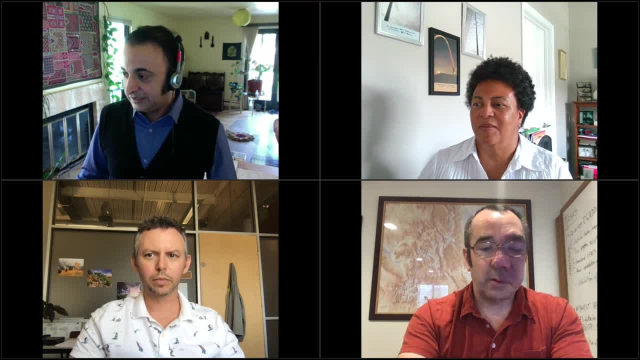 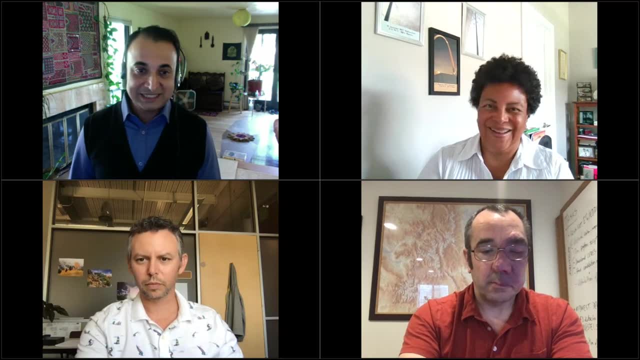 Some parts of Canada are there, But for now it's not there. I think it just would require more funding and partnership to extend it. I mean, the data is there. MODIS is global data, So you can really take it anywhere. 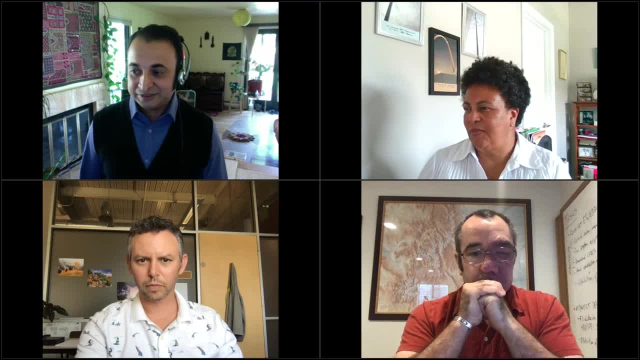 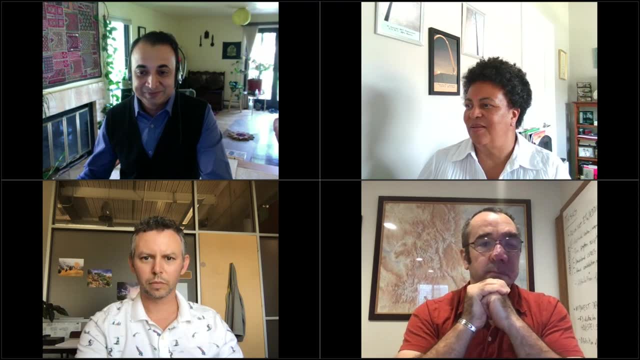 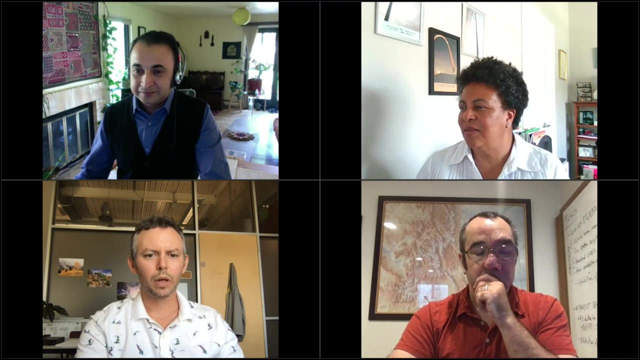 So it's just about the deliberation to get it there Right now. we need people and resources to do that, But thank you for your interest. OK, Let's get one from Keith Robinson. Keith asks: can any of the tools described? 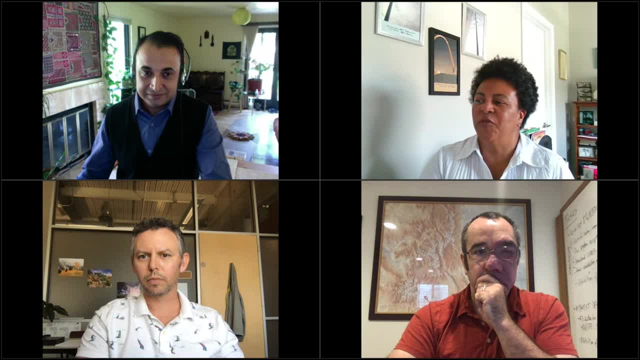 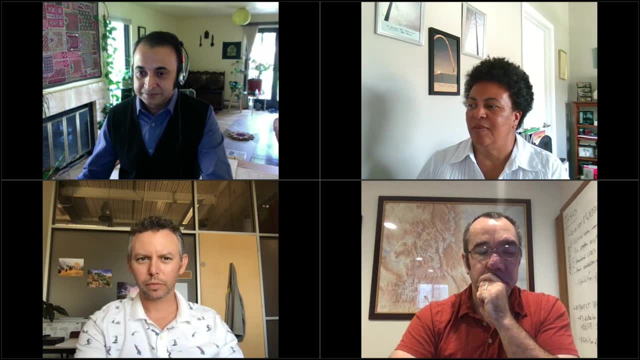 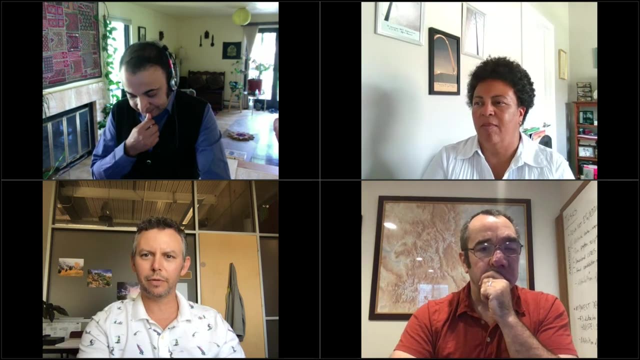 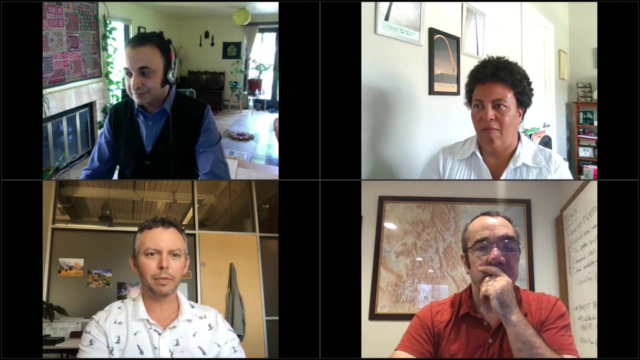 be used to help identify where more monitoring is needed to improve regional assessment. So I don't know if the tools themselves could do that, But that's where we like to hear from folks. We did show a lot today. Is there something missing that is needed for the Northeast? 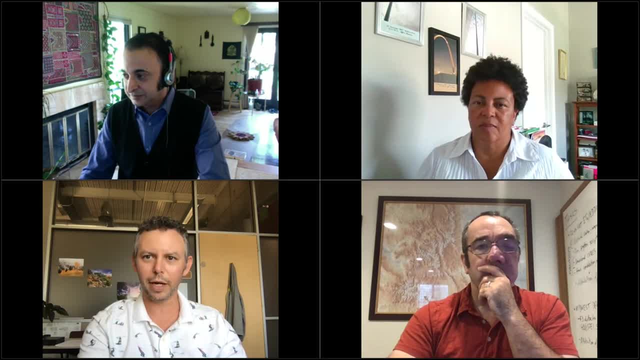 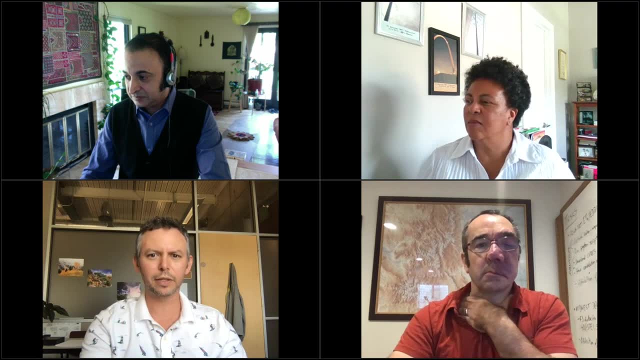 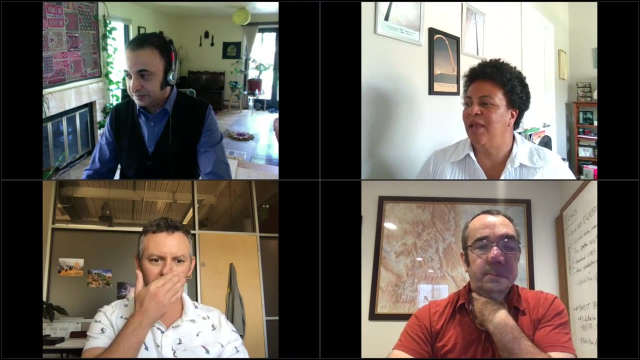 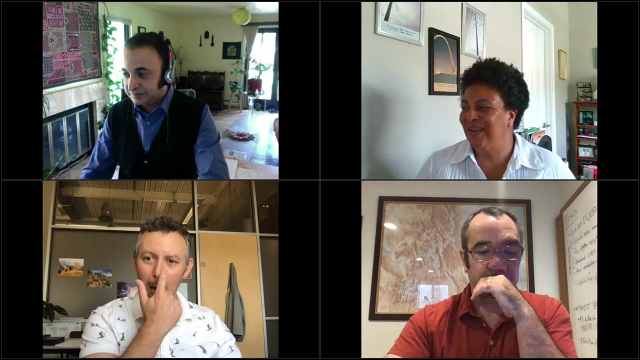 that is not in these tools or anything that you've seen, And so I'm not sure the tools themselves can help answer. But I'll try to answer those questions And Jeffrey Zimmerman ads API would work. I don't know if that's a statement or a question. 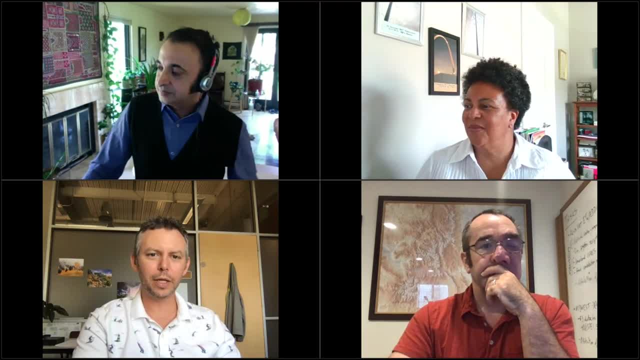 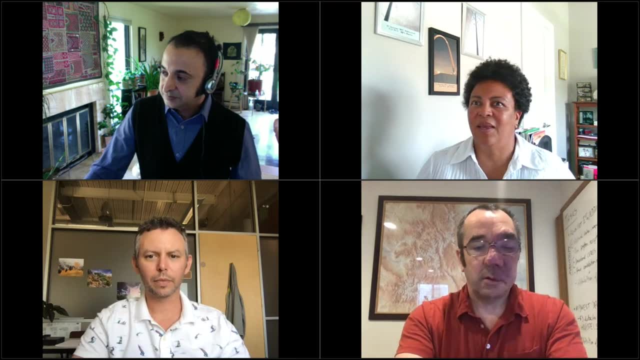 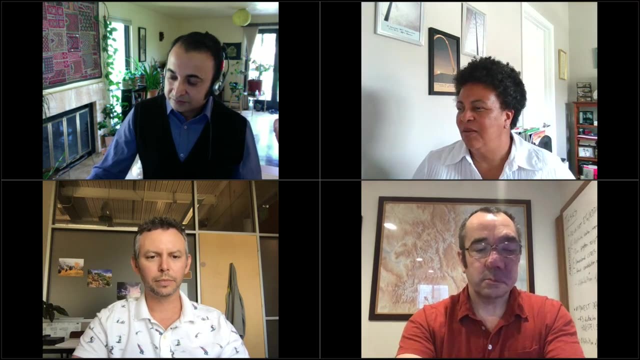 API would work. Yeah, And if you want to contact me about that, if you're interested, we can set you up with an API token to start using that for climate engineering. OK, going to probably wrap it up with this one. it's from stephen harkey. stephen says um on the drip. 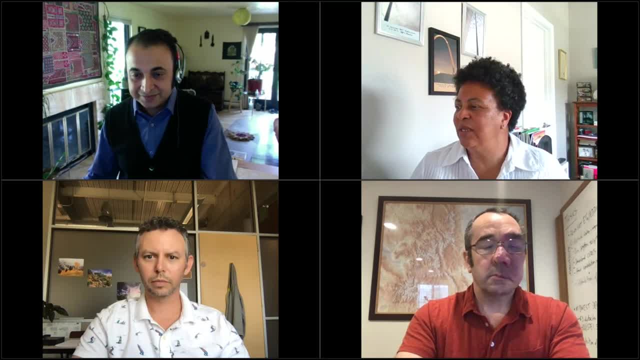 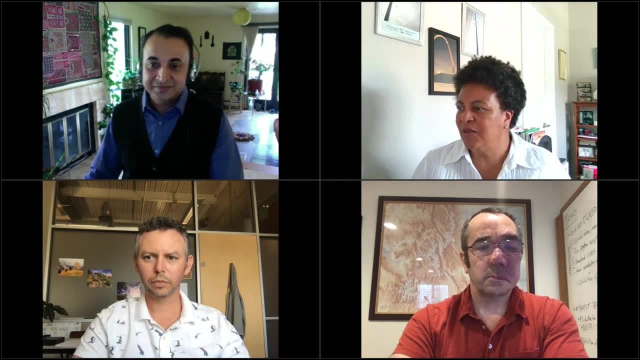 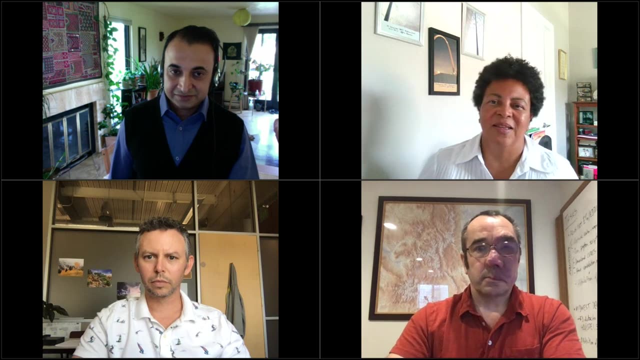 many of the northeast states are small and when zooming in to see details they become, uh, just small dots and they lose their detail. can this be made better? also, can you download the charts at the bottom of the page? oh, i guess that's for me, uh, at the page versus the screenshot. 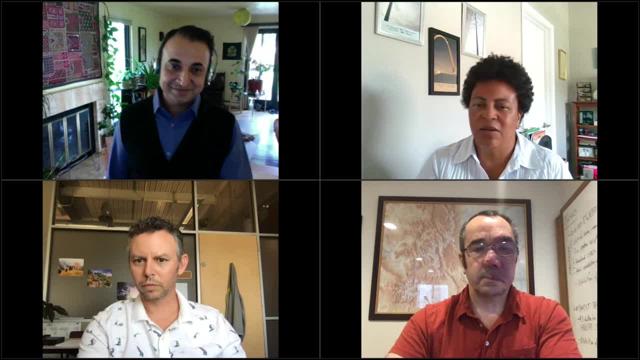 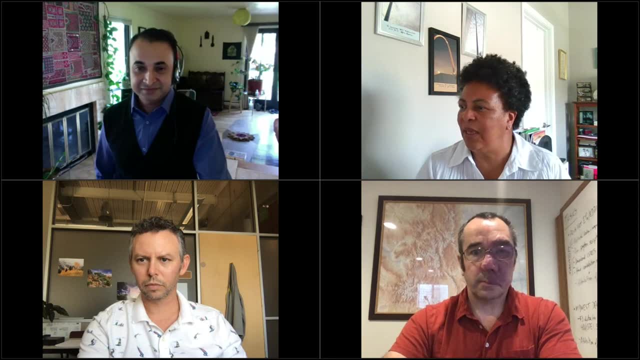 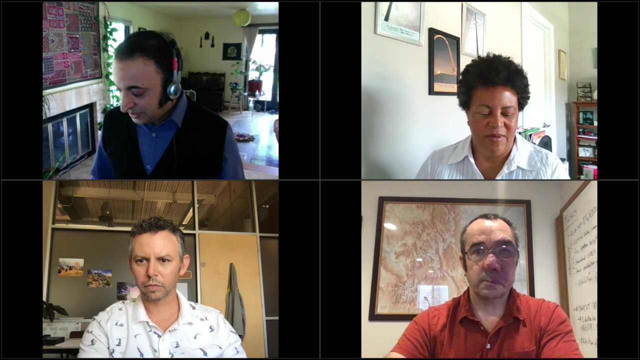 so what i would say about, uh, the download is that we're going to have the entire recording available and if that doesn't quite meet your needs, uh, please email me. but uh, let's go ahead and let impias comment on drip. yeah, thank you for your question and thanks for looking it up quickly. 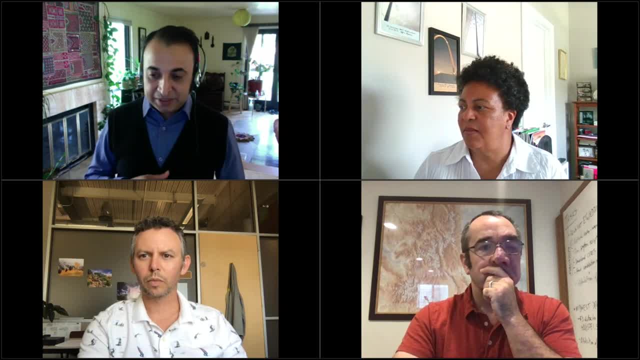 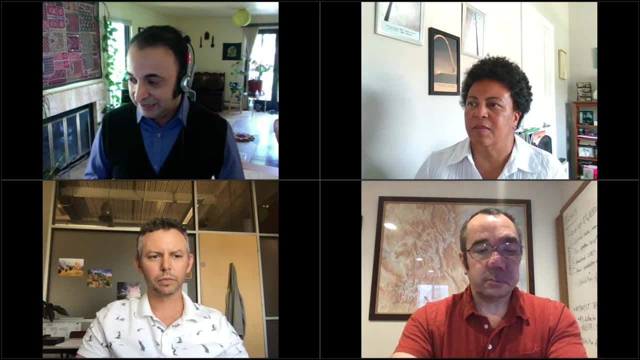 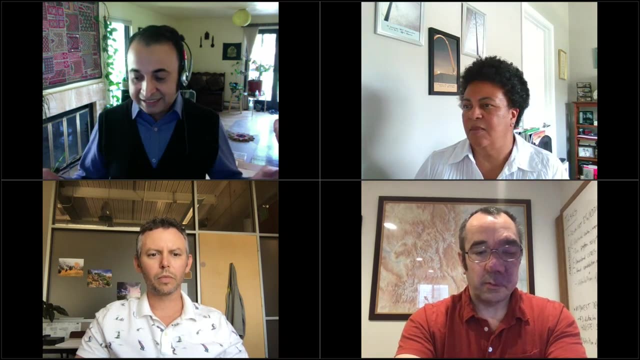 uh, that is the one of the issue with the spatial plus. i did mention my, uh, my presentation, that, uh, you know, climate engine would give you much cooler maps. if you're interested in the maps, uh, we will actually look into that uh at some point. but our main interest was really looking, getting the time series data and and visualizing the 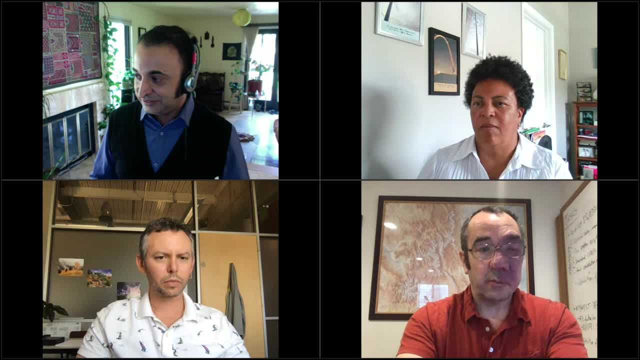 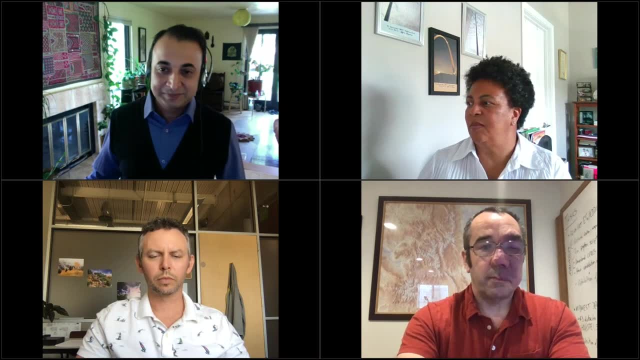 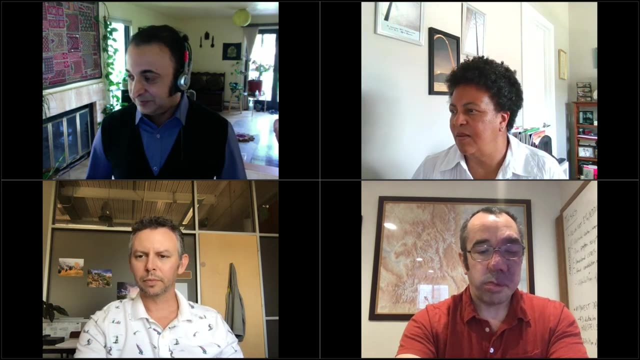 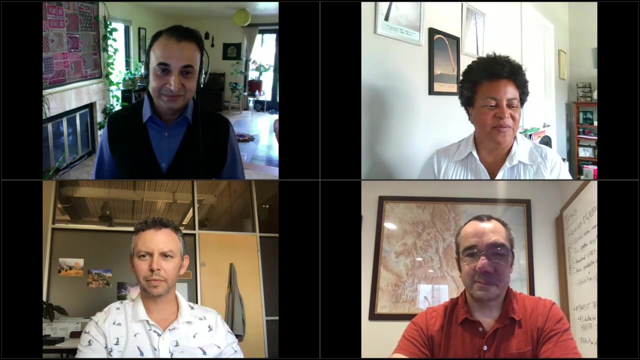 time series, and that's why we put more effort there than kind of improving the maps, because other there are other utilities uh out there which can do a better job mapping these things. okay, thank you, my goodness, i think we just made it through in the nick of time all of the questions that we have. my apologies if we 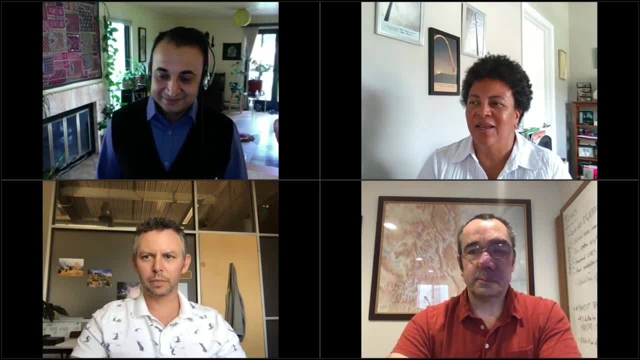 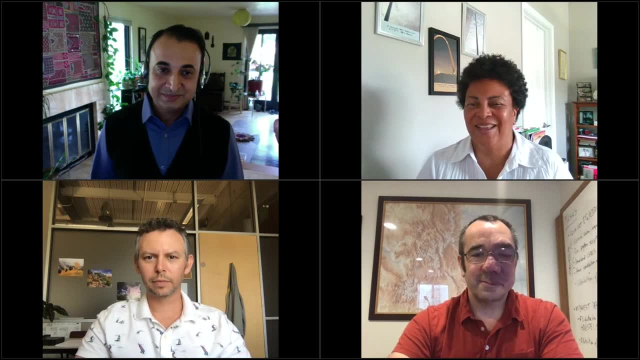 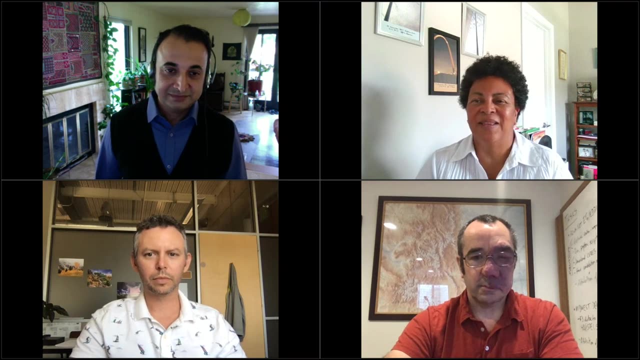 missed anybody, but i do think this was a great discussion. i hope, uh, the folks here in the northeast now feel like we're not being left out of drought research and that there's active work going on so we really can get to that early warning capability. thanks again, so much to dan. 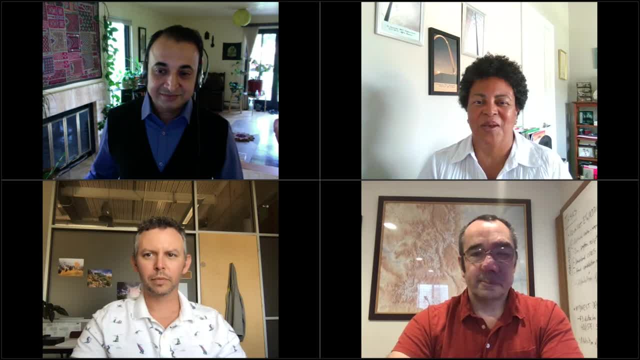 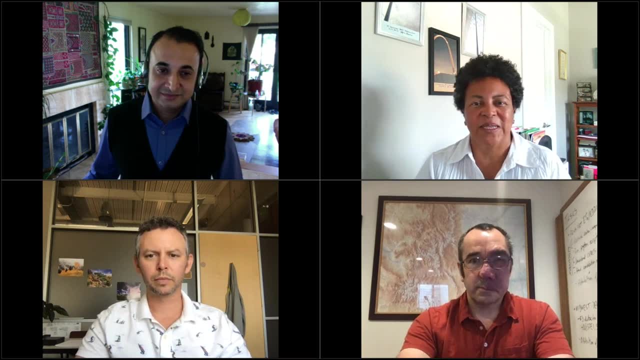 and his team, uh, impias and mike, for your presentations as well. please look for this recording on droughtgov shortly and also the recording from the first session last, from last week, and we'll also be sending out- you'll watch your email for our constant contact email. that kind of highlights uh what went on. quick little summary and then a link. 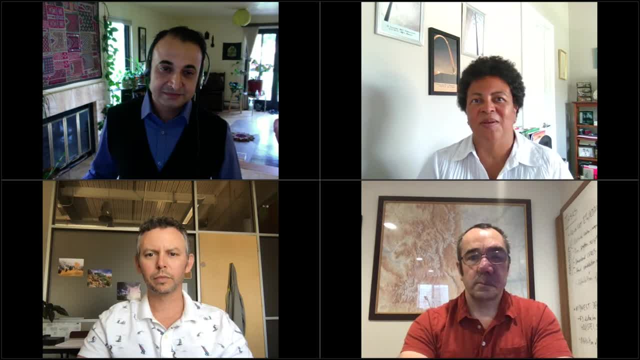 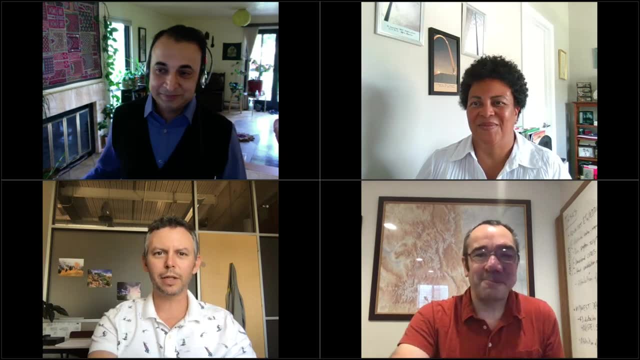 to the recordings that we've had for the last two sessions. so thanks everybody. uh, have a great day. thank you, thank you, bye-bye you.